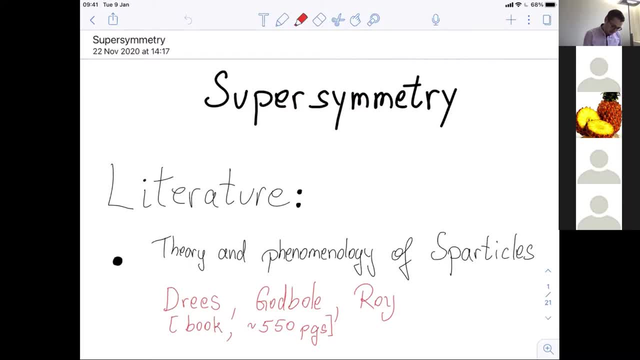 for example the space-time symmetry and internal symmetries, where the internal symmetries can be either global or local. Local gauged it means gauged. For instance, in the standard model we have the point carré symmetry, which is the full space-time symmetry, And 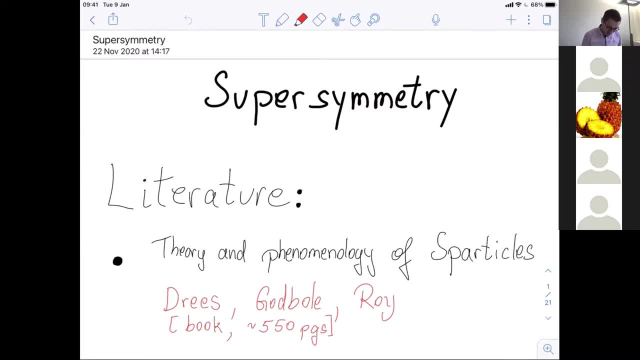 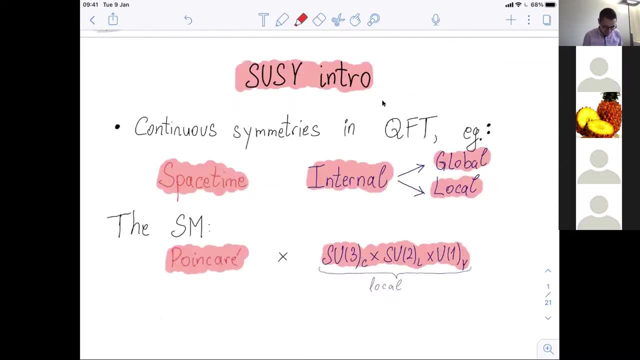 then we have the gauge symmetry, which is the internal local symmetry, which is the product of SU3 color, SU2 left and U1 hypercharge. I gave you examples of continuous symmetries in the standard model, which is the point carré symmetry and the gauge symmetry, And 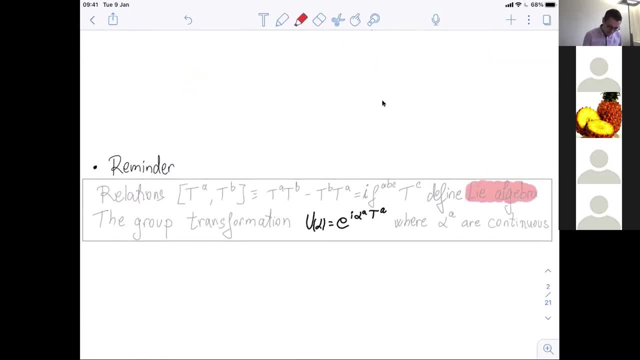 now I talk about the Lie algebra. The defining relation between Lie algebra is this commutator relation, So the two elements of the algebra which I call here TA and TB. there is a relation, Lie bracket, which is the commutator. This is a linear combination of the elements inside the algebra F A. 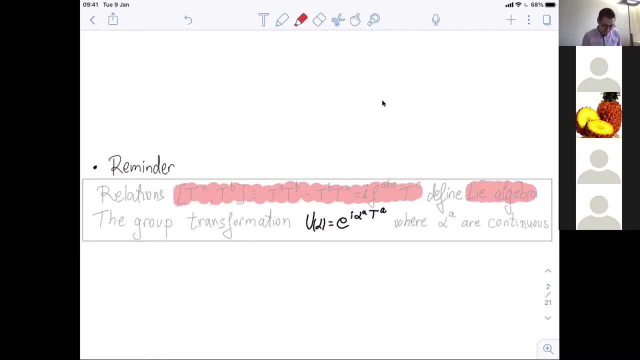 B, C are the structural constants which define the algebra, And these elements are called the generators of the symmetry. Why? Because when you exponentiate the generators in this way, where alpha A are some continuous parameters, hence a continuous symmetry. So 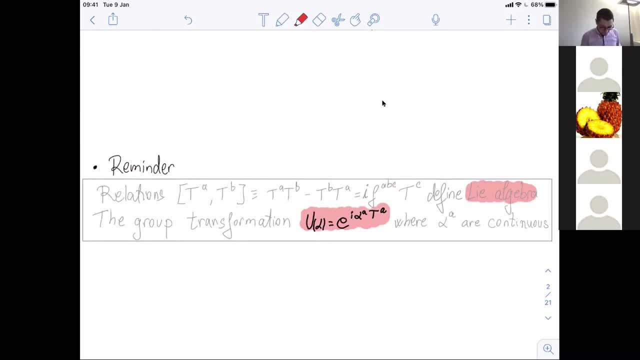 alpha A are real numbers. We get the group transformation. A symmetry is invariant under these transformations. So when you do this transformation you get the thing stays the same. That is the group transformation. The thing stays the same. That is the group transformation. 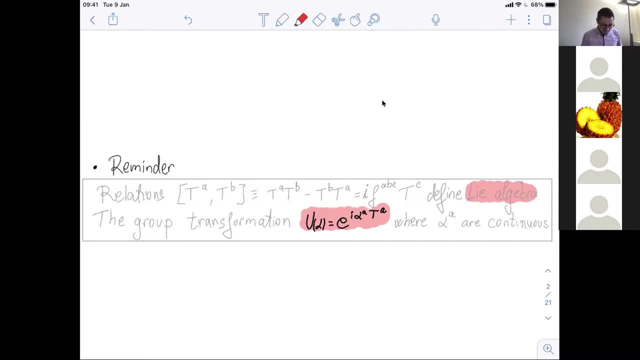 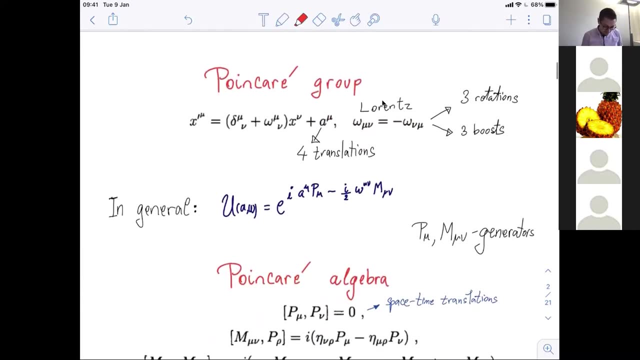 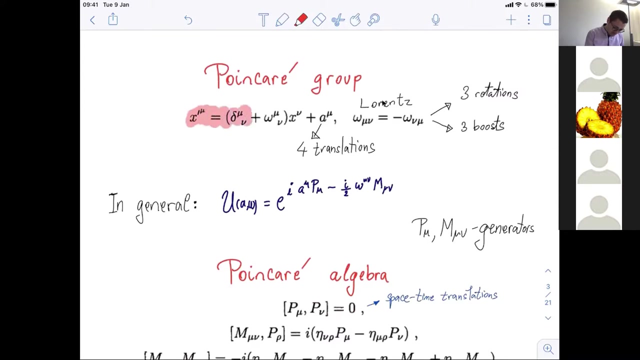 That is the symmetry. All right, So the key concept here are these algebras. So let's go back to the point carré group and point carré algebra. So the point carré group is the group which transforms the space time in this way, So the inhomogeneous part. 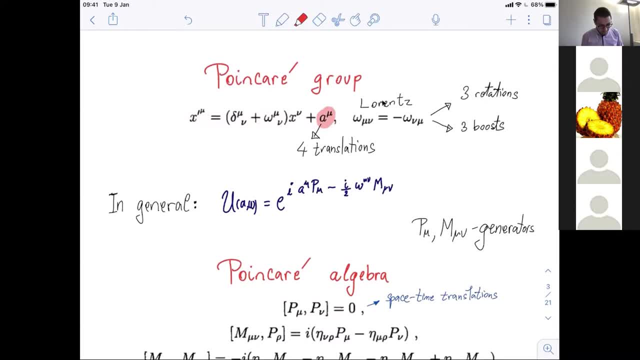 corresponds to the translations. In fact there are four generators of translations. And then there is this part which corresponds to the Lorentz group. These are four-dimensional matrices and they are anti-symmetric matrix, So it has six degrees of freedom, In particular. 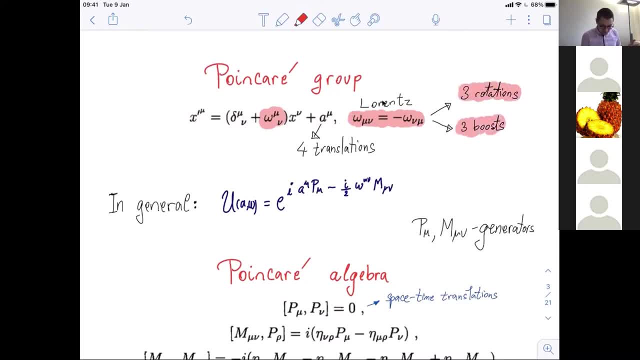 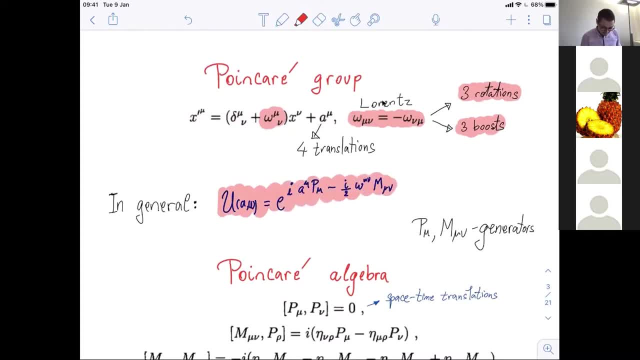 is given by this formula, where a? mu and omega mu nu are the parameters which define the, the group element. okay, continuous parameters which define the group element, and p? mu and m? u nu are the generators of the, of the transformation elements, of the, of the of the algebra. so how does this algebra look like? 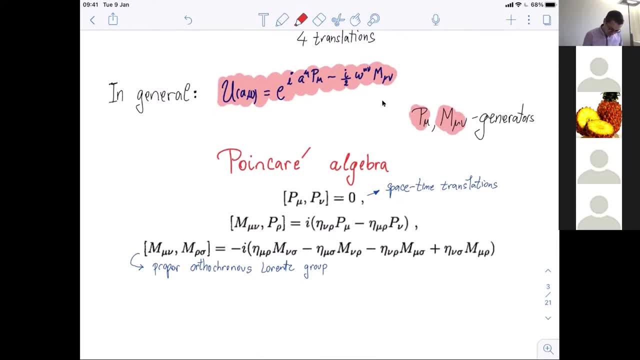 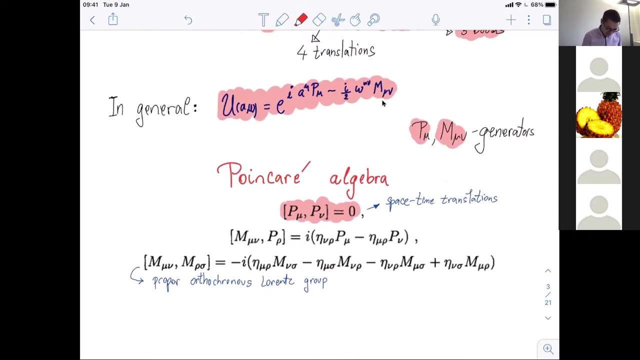 it's given here by these three equations: the first one is the commutator of, the, of, the of the translations. so these are space-time translations: and and it's zero the. the third one is the commutator of the Lorentz generators. notice that the commutator 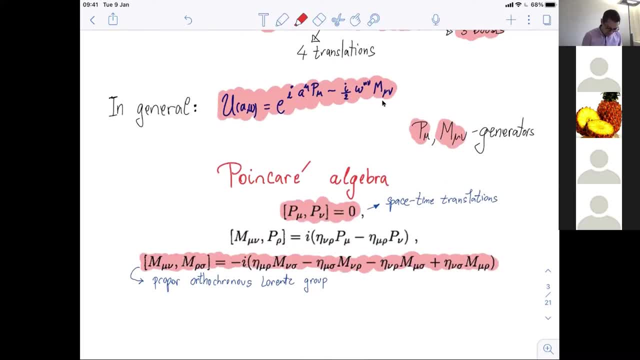 of the Lorentz generator is the linear combination of themselves, meaning that this is the Lorentz, this is sub-algebra of the full Poincaré algebra. this is the Lorentz algebra. In fact we are considering only so proper, orthochronous Lorentz group. so we are considering only 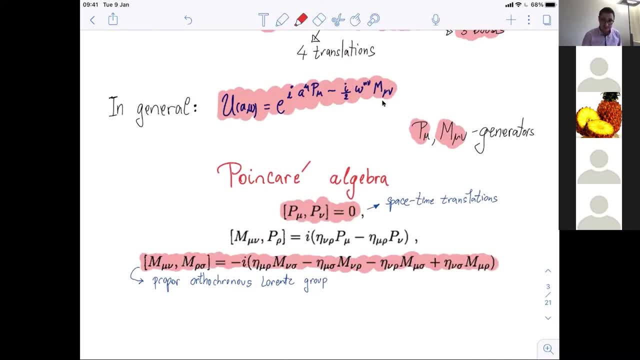 transformations which are continuously connected to the identity transformation. Also notice here that there is a, the second relation, which mixes translation and Lorentz generators Under commutation. it gives the linear combination of the of the translation generator, so it's a. 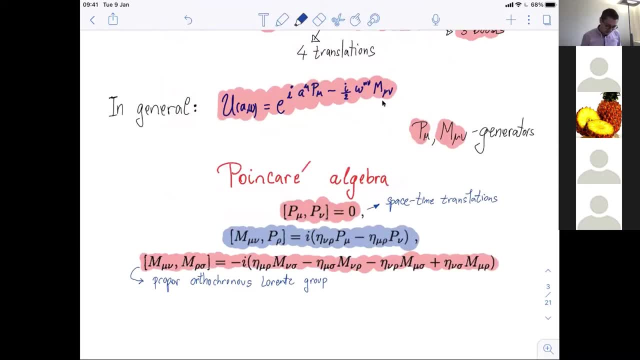 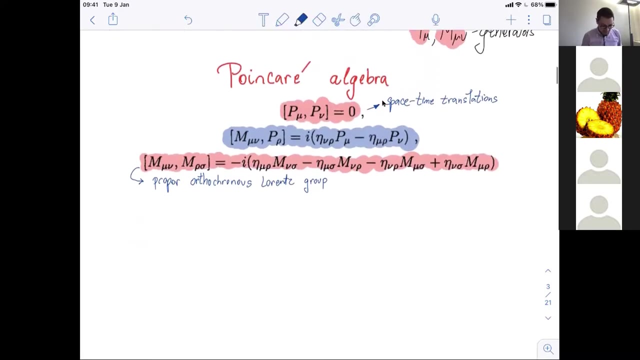 non-trivial relate, non-trivial way of combining translation and rotations and boosts. All right, so this is the second relation. This is the Poincaré algebra and it is really the basis of the way we understand the spacetime and it is the basis of the standard model. 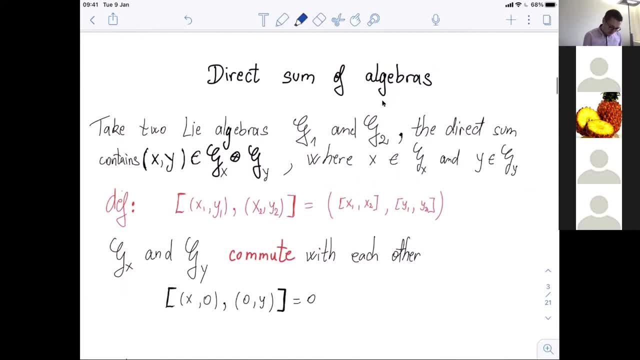 So one thing: when we talk about the full, continuous symmetry of the standard model, is this direct sum. So the direct sum of Lie algebras- G1 and G2, are defined in this way. So the direct sum, the elements of the direct sum, 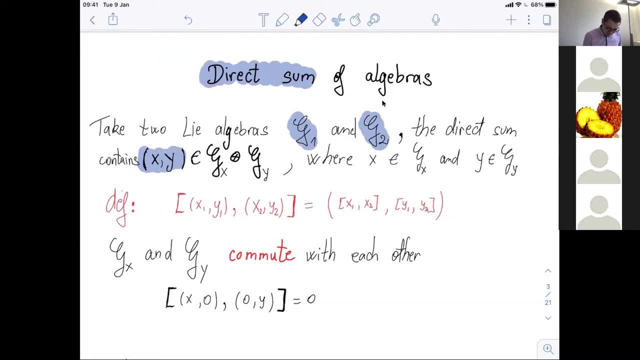 are ordered pair X and Y, where X belongs to GX and Y belongs to GY And the defining Lie bracket simply says that the first, the first term in the element, will be just the, the, the commutator under gx. okay, so you take x1, x2 under gx and you do the commutator, and 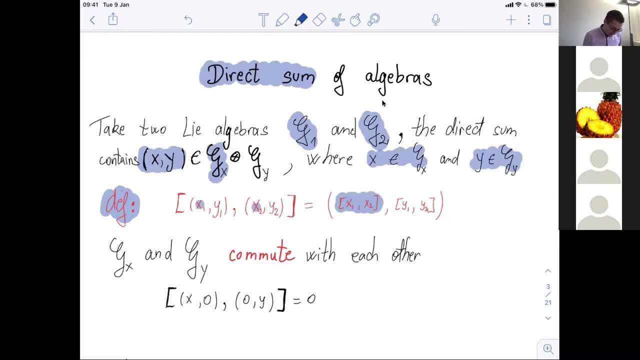 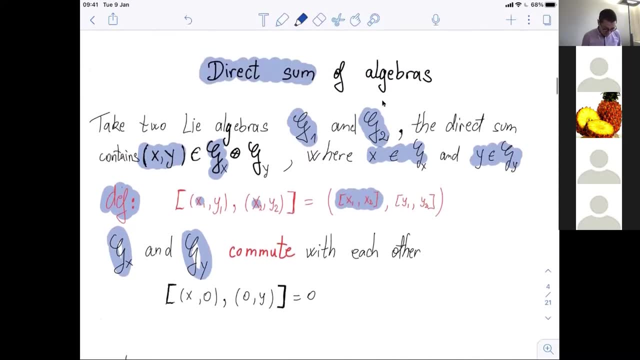 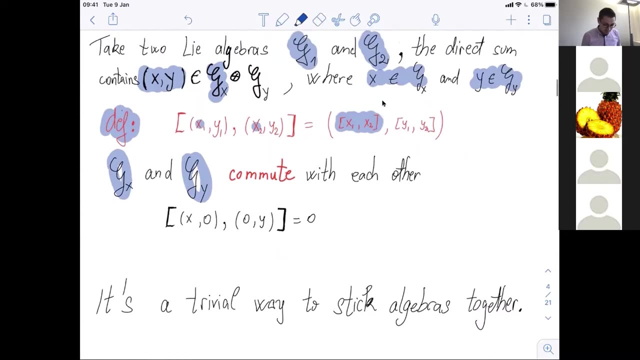 likewise for y. it's a very trivial way. so in particular, gx and gy commute with each other. this is the direct sum of algebras and it's a linear. it's a trivial way to stick algebras together. that is what we have in the standard model. so the full, uh, the algebra is the product. 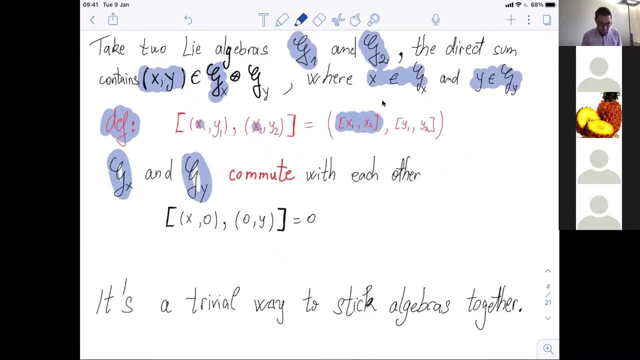 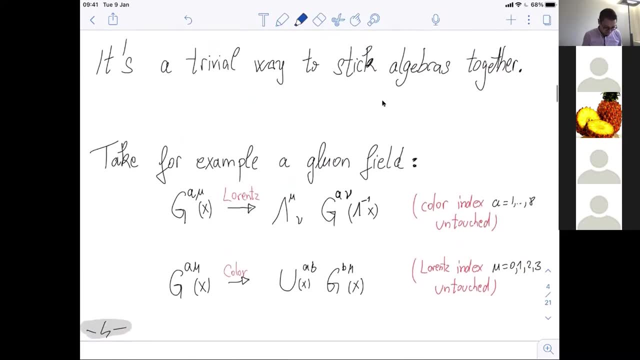 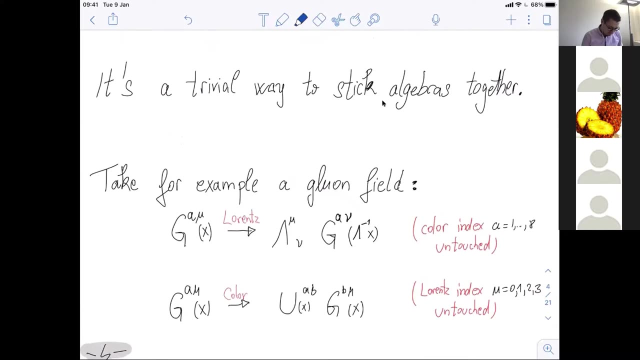 of the point career, one for the space time and then times the, the internal one for the gauge symmetries and maybe some other global symmetries. um, well, well, simple example. so let's um the illustration of this, uh, separation. for example, let's consider the gluon field. 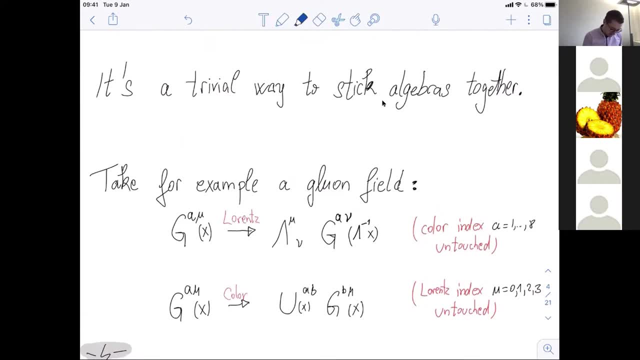 the gluon field. uh, so first of all it's a field, so it depends on the space time coordinate. then it has two, two indices: one is a, which is the color index. so the gluon is a joint representation of su3 color and the color index goes from one to eight. 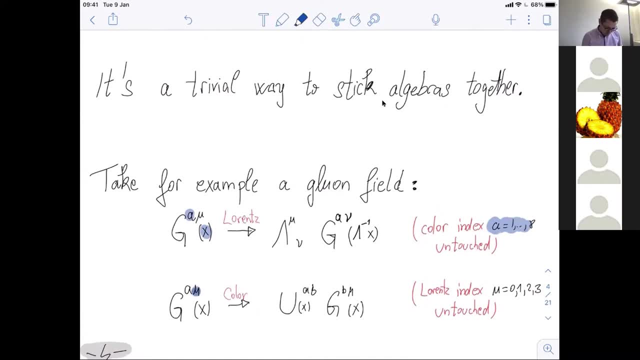 and the second one is mu, which is the space time index. gluon field is a is a four vector. it's the vector representation of the of the uh lorenz group. so under lorenz transformation shown here, the the color index is untouched. so you're just you know. 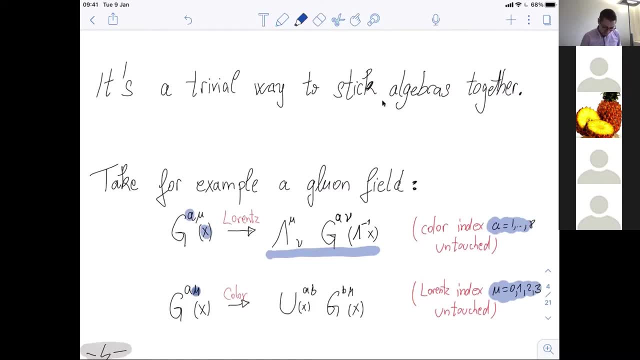 but you're just doing the transformation on this, on the, on the, on the lorenz indices. and likewise, when you perform a color, color rotation, which here depends on x, because it's a local, it's a local transformation, then you don't touch the, the lorenz index. okay, so it's a. it's a very trivial. 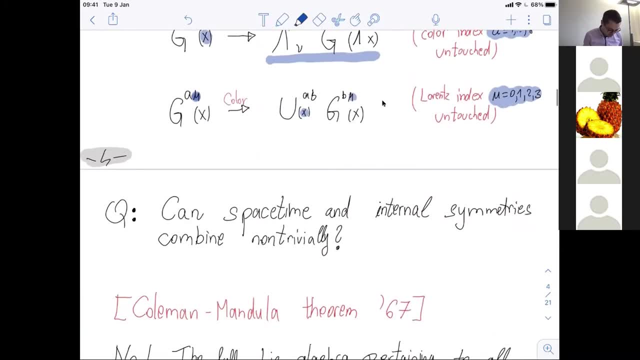 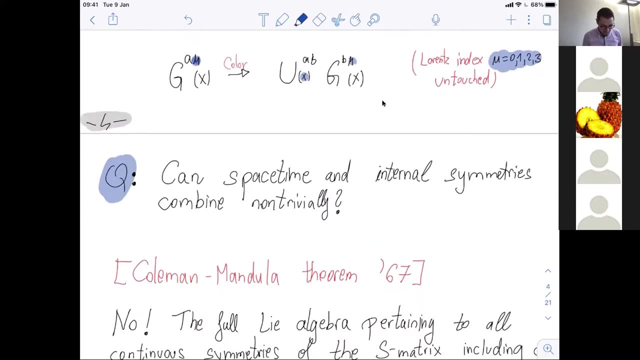 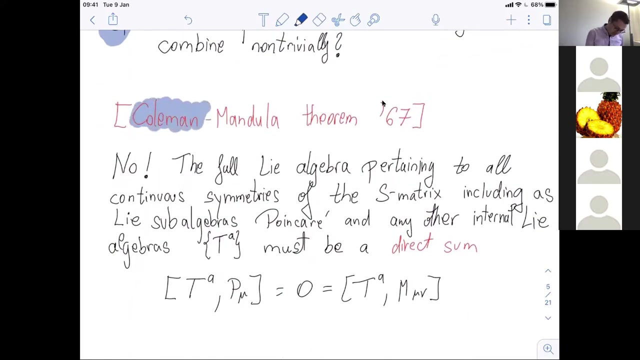 way to separate different uh symmetries. so the question which um we want to ask here is that is the following: can space, time and internal symmetries be combined in a non-trivial way? that's the question. so that there is this famous theorem which goes under the name of coleman mandula, theorem from 67. 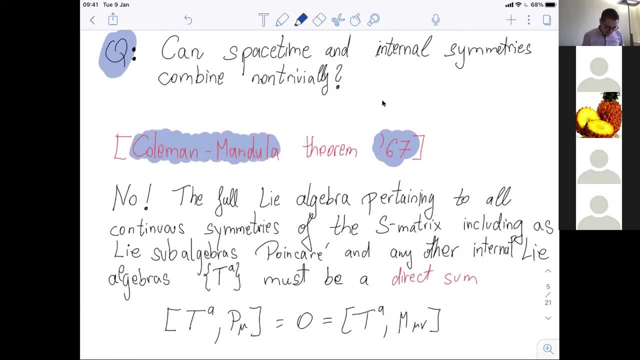 um, with the answer being no, the full lee algebra um pertaining to all continuous symmetries of the s matrix s matrix being the, the, the, the, the scattering made the the scattering matrix um of the theory. so the the full lee algebra of that describes, uh, all continuous symmetries, and including: 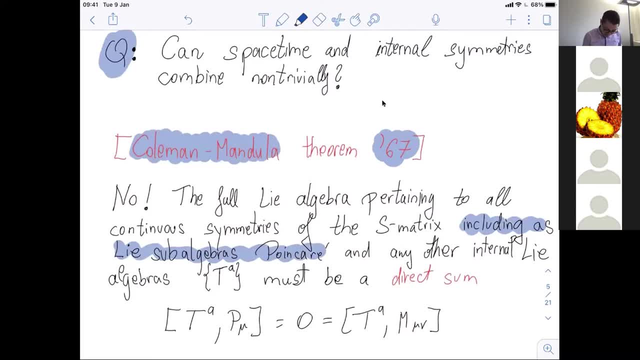 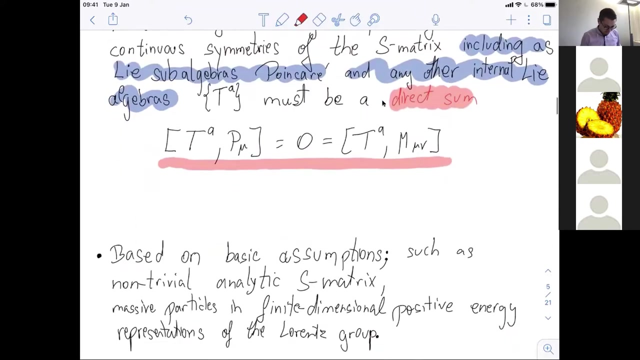 lea, subalgebra, point kare and any other internal symmetry must be a direct product. okay, in particular, this has to hold, as we saw, for example, in the standard model. okay, so let's look- uh, sorry, let's look- at rome. to go back to the old, 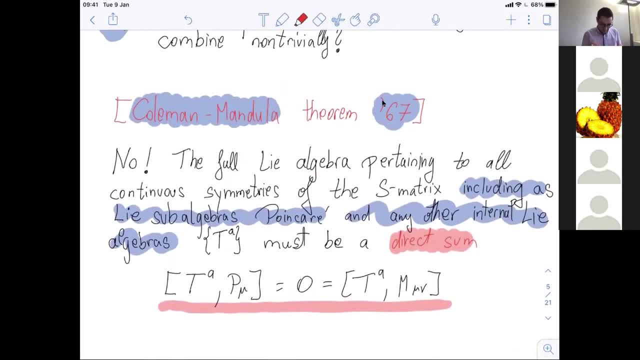 okay, so the the most general continued symmetry, um, which is lea algebra. okay, that is the caveat. if the continuous symmetry is lea algebra, then the most general one, um. if it includes a subalgebra, point, kare and any other, then it has to be a direct. 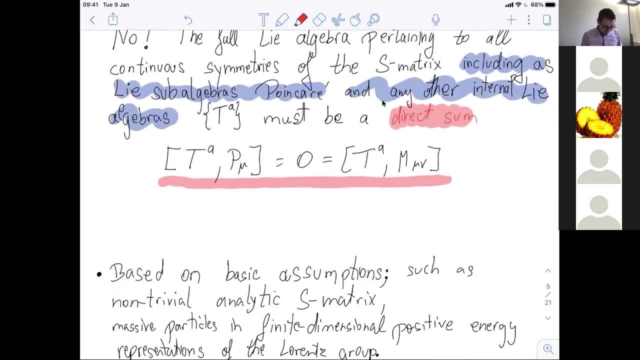 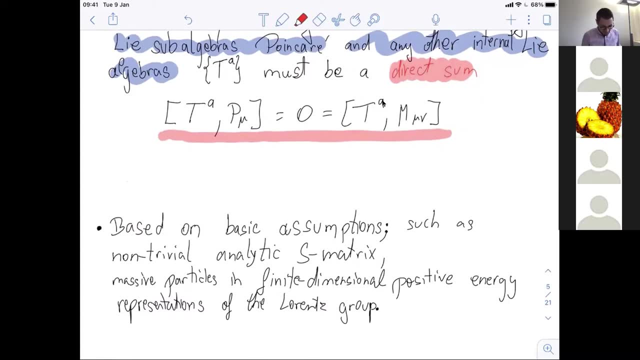 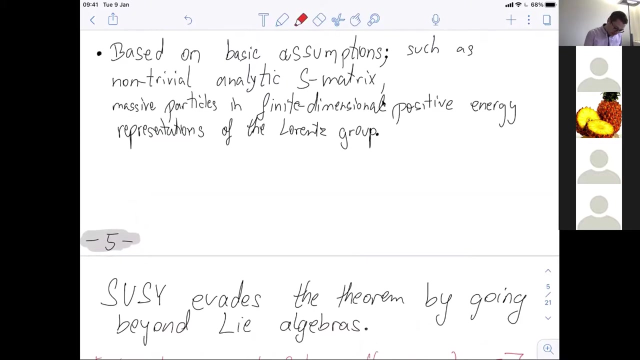 sum um. so this, uh, this is this- is based on some, um, reasonable assumptions to have like in interacting theory with the finite dimensional representations and so on. So it's a quite general result in quantum field theory. So supersymmetry actually evades the theorem. It evades this theorem. 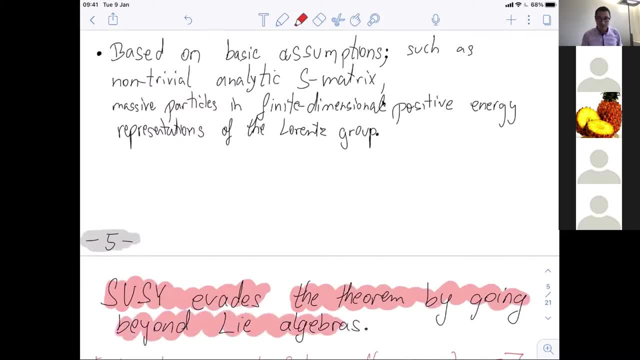 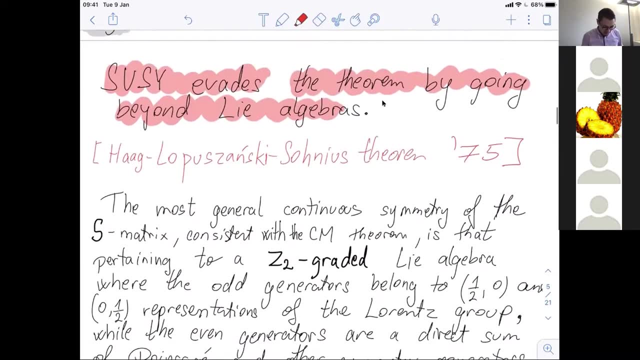 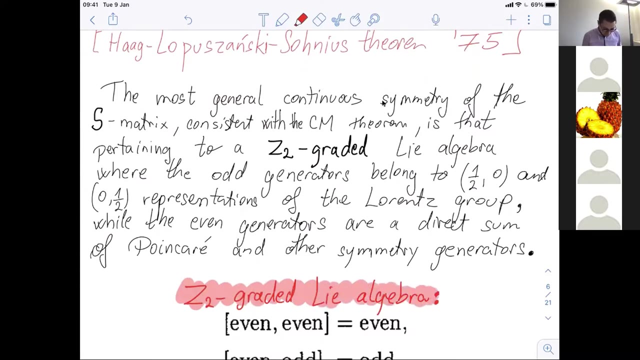 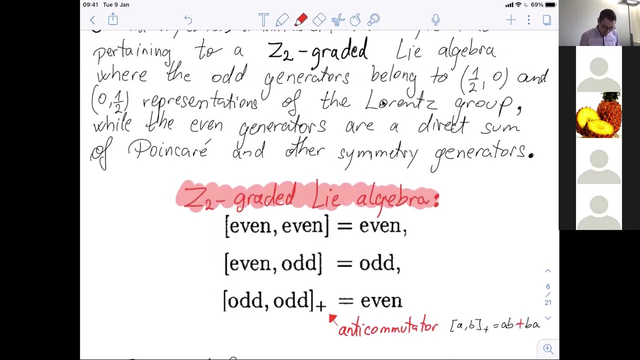 by going beyond the Lie algebras. So supersymmetry algebra is not a Lie algebra. Okay, Actually it is something which is called Z2 graded Lie algebra, And this Z2 graded Lie algebra in simple words means that there are 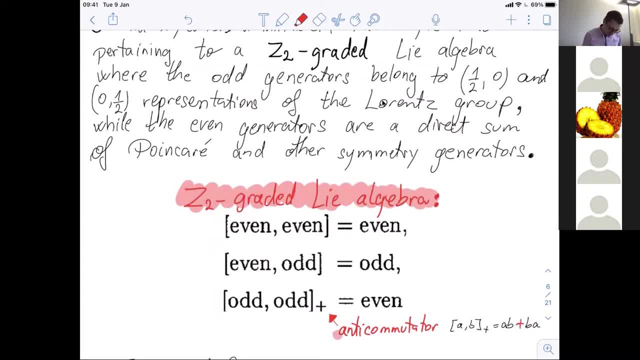 in addition to commutation relations, there are also n anti-commutation relations. In fact, there are two types of generators: even and odd under Z2.. And the even generators, so this one here. this is just, you know, the ordinary Lie. 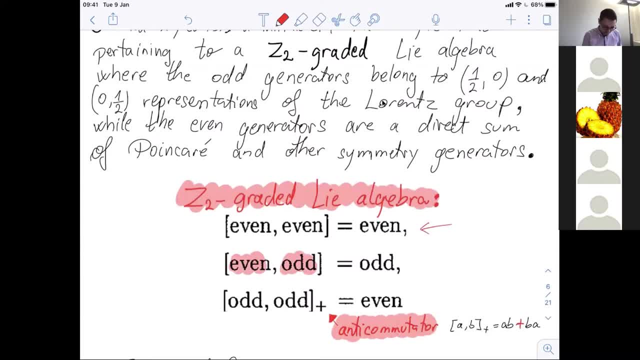 algebra For the even generators: they obey the ordinary Lie algebra. And the odd generators, they, when they commute, they don't have a Lie algebra. So the even generators, when they commute, they don't have a Lie algebra. So the even generators, they obey the ordinary Lie algebra. 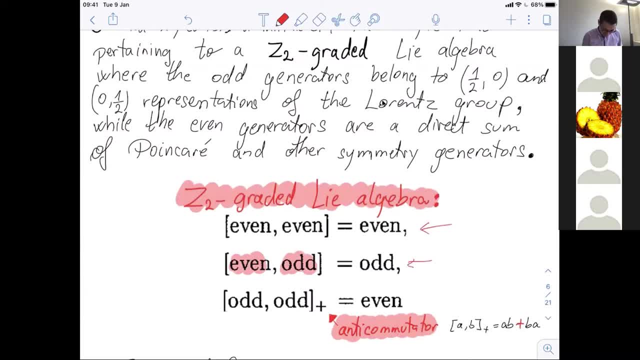 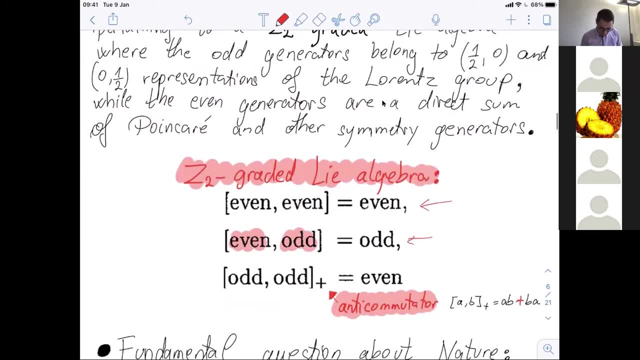 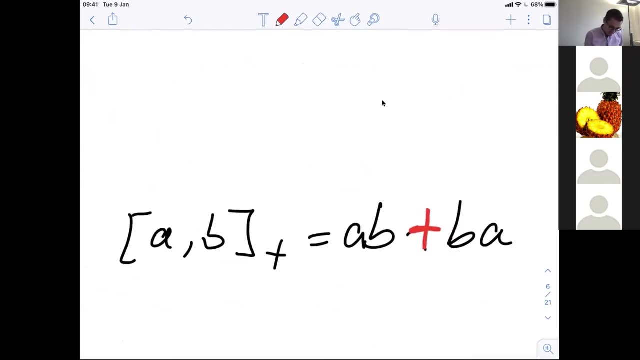 So the commutator with the even generator gives an odd generator and the anti-commutator gives the an even generator. So what the anti-commutation is is basically this relation. So this is the. in some literature, this symbol is equivalent to these kind of brackets. Okay, So this is the anti-commutation. 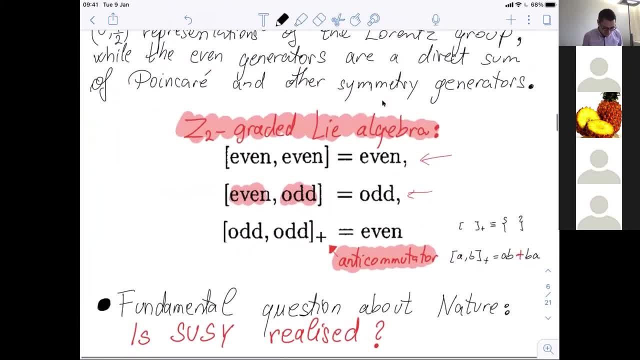 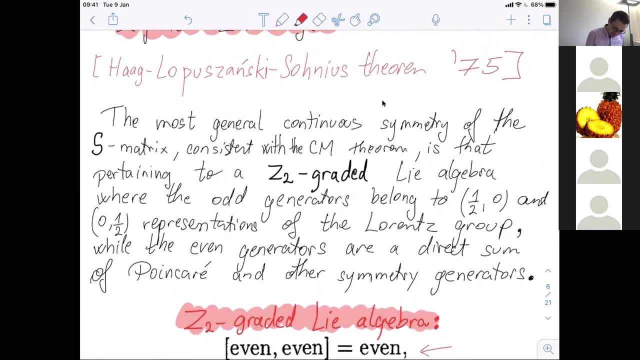 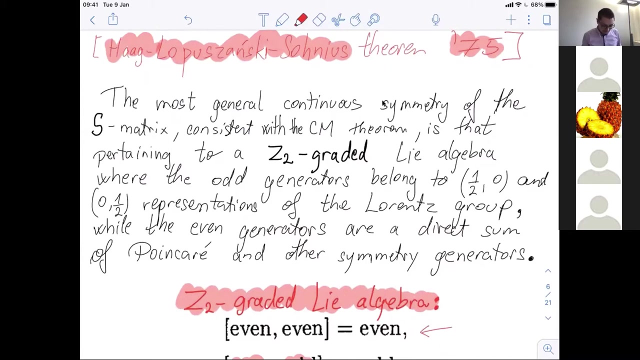 the anti-commutator. Okay, So there is another theorem from 75 by Haag, Lapuzansky and Zonius, which says the following: The most general continuous symmetry of the S matrix consistent with the Coleman-Mandula theorem is that pertaining to a Z2 graded Lie algebra. 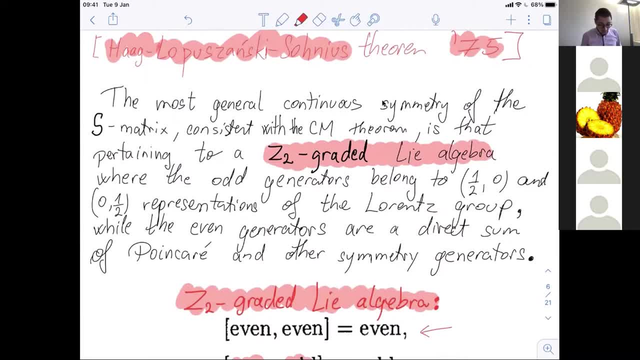 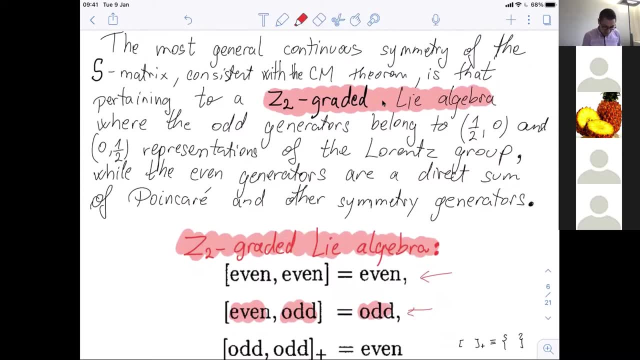 is equal to one half of the representation of the Lorentz group Where the odd generators okay. so the odd generators belong to spin one half representation of the Lorentz group, While the even generators are just the usual direct sum of Poincaré and any other internal 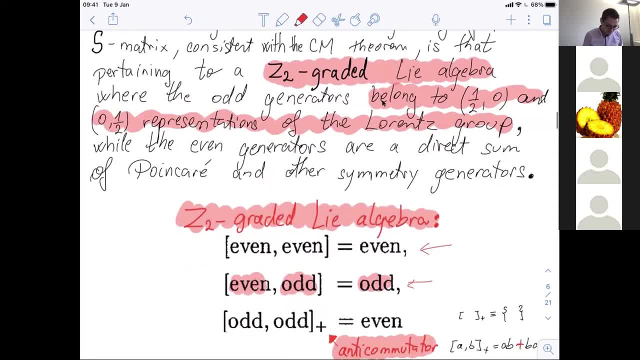 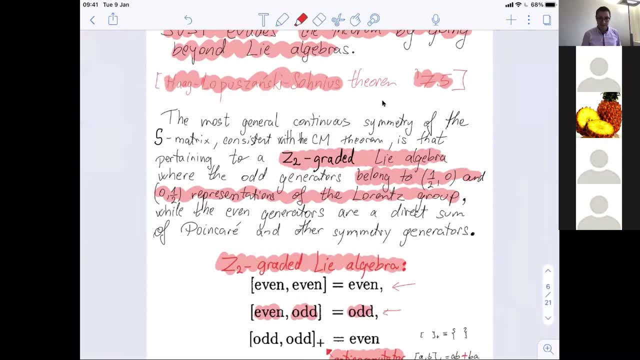 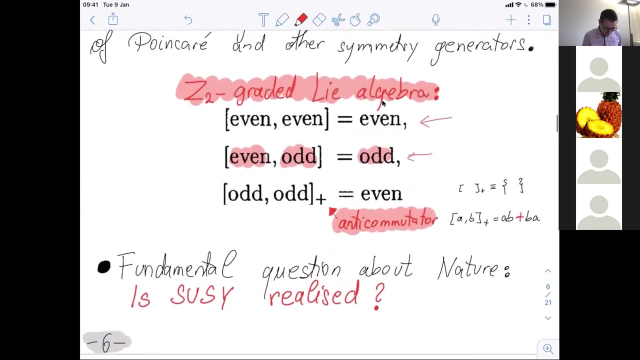 symmetry. Okay, Okay, Okay, Okay, Okay, Okay, Okay. So this kind of underlying structure for the continuous symmetry of the S matrix, it gives a consistent quantum field theory. And now the fundamental question is at this point, really the fundamental question about nature is: is supersymmetry realized? 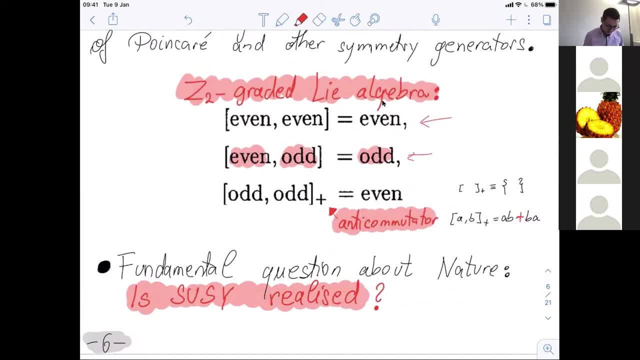 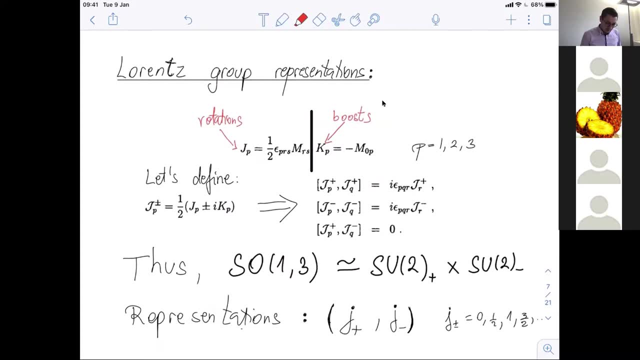 Okay, Well, let me quickly remind you of the Lorentz group representations, given that the odd generator, the supersymmetry generator, is spin one half representation of the Lorentz group, just to explain a bit better what this means. So the Lorentz group contains rotations. 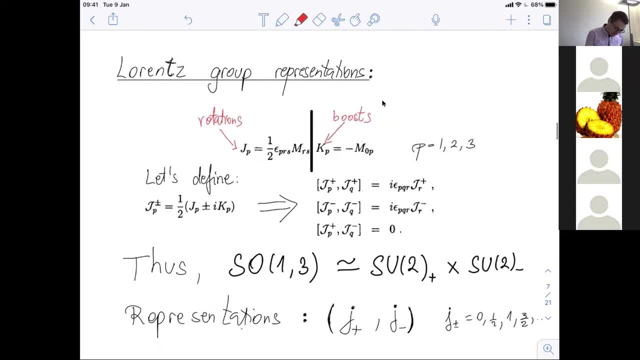 and boosts. Okay, So these are in particular rotations and these are boosts. These are some specific elements of this, of the M mu nu tens generator. So we do the, we do the, the red redefinition, and we can basically write down the algebra, the Lorentz group, as the direct sum of the two. 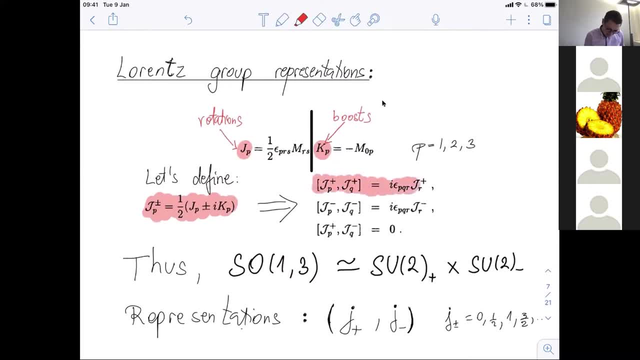 algebras. So you see, these J plus generators form an algebra on their own, the same as the J minus, And the commutator between the two is zero, meaning that it's a. it's a trivial combination of the two. So the the Lorentz algebra. 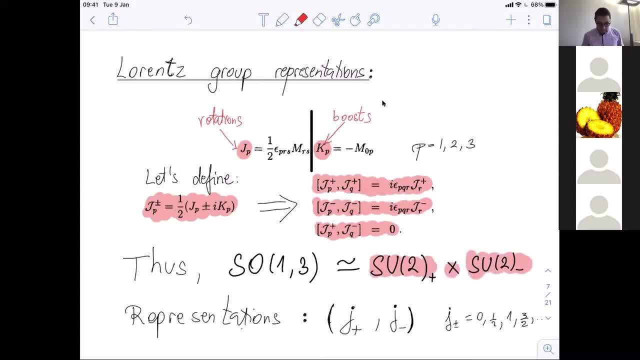 is basically this, the combination of the SU2 plus and SU2 minus. So SU2, we know how to deal with finite dimensional representations. They are basically half integers spins Integer and half integer integer and half integer spins, and the representation of the Lorentz group is the ordered pair J plus, J minus, where 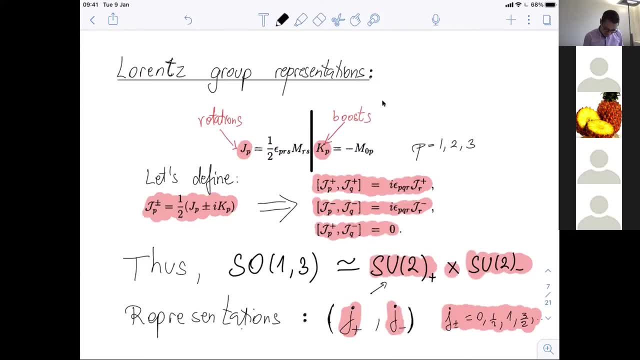 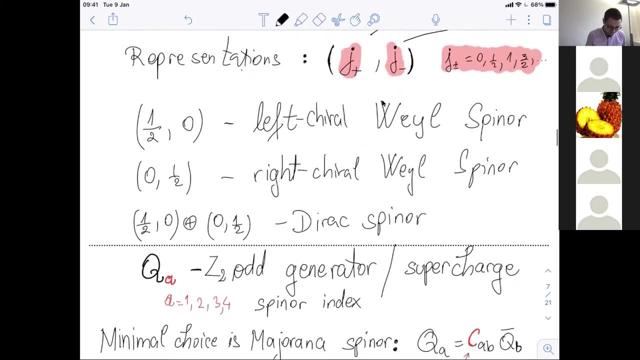 J plus is the representation under SU2 plus and J minus under SU2 minus. Okay, so this is the representation, finite dimensional representation of the Lorentz group. So the the theorem which I'm not even going to explain should be called Thorian Estado's Gods of JA. particle two is: H is- I am using the whole formula for this question- the theoretical bre 하는데 Management. i de Beaumont, i Pfallisse, who Pfallisse? Gouvert is also Pfallisse, and so Pcallisse runs those geometries10710. 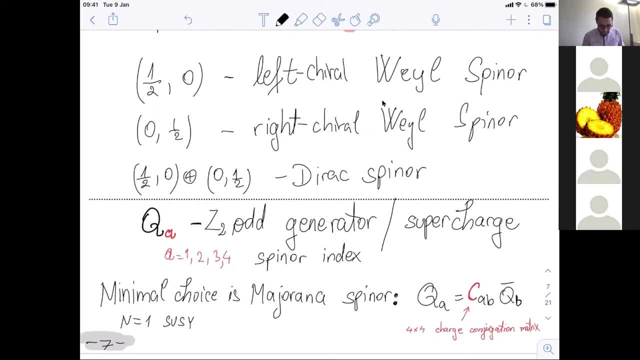 which evades the Coleman-Vandula theorem. the supersymmetry theorem says that the odd generators from the Z2 graded Lie algebra are actually in one half comma zero or zero comma one half. the representation of the Lorentz group. These are left chiral. 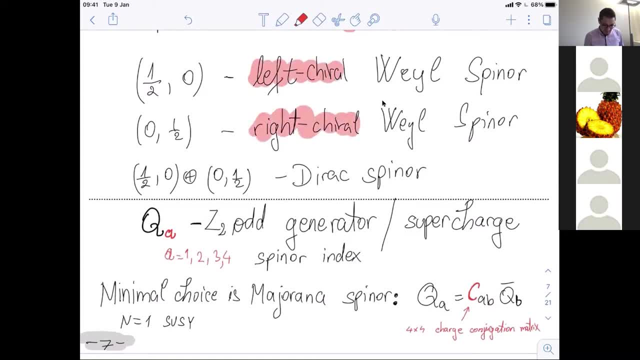 and right chiral Weyl spinors respectively. I'm sure you're familiar with this. This is studied when you study fermions in quantum field theory, you study Weyl spinors. The Dirac spinner is the direct sum of these two irreducible representation. 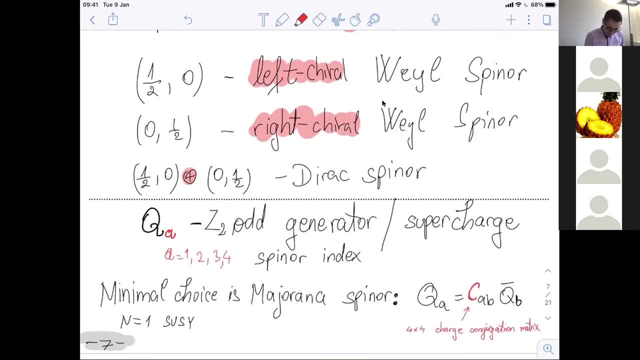 So this representation is reducible. It can be reduced as a direct sum of left and right chiral, Right chiral spinors. All right, So the Z2 odd generator of the super algebra, we will call it Q And it carries this index A. 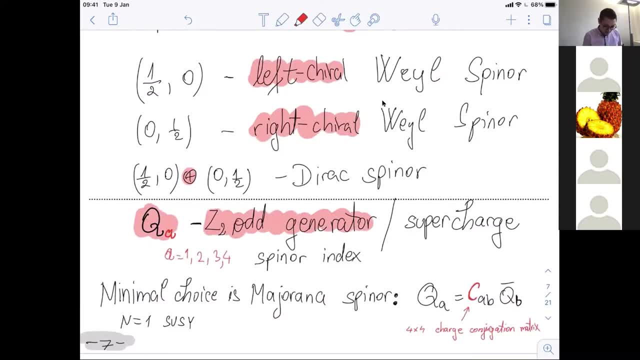 and this index is in the Dirac space. Okay, In the spinner space It's a spinner index which go one, two, three, four. So we will take a minimal choice, meaning to take one Weyl spinner and we can out of Weyl spinor. 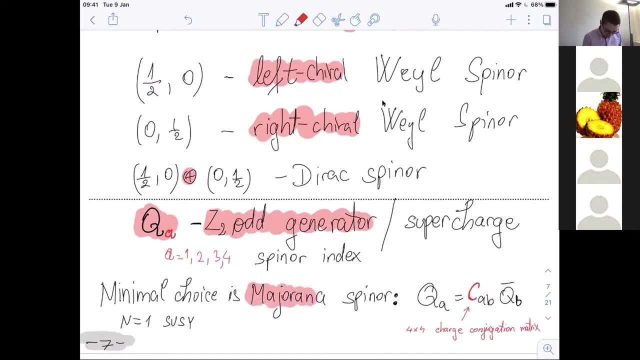 we can make a Majorana spinner. A Majorana spinner we can make by the charge, by imposing the charge conjugation, So saying that the charge conjugate is the charge conjugation on the spinner. And this is basically the encoded in this C matrix. 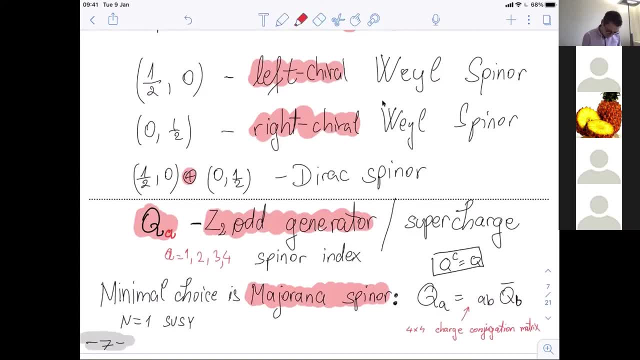 Okay, So the It's encoded in the C matrix. This is just a minimal choice And this is called an equal one supersymmetry. So we have only one additional odd generator. You can have N equal two, N equal three and four, So on As many as you wish to put in, And in fact N equal four supersymmetry is very important. example of an equal four supersymmetry is very important. example of an equal four supersymmetry. 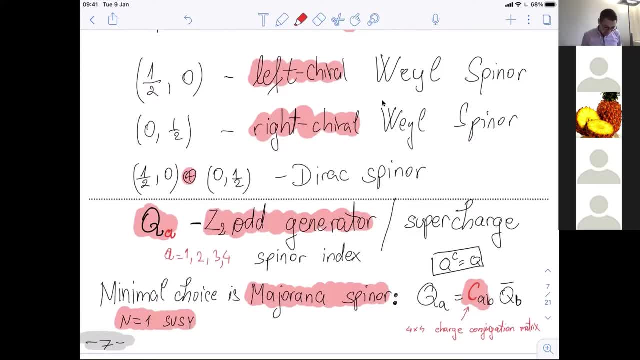 of an equal four supersymmetry is very important. example of an equal four supersymmetry in studied in theoretical physics. for the moment we will stick to an equal one supersymmetry and we, so our generator is is a. you can think of it as a four. 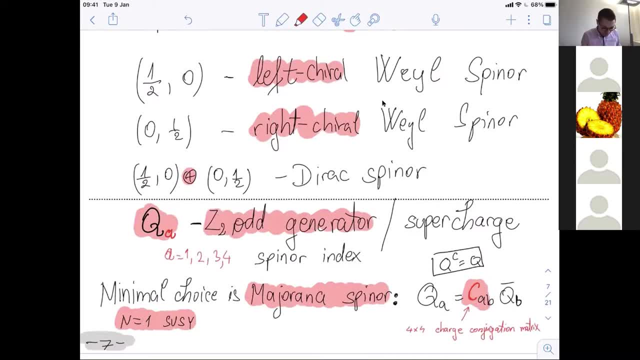 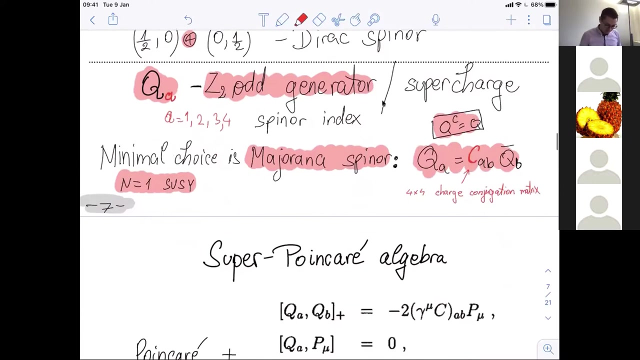 component spinner. four component spinner: it will in fact be a Majorana spinner, satisfying this equation. satisfying this equation which means that the spinner, the charge it's the spinner, is equal to the charge conjugate. okay, so this is the super Poincare algebra. so the super Poincare algebra. 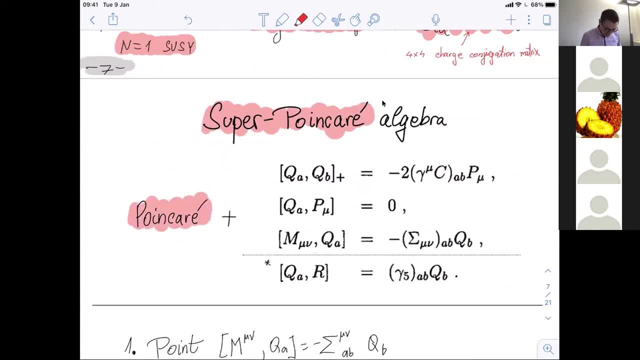 so it consists of the Poincare algebra plus these three additional relations, and so the third one you should forget for the moment and focus only on the on the first three. so Q is the odd generator of the Z2 graded Lie algebra. P and M are the translations and 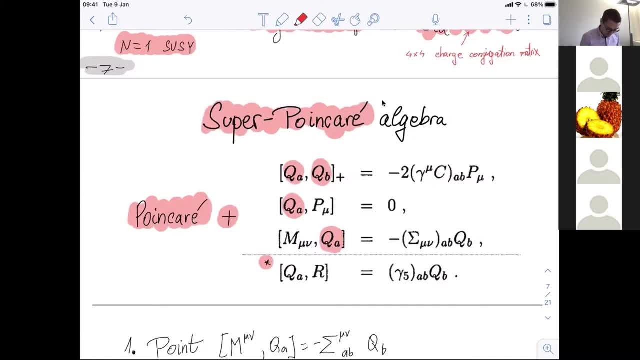 Lorentz, generators of the Poincare algebra. so the first equation says that the anti-commutator of the of the two odd generators gives translations, space-time translations. the second equation says that the, the, the odd generator, commutes with the with the space-time. 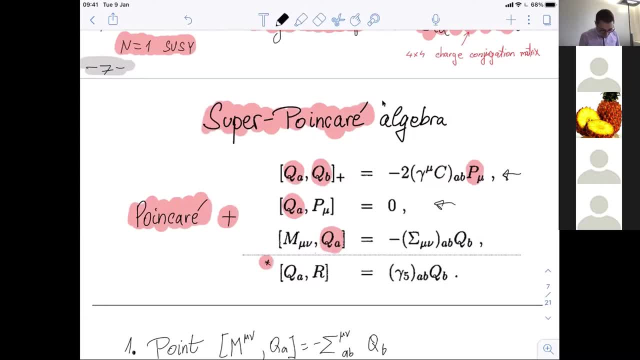 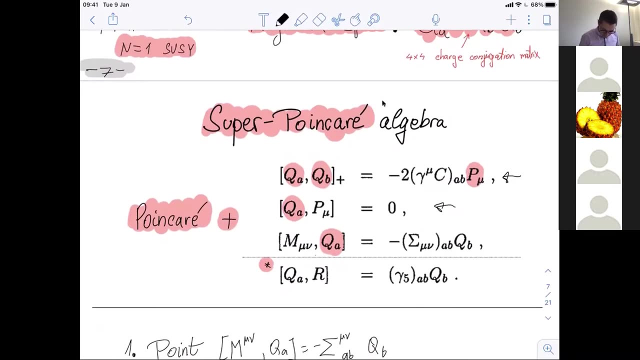 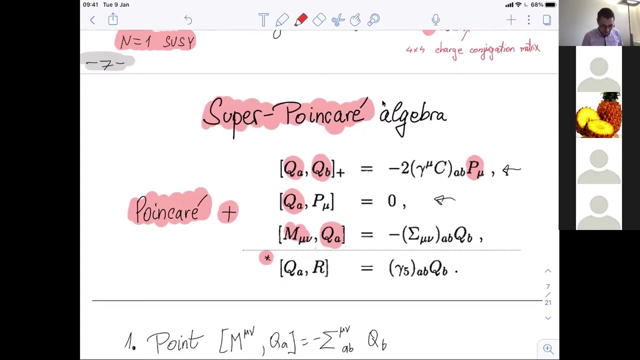 translations and the. the last equation says that the odd generator is: is. is some representation under this, under the, the Lorentz transformation? okay, so I will call this odd generator from now on a super charge, because it's a, it's a generator of supersymmetry and it. 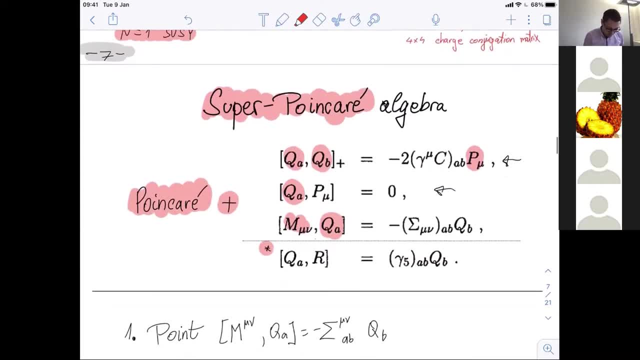 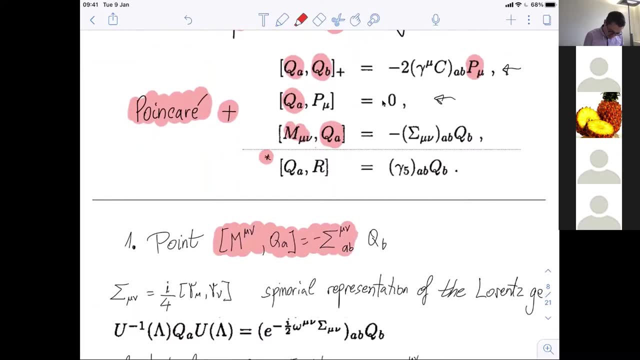 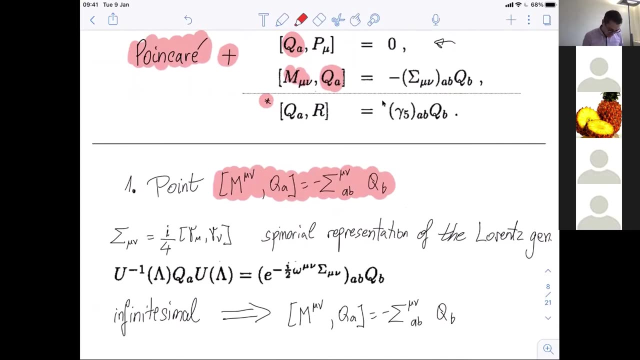 really is a charge in another sense. so let's start with the, with the, with the last relation, which is this relation. so this sigma is basically, in terms of gamma matrices, in Dirac space, is the commutator of the gamma matrices, sigma mu nu and, if you remember this from, from the, 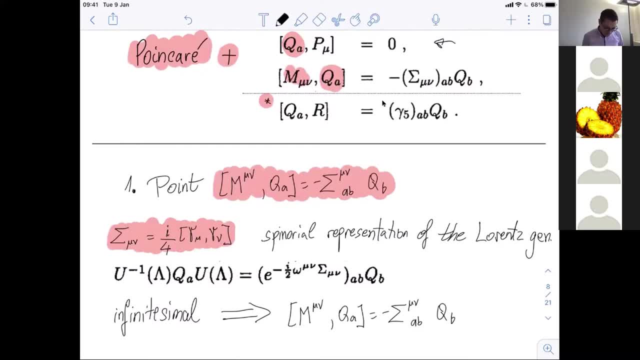 from Dirac spinors. this is the, the representation of the Lorentz group, the spinner representation, the Lorentz group. or in other words, this equation: here is how the, the, the, the, the field transforms. you take a fermionic field, it's an operator and you do a transform, Lorentz. 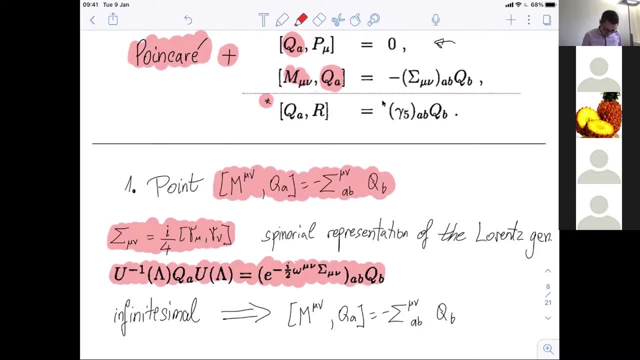 transformation, then this is the, the form of it. I mean so it. these are: sigma mu nu are the generators and omega mu nu is the group, elements, okay, parameters. So if you take the infinitesimal limit, so saying that these omegas are infinitesimally small, 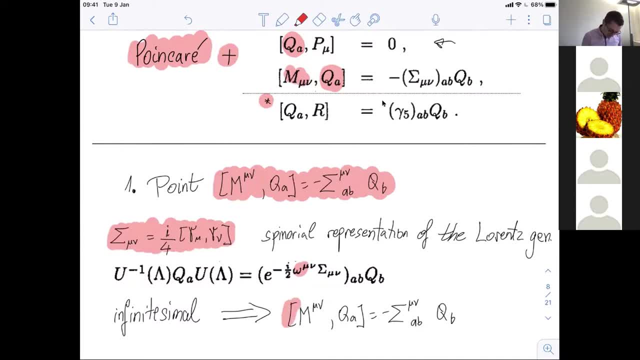 and you expand this equation, you would get the algebra. So what does this mean? It's basically our definition that the Q, the supercharge, is this particular representation of the Lorentz group- spin one half fermion. okay. So supercharge is not a field, it's just a fermion, okay. 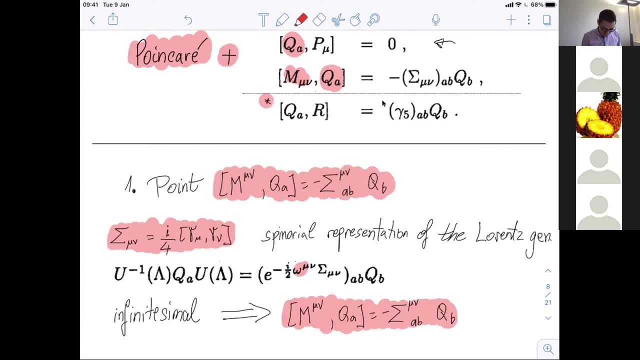 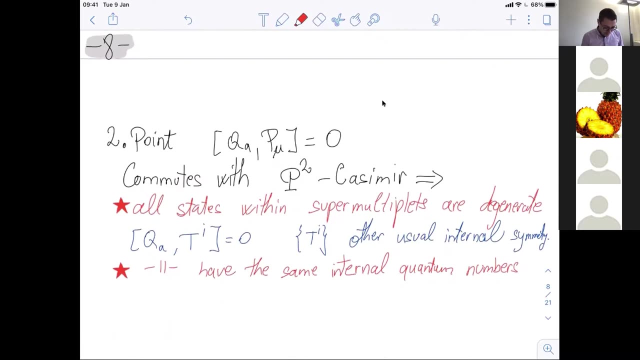 There is no X, so there is no okay. So this relation just tells us that the supercharge is a spin one half fermion. Okay. so now the second point. we saw that the supercharge commutes with the space-time translations. 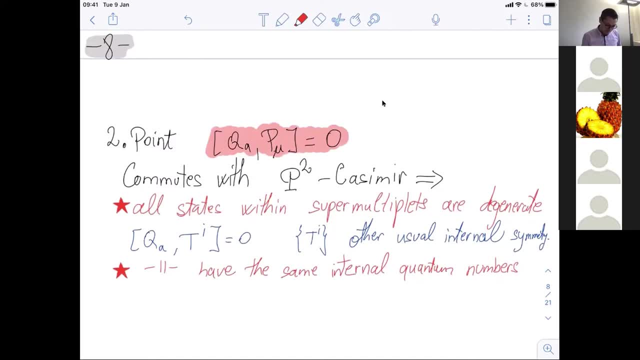 This has a consequence that the components of the supermultiplet, so states in a supermultiplet, will be mass degenerate, So they will have the same mass. So you put the bosons and fermions in this supermultiplet, they will have the same mass. 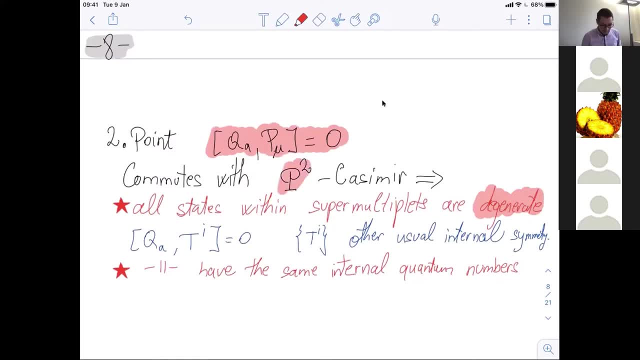 Why? Because the Casimir p square commutes with the supercharge. The same holds for other usual internal symmetries, for example gauge symmetry. So the generator of the gauge symmetry commutes with a supercharge And therefore the particles within a supermultiplet. 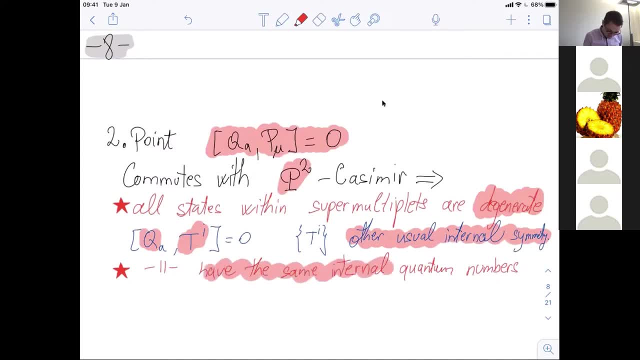 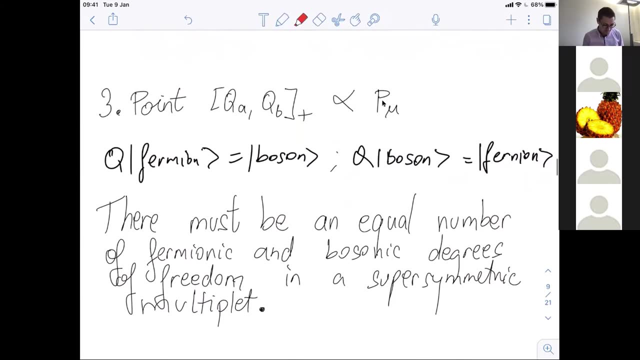 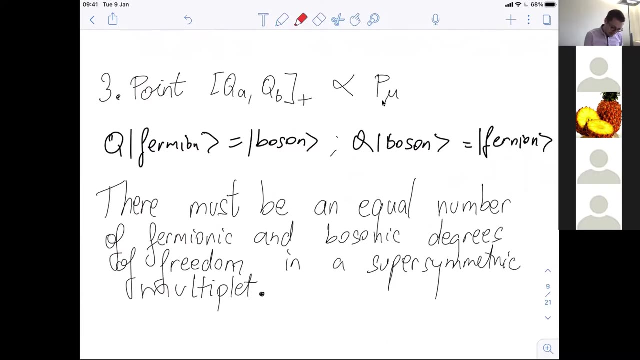 will have the same internal quantum numbers. Okay, Okay, And the third point is related to this algebra, this relation, And one can derive from this relation, basically that within a supermultiplet there has to be an equal number of fermionic and bosonic degrees of freedom. 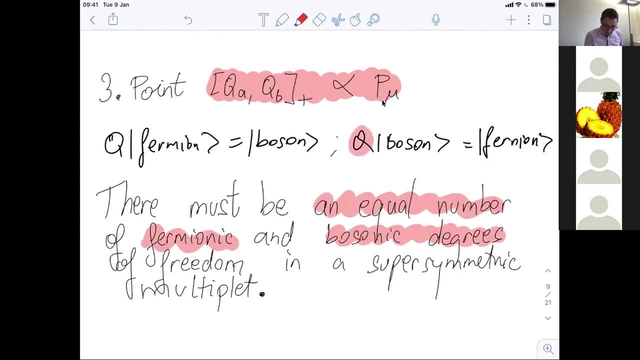 So Q is a spinner. Now, when it attacks on a boson, it will give a fermion. This is just to be Lorentz-like. This is a spinner, And also Q when it attacks on a fermionic state. 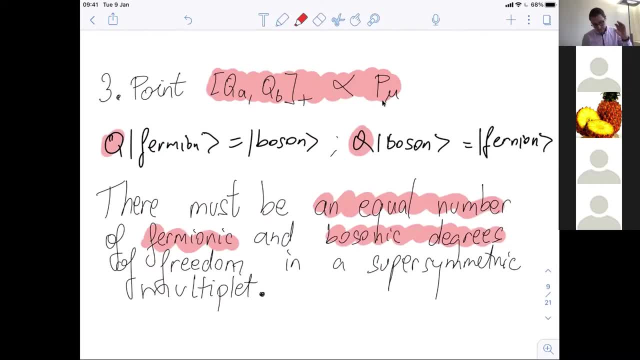 it will give a boson state. So Q is this generator of supersymmetry which takes one component of the supermultiplet bosonic one and transform it into fermionic one. And this equation, this anticommutator, tells you that, being proportional to the translations, 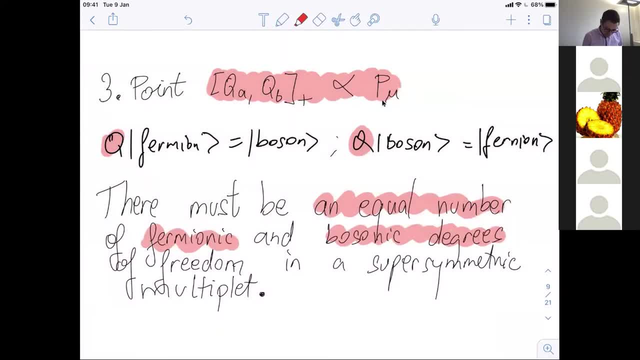 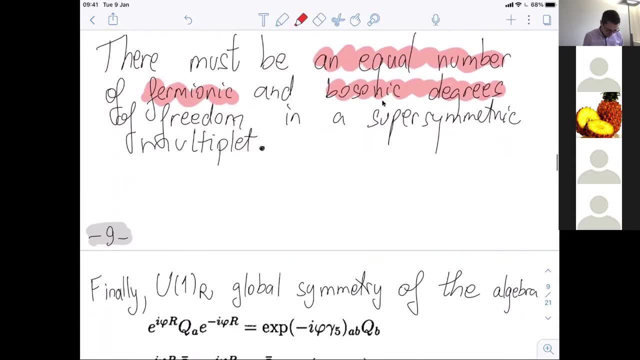 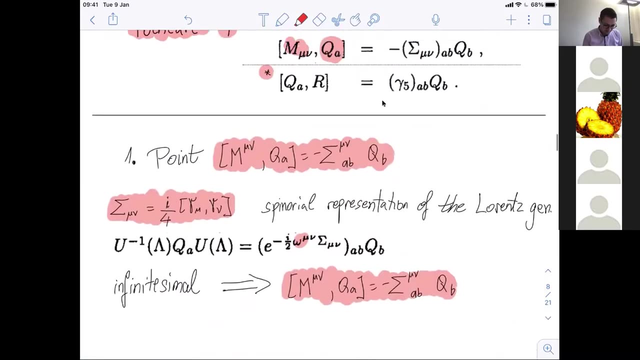 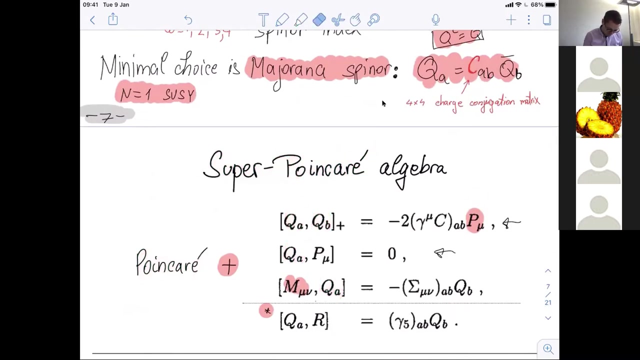 tells you that you should have an equal number of fermionic and bosonic degrees of freedom in a supersymmetric multiplet. Okay, So are there any questions at this point related to the superpoint carry algebra? Yes, I mean. I would have just a question on the last point. 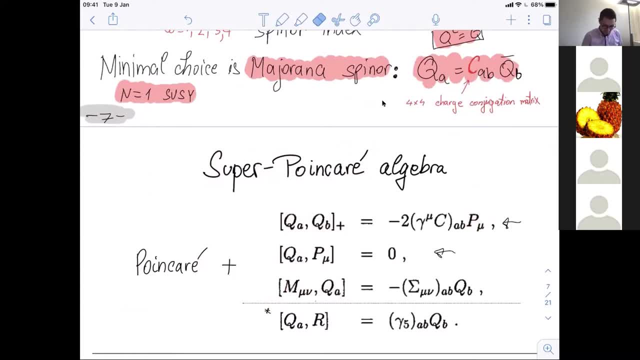 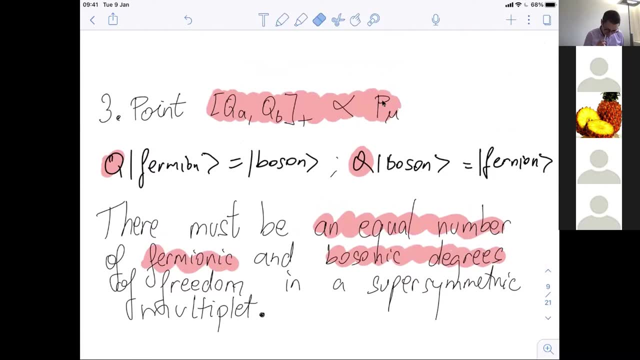 So I didn't get this connection. So from this anticommutation relation does this follow that when Q acts on a fermion, you get a boson? Yeah, so there is a lengthy derivation of this result. I'm just stating this result. 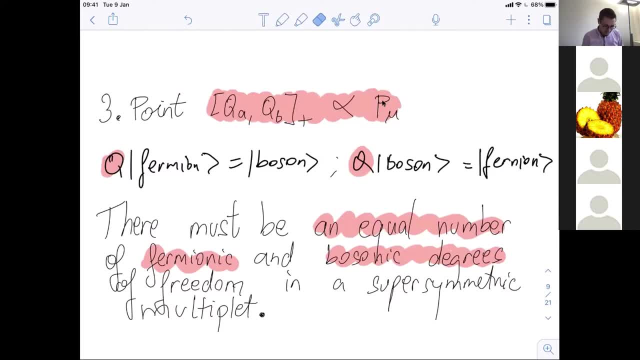 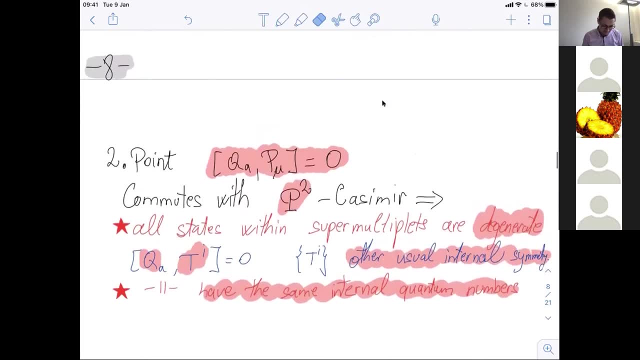 Yes. So this algebraic relation tells you that there is an equal number of fermionic and bosonic degrees of freedom in a supermultiplet. This one tells you that within a supermultiplet, of course, when supersymmetry is preserved. 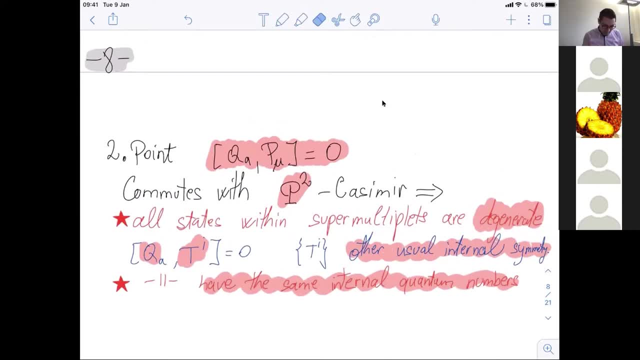 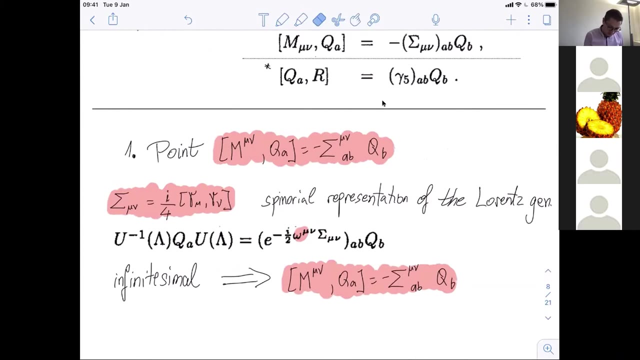 the particles, the states are mass degenerate And, furthermore, they have the same internal quantum numbers under the, for example, gauge symmetry. They are in the same representation of the internal symmetry And this one, this relation of the superpoint, carry algebra. 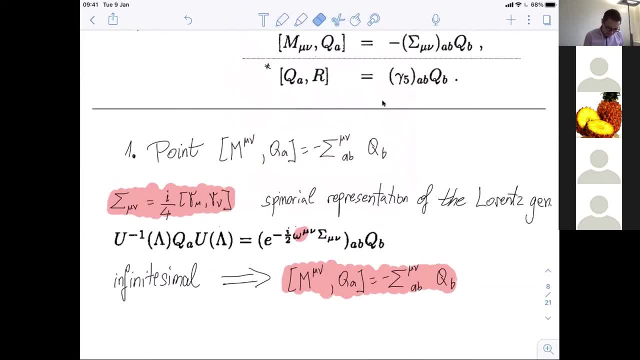 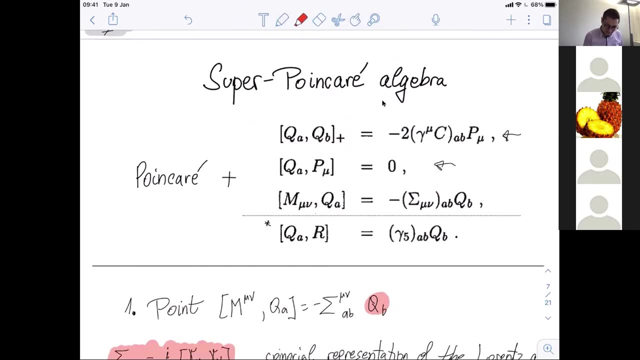 tells you it's simply a defining relation for QA of superpoint carry algebra Of the supercharge, saying that the supercharge is a spinorial representation, spin one half representation of the Lorentz group. Okay, But maybe these three things is worth remembering. 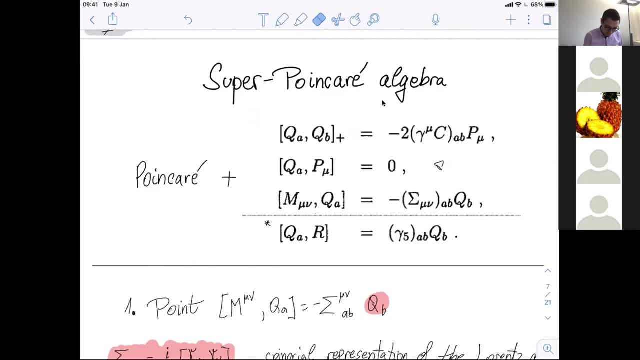 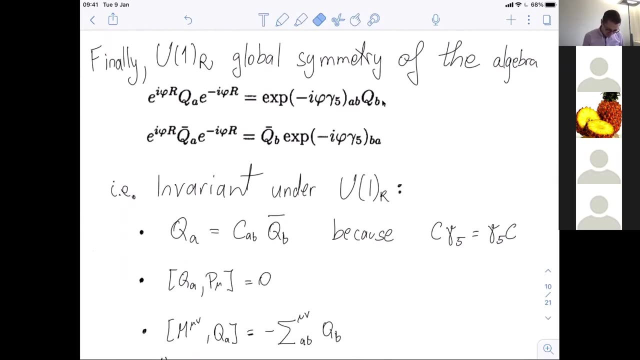 about the superpoint carry algebra. that underlines the supersymmetry. Okay, Thank you. Okay, So there's this subtlety about the globals, the global symmetry of the algebra. If you remember, there was a fourth relation which does not belong to the algebra. 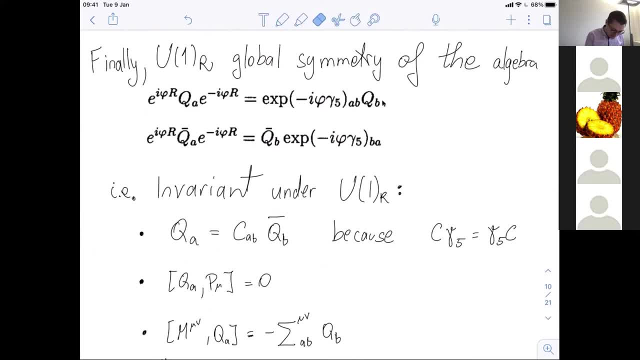 but it is the following. So, in particular, one can notice that the algebra has a global symmetry. Okay, The algebra has a global symmetry, one In particular when you change the field in this way, with this chiral gamma, five chiral way. 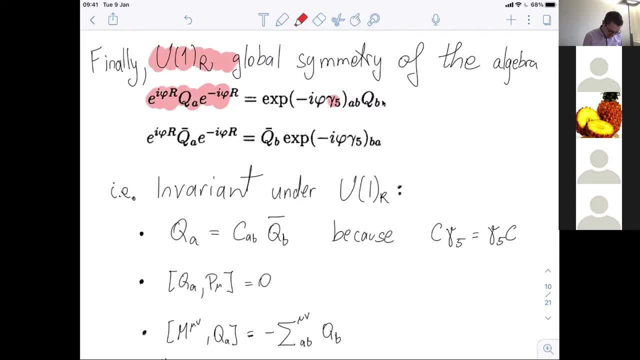 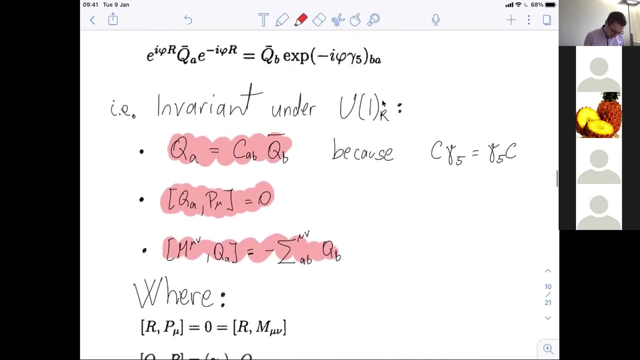 then you have all these relations, invariant meaning they stay the same. Okay, So in particular, this one and that one and that one. Okay, And so it's in particular meaning that there is some unitary generator, R which commutes with the point carry generators. 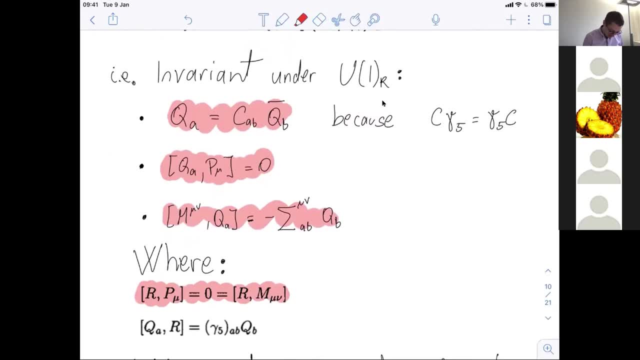 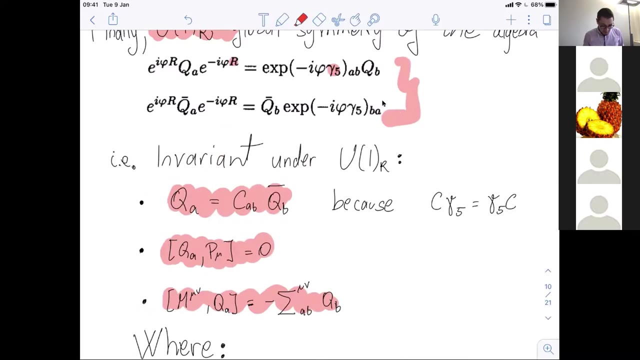 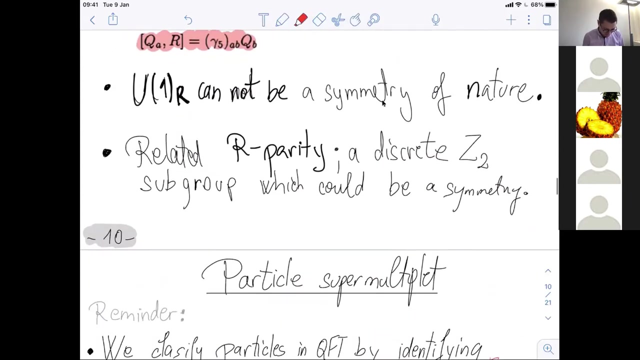 however, it has this non-trivial commutation with the supercharge, And this last equation simply follows from these two things. Okay, So the super algebra has this U and R global symmetry. Why is it good for? It's just a minor, it's technical detail. 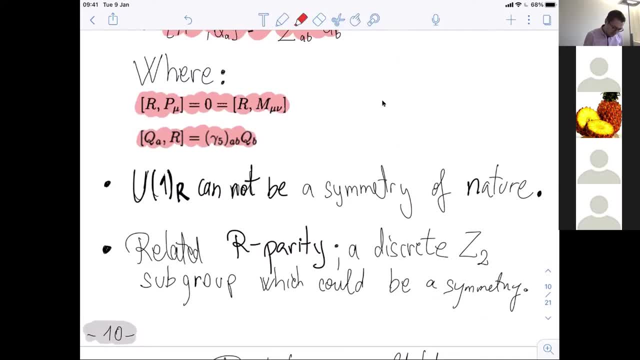 which I want to go quickly. So, first of all, this U and R cannot be a symmetry of nature. It's anomalous and broken by some interactions. However, there is a discrete subgroup of it, So meaning the U and R is just the symmetry of the algebra. 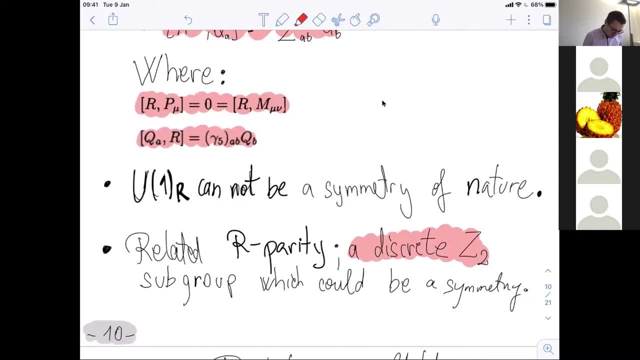 but not necessarily of Lagrangian. Okay, So there is a related discrete subgroup of it which is called Z2 discrete subgroup. So U1 is a continuous group, Z2 is a discrete group subgroup which is called R parity. And this R parity could be the symmetry of Lagrangian. 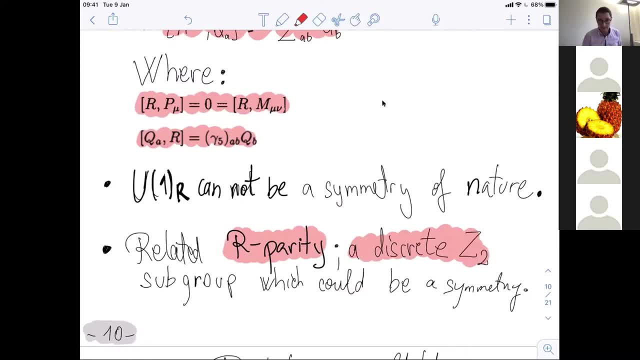 It will play a role in MSSM. So, in particular, ordinary particles- to give you to jump a little bit ahead- will be even under this R parity, while their super partners will be odd. And for this reason, this R parity will be even under this R parity, while their super partners will be odd. 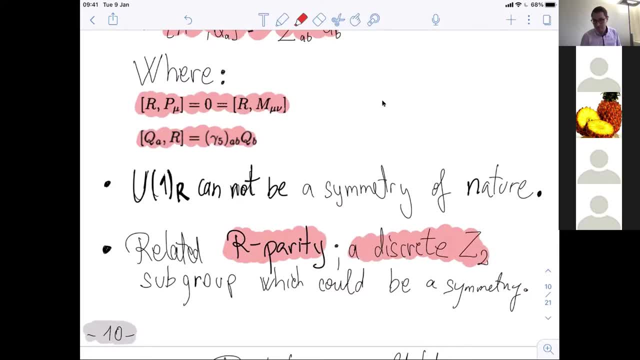 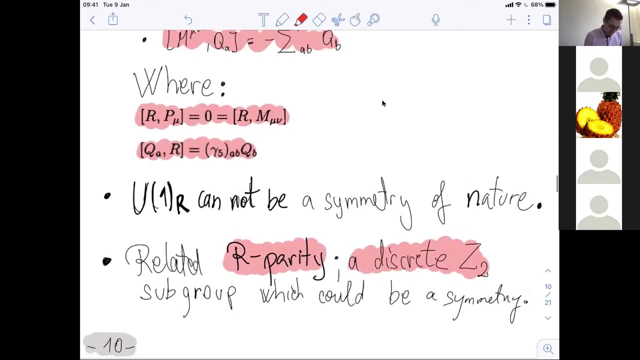 And, for example, the lightest supersymmetric particle cannot decay, It will be protected. Its decay will be protected by this R parity, which means that that thing could be, for example, a candidate for dark matter or something like that. So, just to keep in mind the existence of this global U1R. 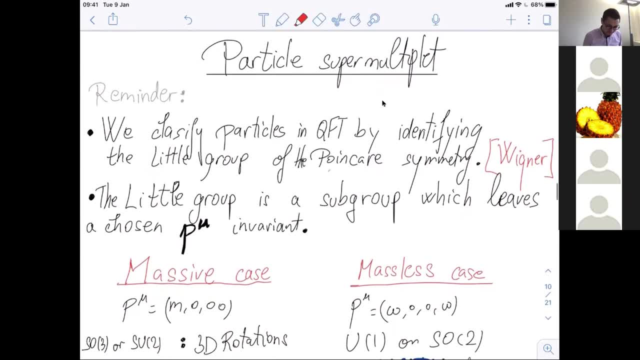 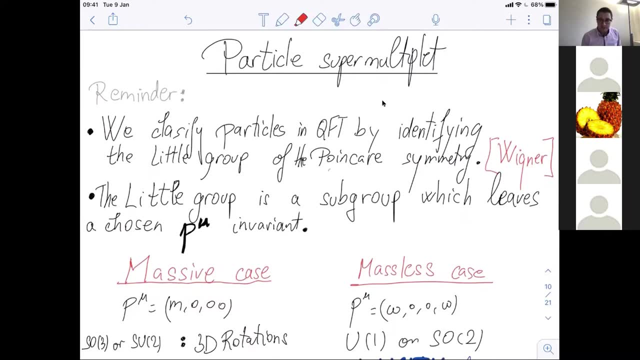 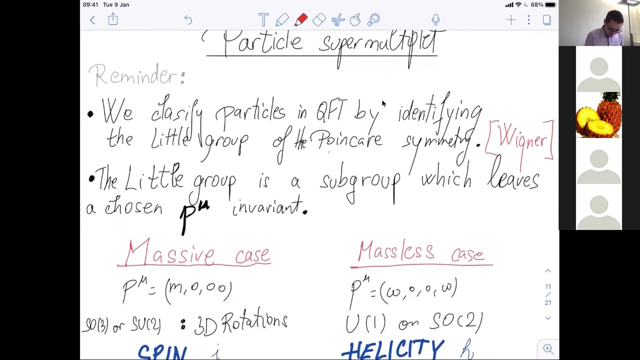 which leads to R parity. Okay, Okay, Any questions about this? Okay, If not, I will move to the super multiplet: a particle super multiplet. So I first want to remind you how we classify particles. We do this by the so-called 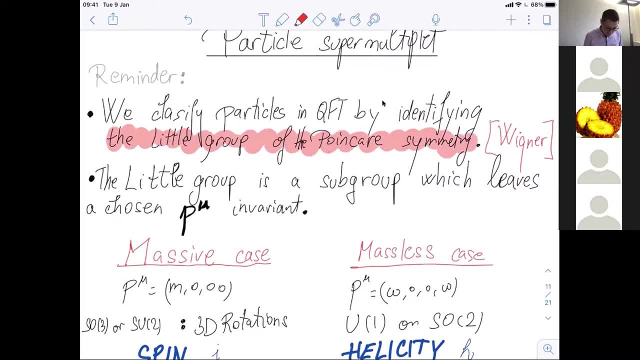 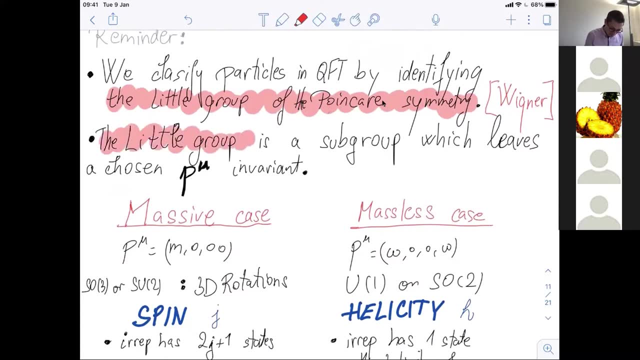 the little group of the Poincaré's symmetry. The little group is a sub group of the Poincaré's symmetry which leaves the group R 1 R. This group here is a sub group, the chosen for particle momentum invariant. so remember that if you so you want to classify. 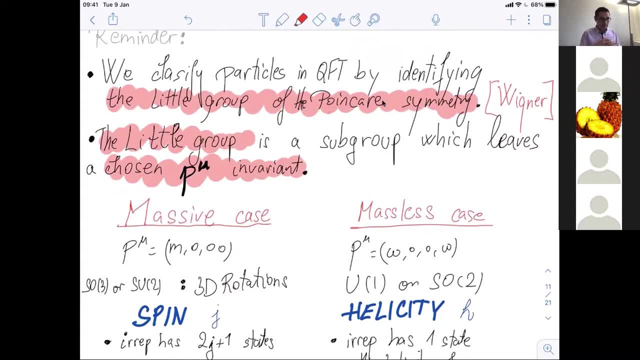 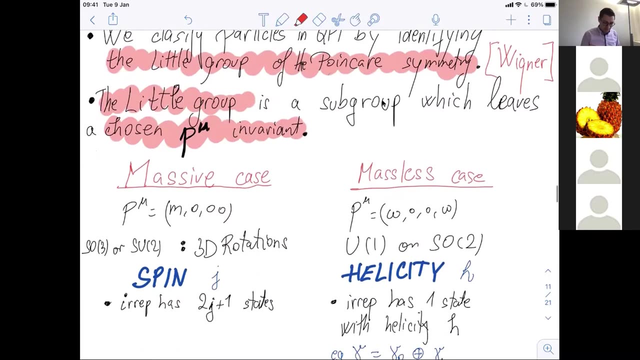 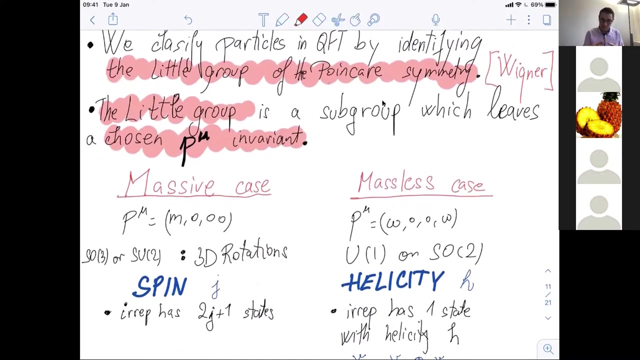 the states under point carosimetry, and the momentum, the four vector of the energy, and momentum is a continuous parameter. so these are infinite dimensional representations. so so how do you do this? you choose a momenta and then you identify a little group. a little group is a subgroup of all point, point career transformations, which would keep this momentum. 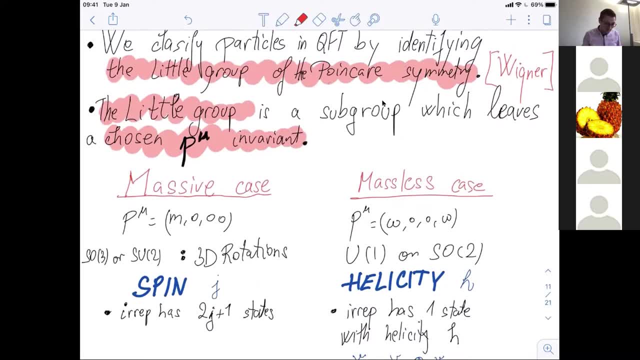 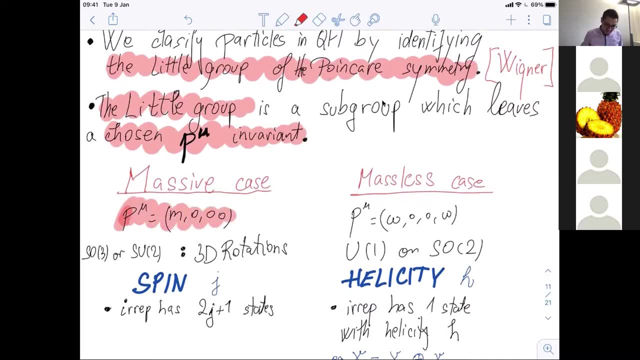 fixed it invariant, okay. so, for example, if you have a massive particle, you can go to its mass frame, and where it doesn't move, so, and then the, the, the subgroup, you can go to its mass frame, and then the, the subgroup, you can go to its mass frame. 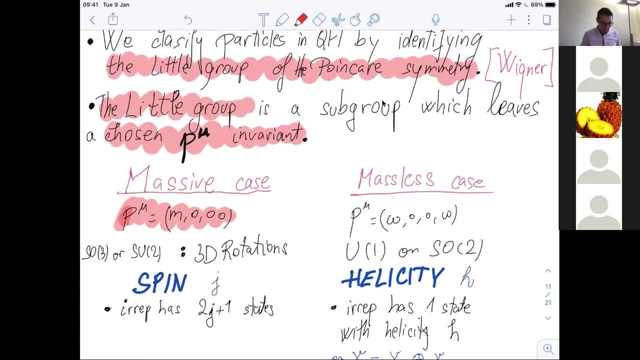 The little group will be simply 3D rotations, which is SU2 or SO3.. This is the little group in the massive case And we know how to classify representation. This is spin, In particular, in the irreducible representation, we have two J plus one states. 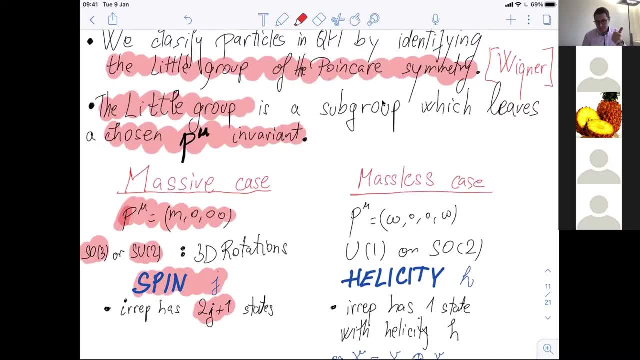 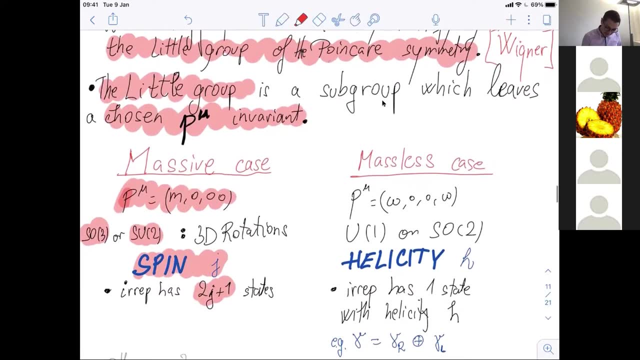 So for the massive particle you say the four vector, for the momentum And then you say the spin. In the massless case you can choose the four vector to be something like this: So there is a preferred direction And the remaining little group. this is a bit of a simplification. 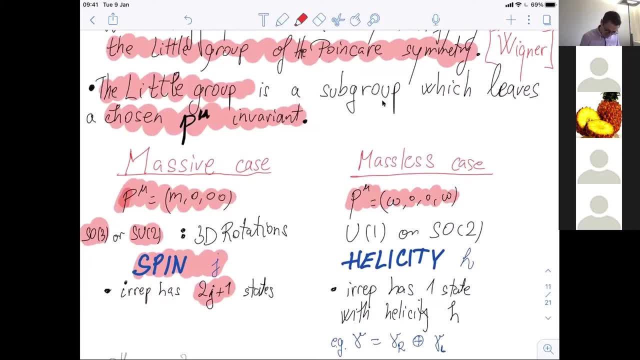 But after the dust settles it turns out to be U1 or SO2.. So you can think of rotations in the perpendicular plane With respect to the axis of motion. And now we talk about the projection of the spin on the axis of motion, which is called. this quantity is called helicity. 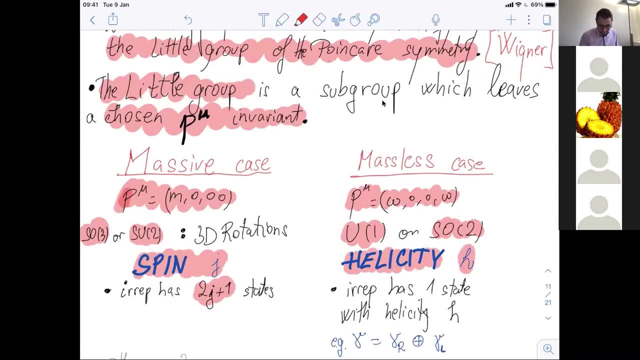 So for massless case we have the quantity which is called helicity. So if you want to classify, say the particle, then you say its momentum- Massless particle- And it's helicity- Irreducible representation- have only one state with helicity: age. 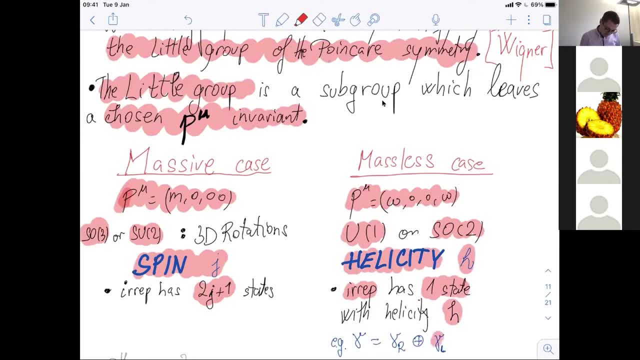 Particular photon can be left polarized. Photon is a massless particle. It can be left polarized or it can be right polarized. These are two. actually these are two irreducible representations. The direct sum is the photon under the little group. 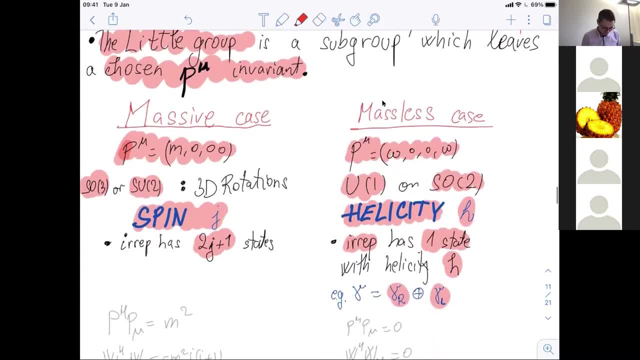 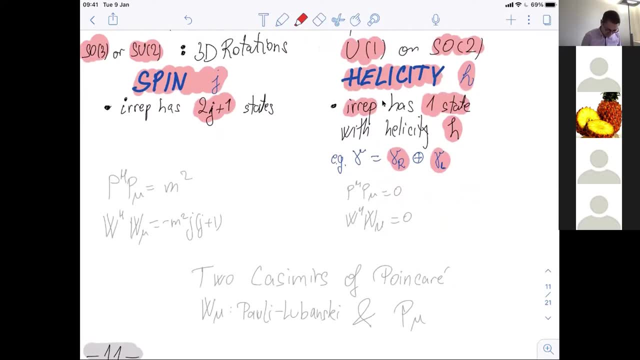 Okay, In other words, we classify the representation of the point career under the Casimir's. And the two Casimir's we have in mind are the built from the four vector momenta and from the Pauli Lubanski four vector. And these are these two Casimir's, P squared and W squared, which gives us the okay. 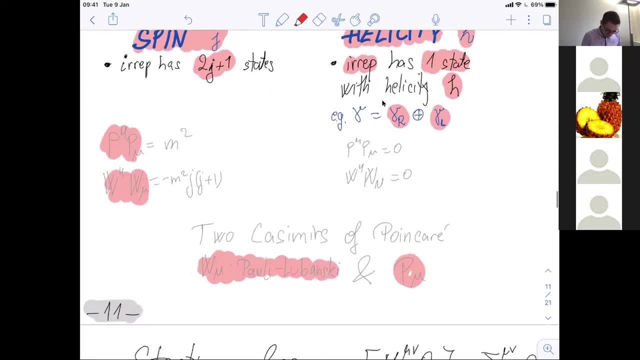 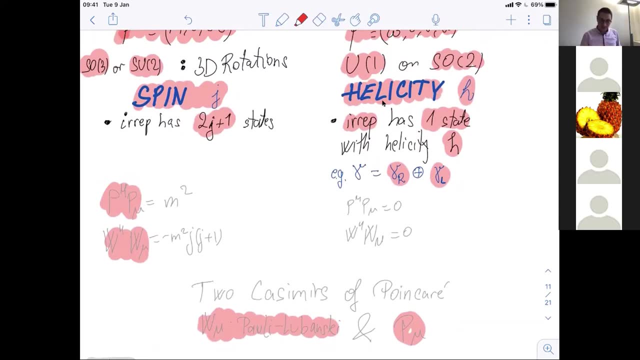 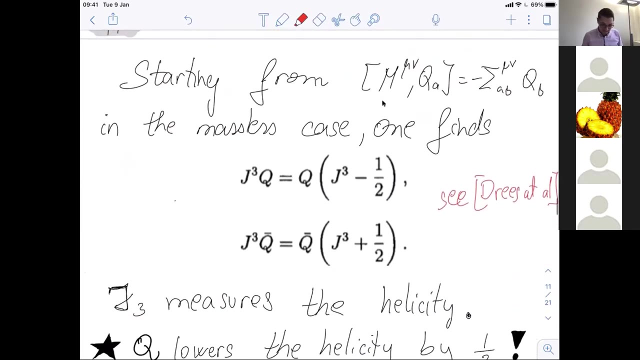 Yes, So it goes this way. So you see that these rotations play a role in defining the, the, the spin or helicity of the particle. So let's go to the supersymmetric case, Remembering that we have this relation in the supersymmetry algebra. 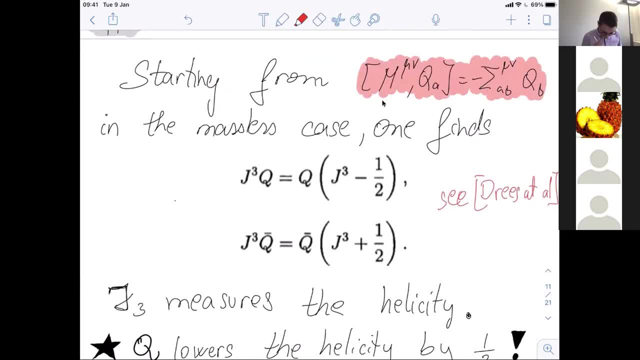 Um and MU nu is are the Lorenzians. These are the Lorenz generators. So let's pick a massless case because it's easier. So if we are in the massless case, we, we, we identified the little group which will be this um, um, we, we identified the little group. 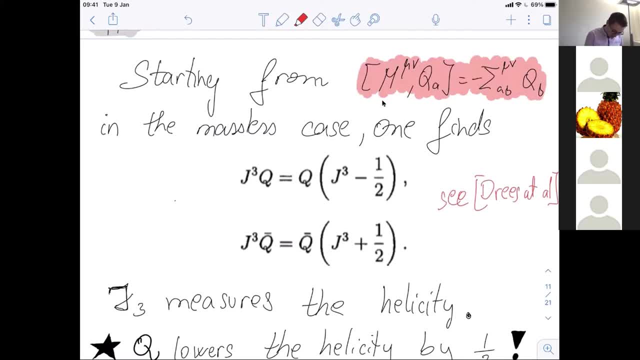 Okay, It will. and then the generator of the little group um will be this, uh J three, the, the projection of the spin on the axis of motion, and it measures the helicity, And so we are going to use the 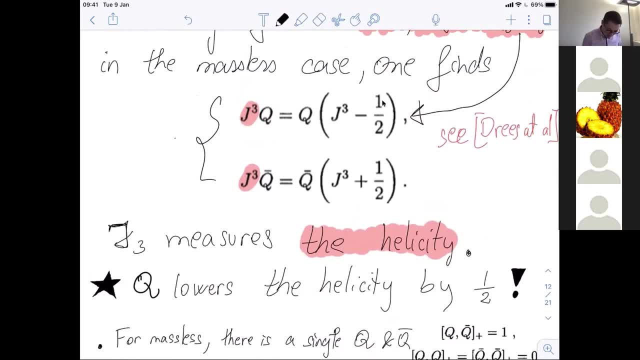 In the matrix of the particle. Okay Now, um, when you start from this relation here, you can arrive to this relation here. This, the, the, the, the two relations just follow from the defining algebra And Please have a look carefully as these two relations, what they tell you. 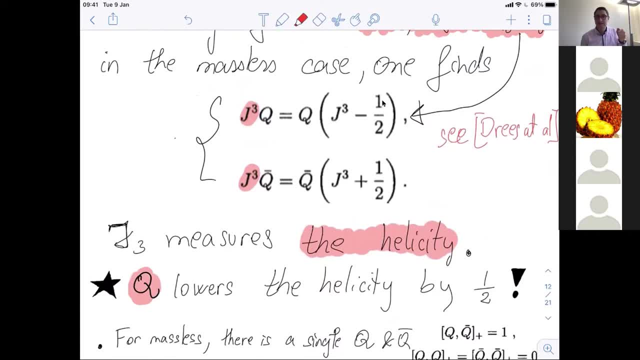 the supercharge acts on a state. in a supermultiplet, it lowers the helicity by one half. These equations should remind you, for example, of these creation and invigilation operators that you encounter, for instance, in the discussion of the SU2 representations. 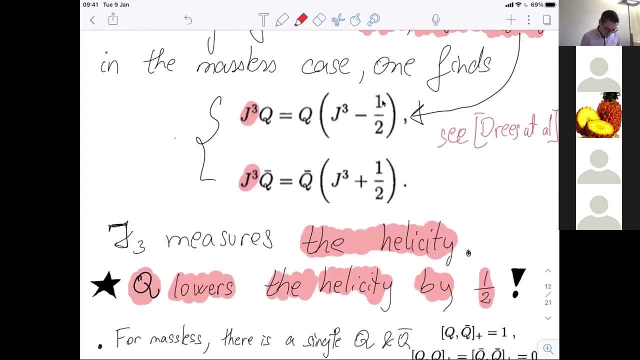 And so Q? is this clear, this point that Q, when it acts on a state in a supermultiplet, will lower its helicity by one half. Or, conversely, if Q, bar the conjugate one, acts on the state, it will increase the helicity by one half. 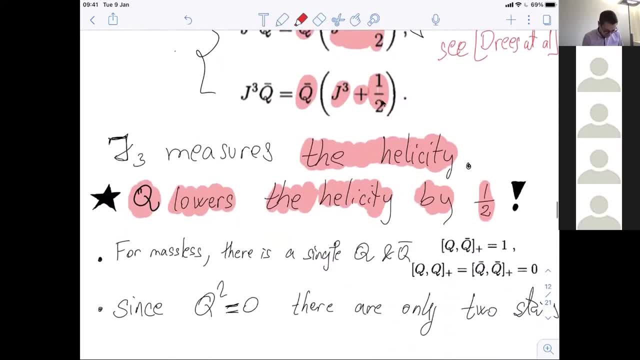 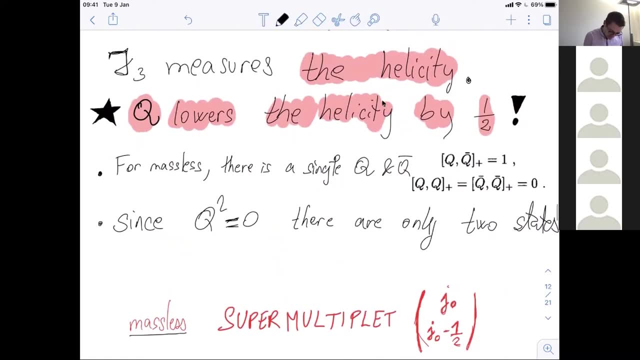 To me that's clear. yeah, Okay, thank you. So one technical thing: remember that Q had indices, et cetera. One can show that in the Maslow's case- a bit of algebra- there is only a single Q. 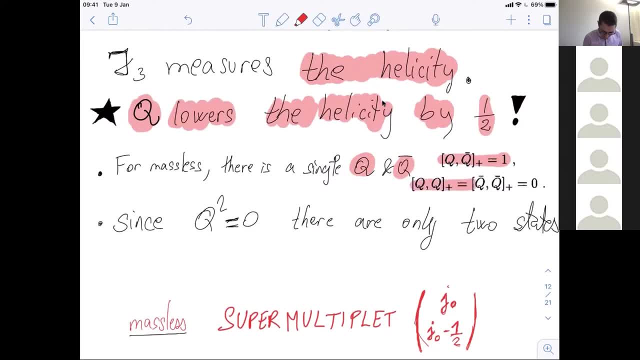 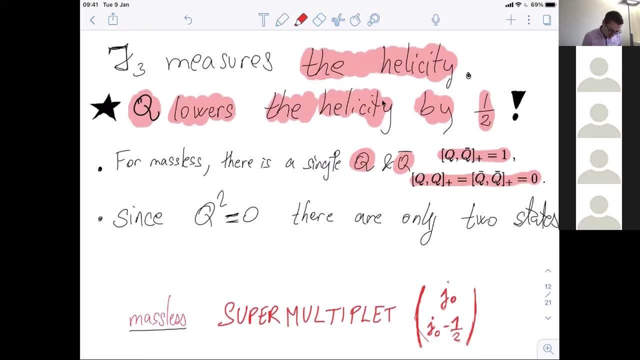 and the Q bar which obeys these relations. This is specific to Maslow's case, And what follows from this is that, for example, Q squared is zero. Why So? Q obeys the anti-commutation relations, For example this one. 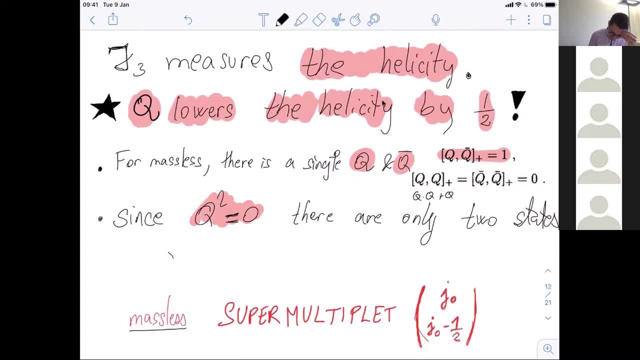 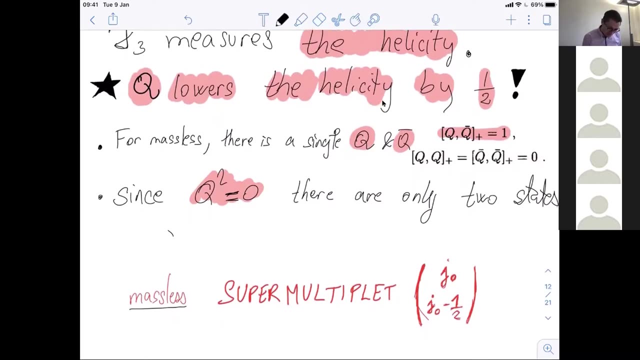 And this one says that Q times Q plus Q times Q is zero, meaning that Q squared is zero. Okay, So this means that there are only two states in the Maslow's supermultiplet. So take, for example, the highest helicity state, J, zero. 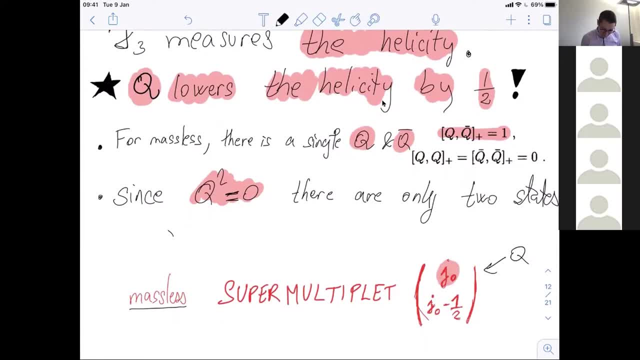 and act on it with Q. This will lower the state. It will give this state, which has a helicity, lowered by one half. Now act again with Q. This means Q squared, This is zero. So you created your multiplet. 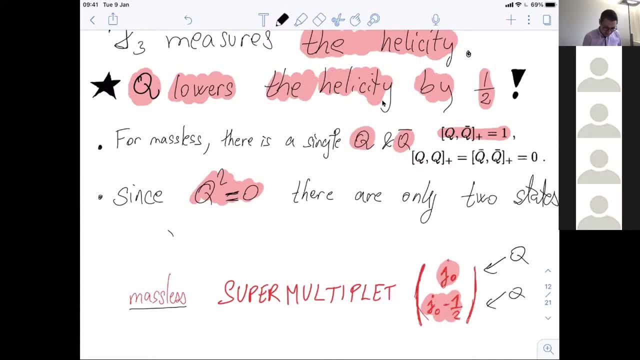 So a Maslow's supermultiplet has two states with J zero and J zero minus one. Okay, This is just a Maslow's case. Massive case is. I will not do it. It's a bit more complicated, of course. 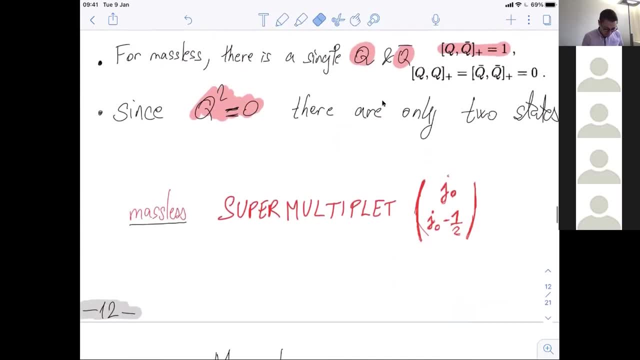 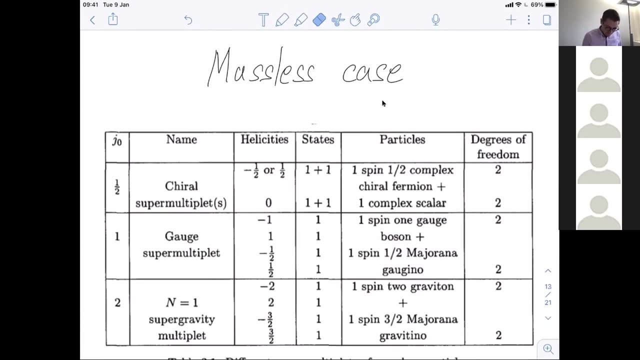 And you can find it, for example, in this book. It's done in great details. So I want to then talk about Maslow's supermultiplet, super multiplets in terms of this J zero, in terms of the helicity of the highest state. 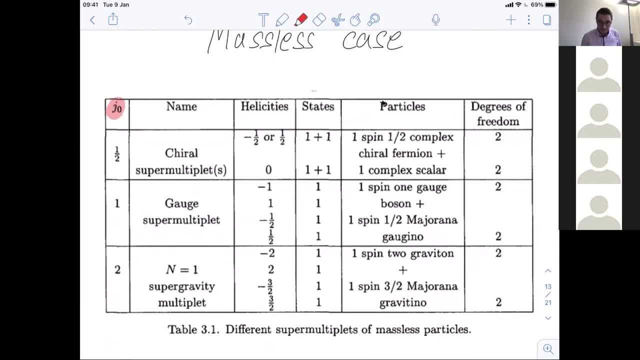 So this table basically summarizes different super multiplets of massless particles. okay, So if you pick, for instance, J zero equal one half, okay, Then the highest component will be one half fermion spin, one half fermion- okay, It will be a Weyl fermion. 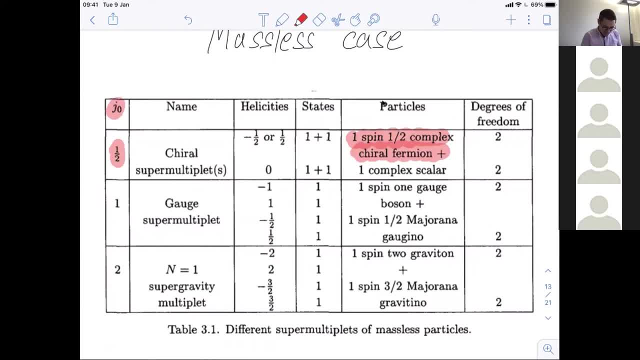 It can be either left or right, So these are usually complex representations under internal symmetries. So how many degrees of freedom are there in Weyl fermion? Weyl fermion has two degrees of freedom, So you can have for in Weyl. 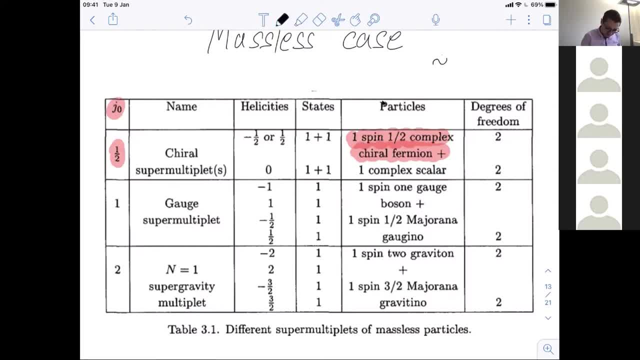 let's say, if you have a Psi L Weyl fermion, then this will describe, for example, left-handed electron and the right-handed positron. So these two states will be created or annihilated by a Weyl fermion. okay, 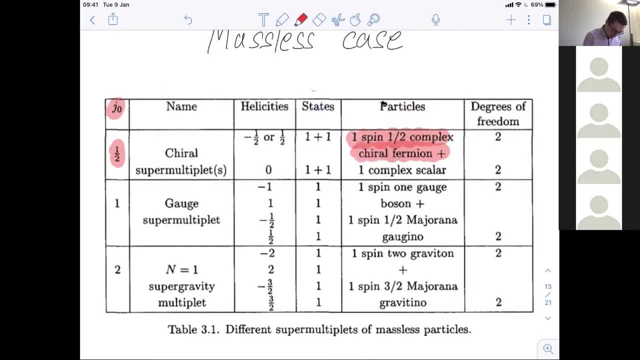 So what is the other component? So this is J zero, that's the highest state, And then we act with the supercharge. It will lower the helicity and we will have this one. It's a complex scalar. okay, It's a complex scalar. 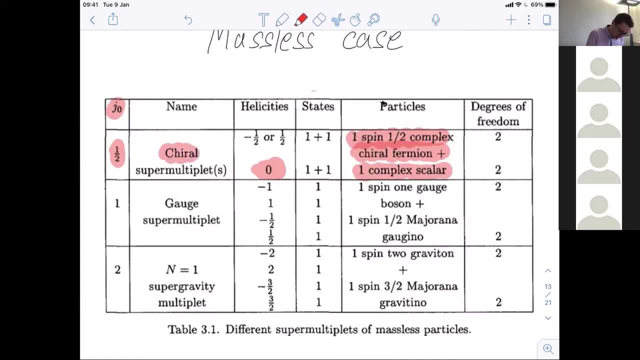 So in a chiral, this is the so-called chiral supermultiplet. The chiral supermultiplet contains a Weyl fermion and the complex scalar. Both of them have the same number of degrees of freedom. The degrees of freedom are two and two. okay. 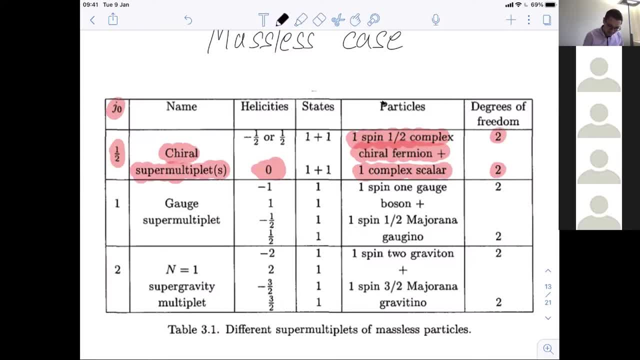 Is it clear why So complex scalar has the real part and the imaginary part? Okay, But for Weyl fermion, which is a two-dimensional spinor, you could say that so it has. Okay, Weyl fermion is a two-dimensional spinor. 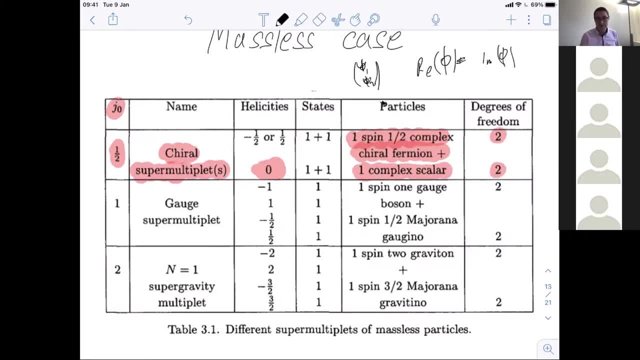 so you can say that perhaps it has four degrees of freedom, But this is oh in fact not true that the on-shell. there are only two on-shell degrees of freedom, and this follows from the fact that the Weyl equation or the Dirac 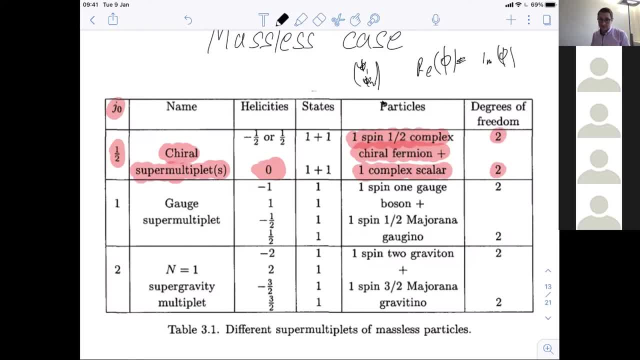 equation is first order, differential equation, and when, in classical field theory, you count the degrees of freedom, so you have the generalized coordinate. generalized coordinate and then the conjugate coordinate. they are one degree of freedom and for the scalar field, indeed, they are independent, because one is q and the other 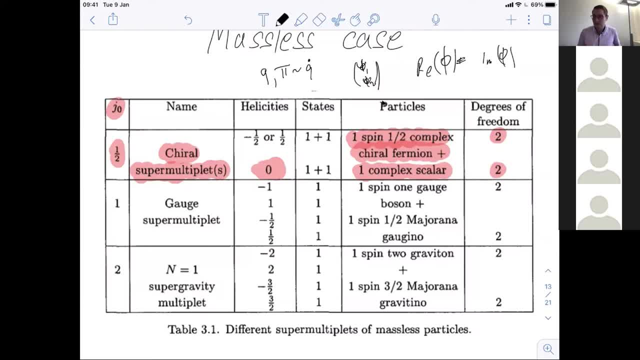 one is q dot and the Klein-Gordon equation is a second order differential equation. but for Dirac equation, which is first order, actually, the conjugate momenta is not independent, it's something like: yeah, it's related to q, so in fact we don't have four. 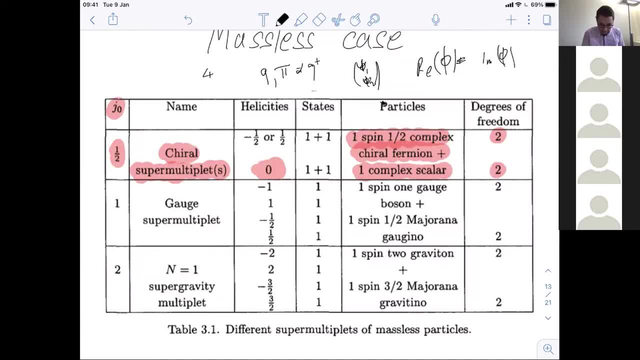 so we have four real parameters in the Weyl two-dimensional spinner, but in fact we have two degrees of freedom, all right. so in addition to the chiral supermultiplot, there are also yeah for different j0. let's say, take j0 equal 1. 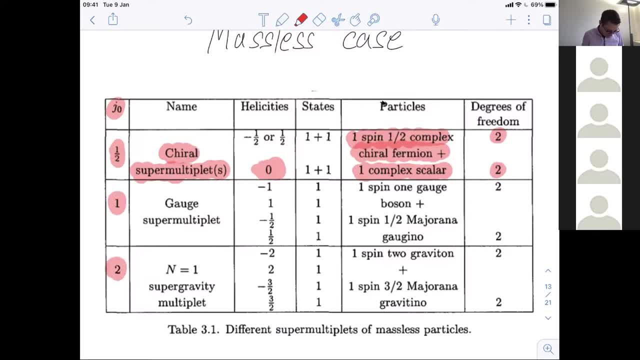 or j0 equal 2, we get what is called gauge supermultiplot, supermultiplot or supergravity multiplet and equal one supergravity. in particular gauge supermultiplot, it has okay particles which have spin, either one or one half, and the helicity can be. 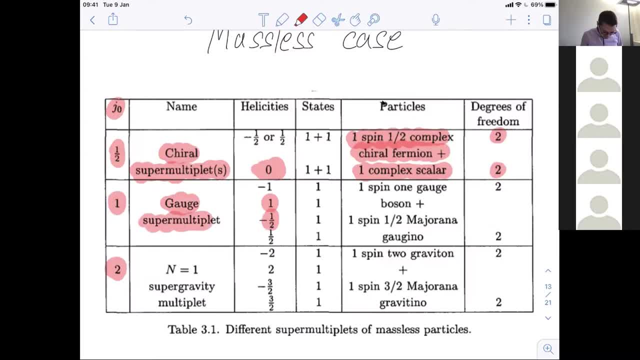 plus, minus, and so what are these? so we have spin one gauge boson. so we have spin one gauge boson. spin one gauge boson is the highest state and then the spin one half fermion. so there is spin one gauge boson and spin one half fermion. 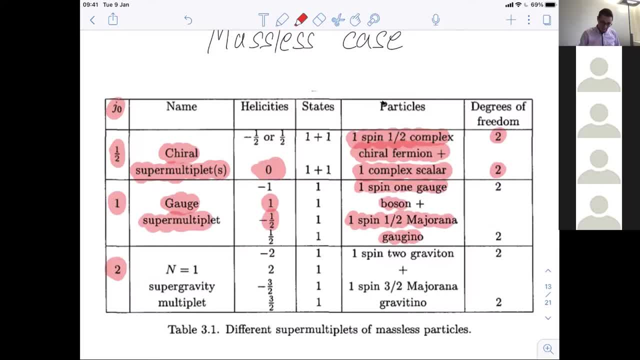 and this fermion is actually a Majorana fermion. so Majorana fermion is built from one Weyl spinner, so it means it has two degrees of freedom. these degrees of freedom are basically particle of some helicity, but it has two degrees of freedom. 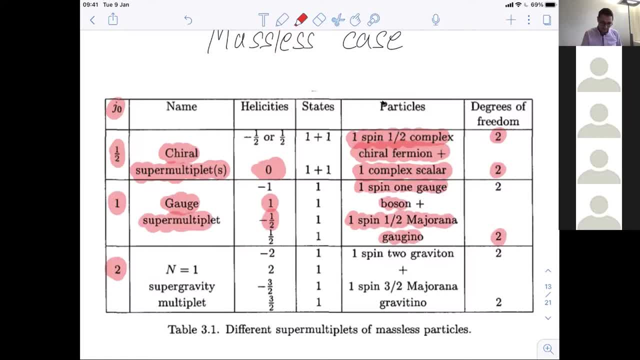 and particle of other helicity, because Majorana particle is the same as antiparticle spin. one gauge boson is in Maslow's case, so it's just like a photon. so it has left polarized and right polarized, so again there are two degrees of freedom for the bosonic. 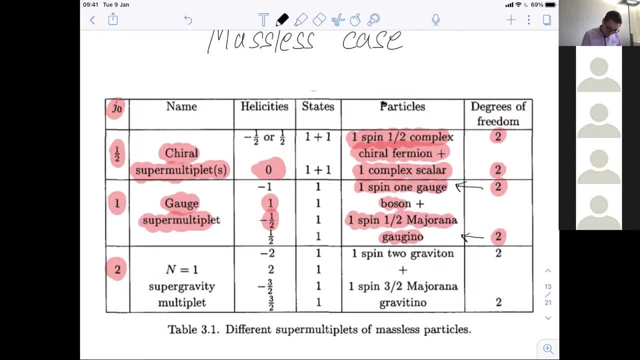 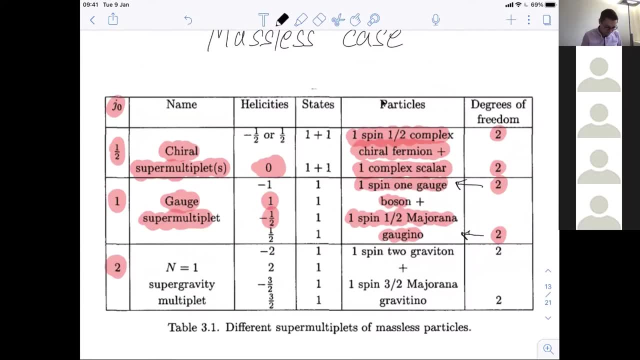 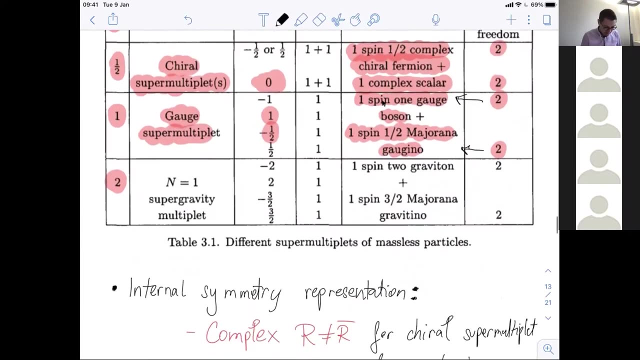 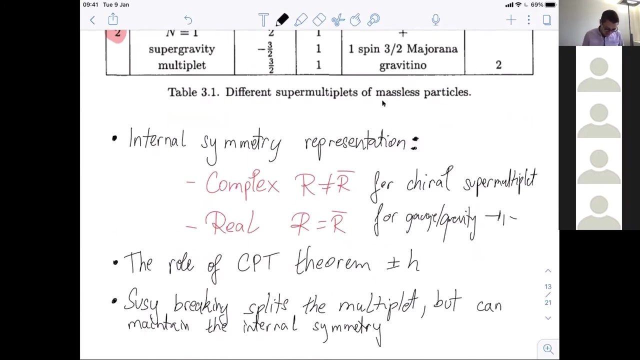 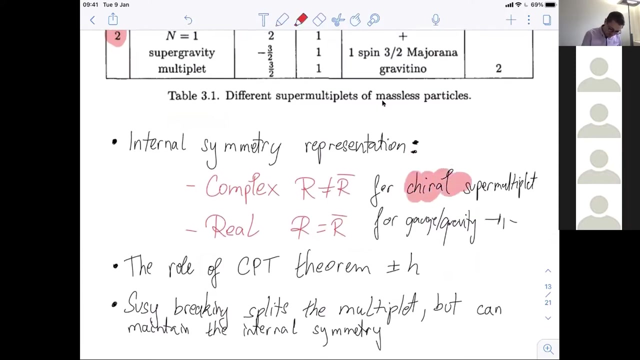 and two degrees of freedom for the fermionic part. okay, so the, the chiral supermultiplat and gauge supermultiplat are very important for MSSM. I won't talk much about supergravity multiplat, so the, so some important points- is that the chiral supermultiplat, 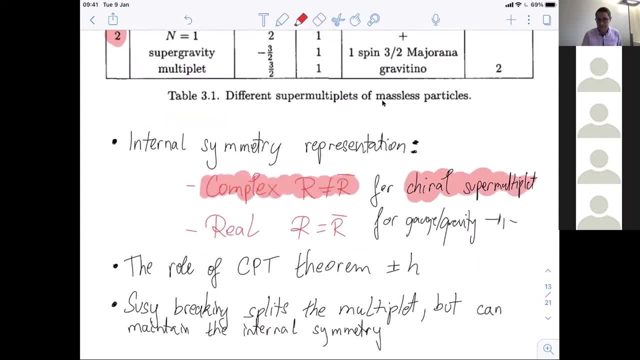 it is a complex representation of the internal symmetries, like gauge symmetry, while the The gauge supermultiplat is a real representation When supersymmetry breaks. so we haven't observed electron superpartner to have the mass of 0.5 MeV. 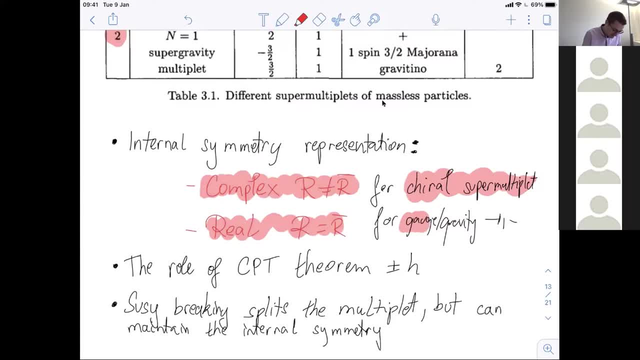 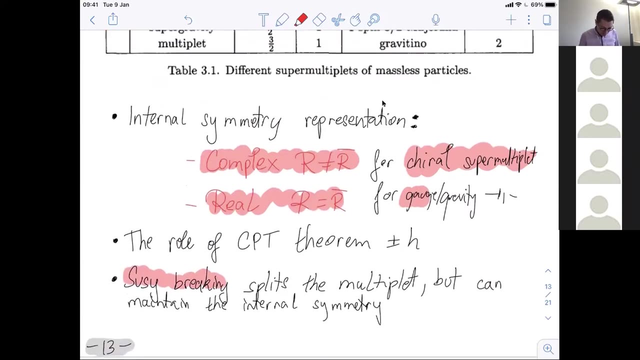 We haven't seen any superpartner at the moment. So supersymmetry is clearly broken in nature And therefore when you break supersymmetry you split the multiplat. So some states are heavier, some are lighter, But you don't have to break the internal symmetry. 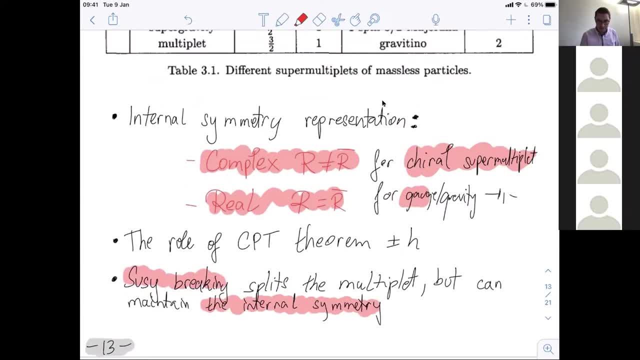 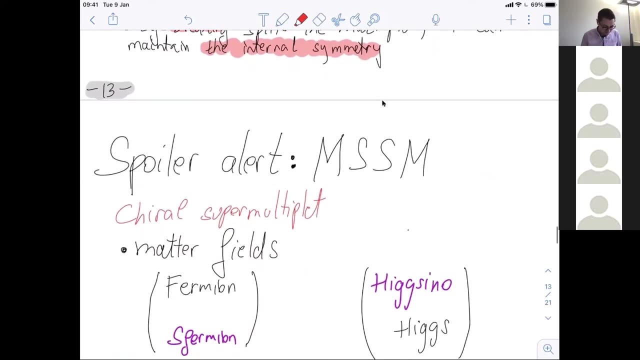 So supersymmetry breaking will split into supermultiplat in terms of mass, but will not necessarily break the internal symmetry. Okay, The gauge symmetry within a multiplat, for example, stays the same, Okay, Okay, I will show this slide. 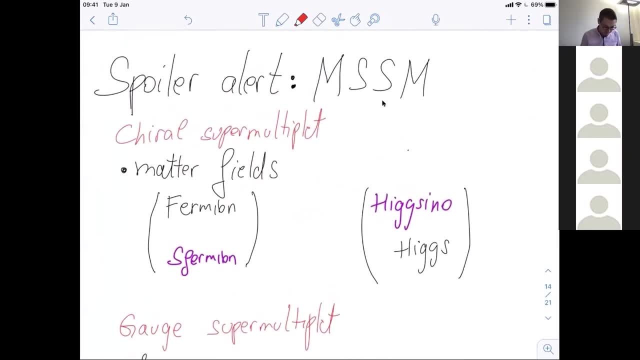 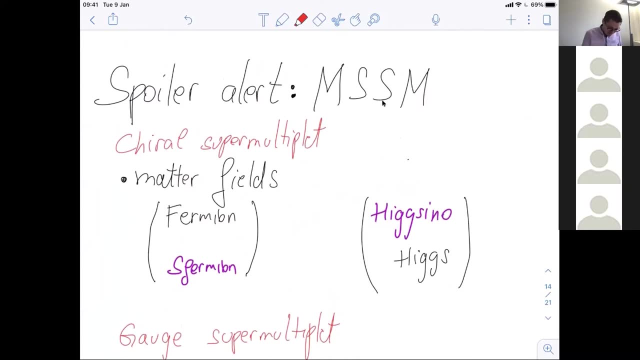 and perhaps we can have a a short break after this. So in the MSSM matter, fields being quarks and leptons, they fit into a chiral supermultiplat, So the fermion of the standard, you know, fermionic matter. 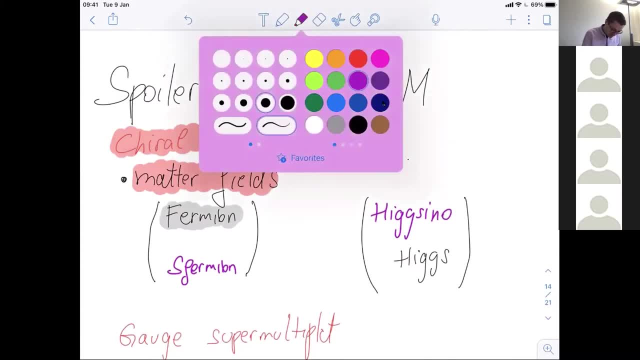 there will be an additional states super, which supersymmetry introduces the so-called superpartner which we call fermion, Okay, And they will be scalars. So this will be spin zero scalar. Also, the Higgs is in chiral supermultiplat. 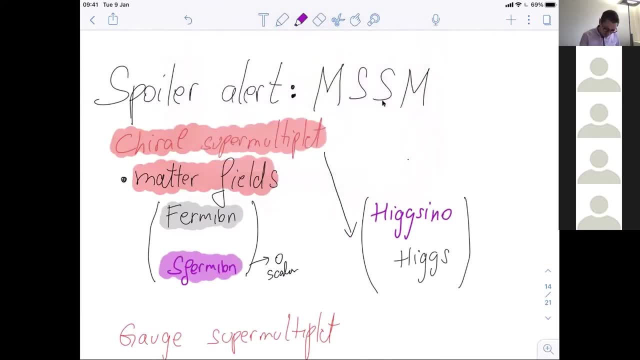 There will be a partner of the Higgs, which we call Higgsino, And the Higgsino will be a fermion. It will be one half spin. Okay, Higgsino will be a fermion. Fermion is a scalar and Higgsino is a fermion. 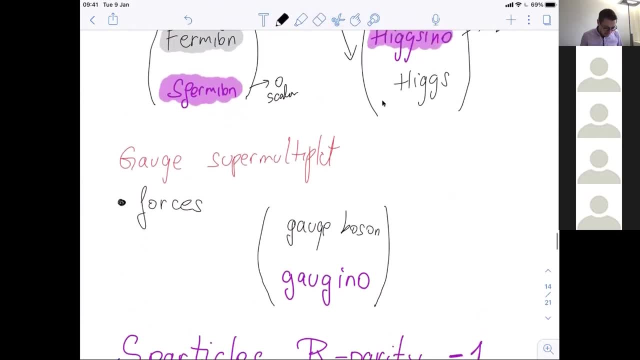 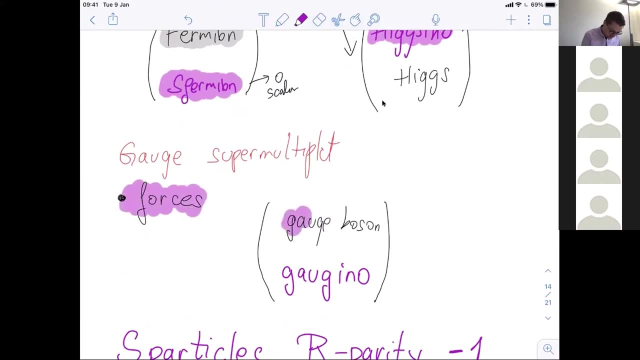 And they sit in the chiral supermultiplat And then there is a gauge supermultiplat which describes forces. So the gauge bosons they are spin one. Their partner will be gauge Gino. Gage Gino is spin one half. 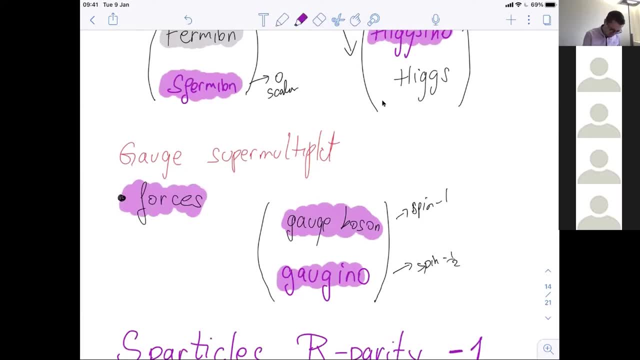 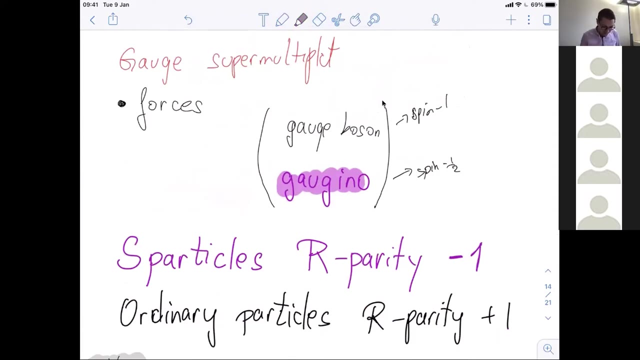 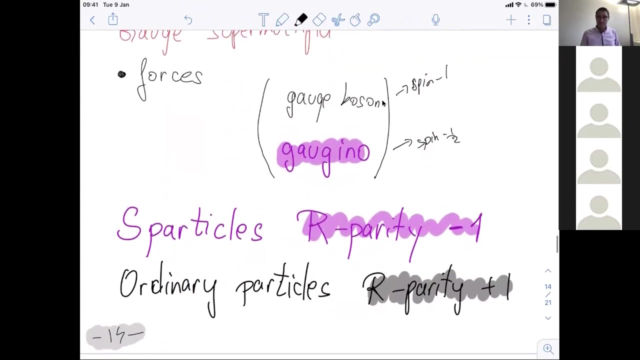 Okay. Okay, That's basically how it works in the MSSM. And then, finally, these particles: supersymmetry electric partners: they have r parity minus one, And ordinary particles: they have r parity plus one. Okay, Any questions? 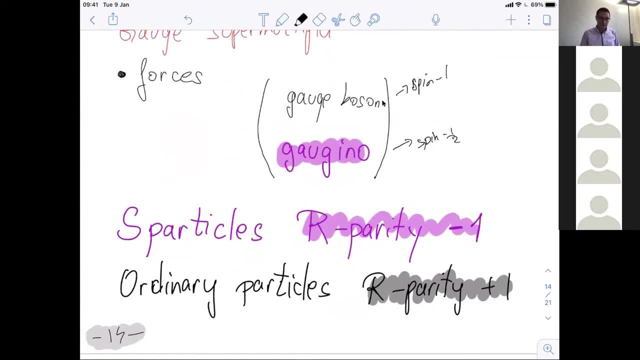 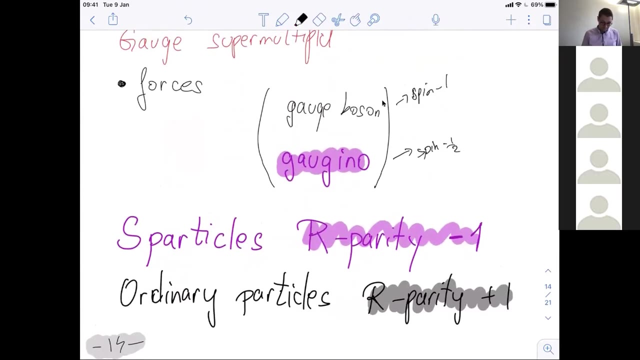 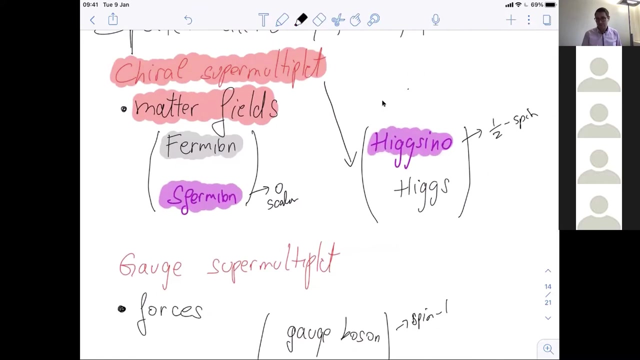 And yeah, Before we close the first class, Sorry, you go first, Mm-hmm. So just about this r parity. how do we know that ordinary particles must have r parity plus one and s particles minus one? So you have to define what precisely this discrete Z2? 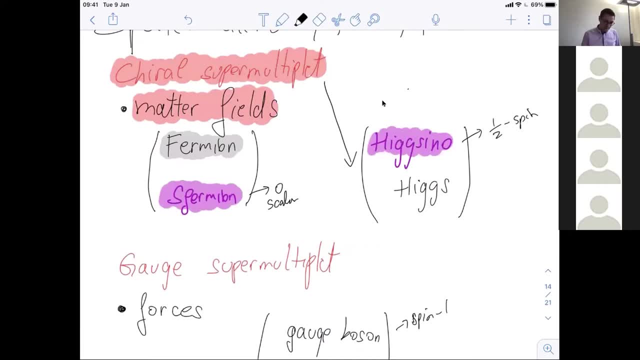 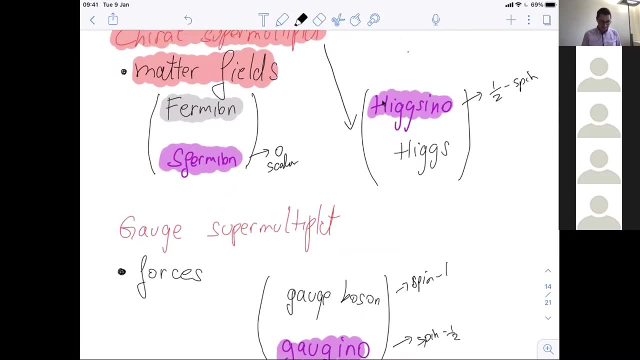 of the original U1R is, And then you have to give to these guys the. I mean then you have to give to these different chiral supermultiplates this r number And then turns out there is a choice in such a way: 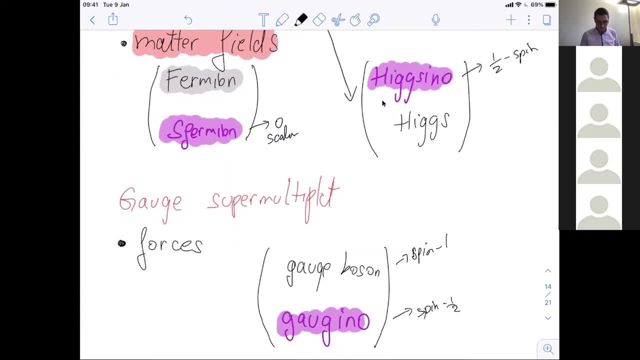 that the super particles are odd and that this one is even. Oh, okay, okay, So it will. yeah, This actually is a rather trivial to show when you start from the algebra: Oh, okay, okay, Okay, thank you. 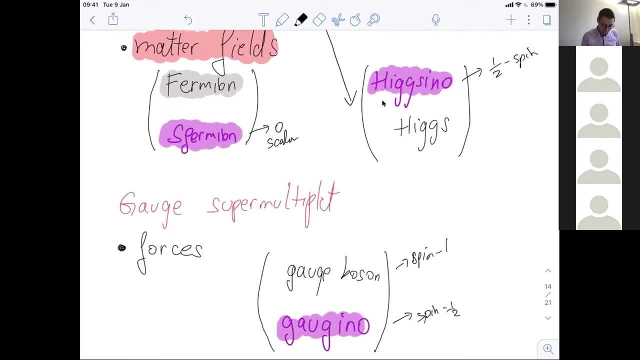 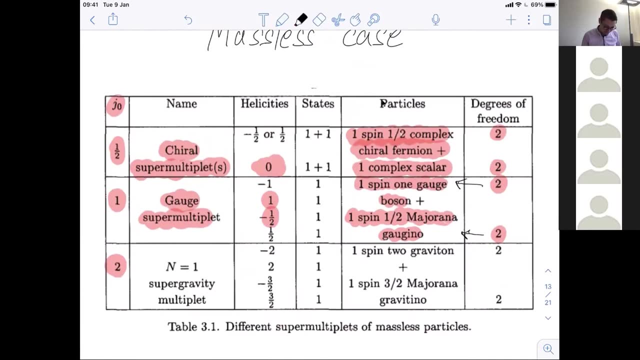 I would have a question about the massless, the massless particles that you showed before The massless supermultiplate. okay, Yes, exactly, So there are three possibilities for J zero. So can all of these be? can J zero be all of these three cases? 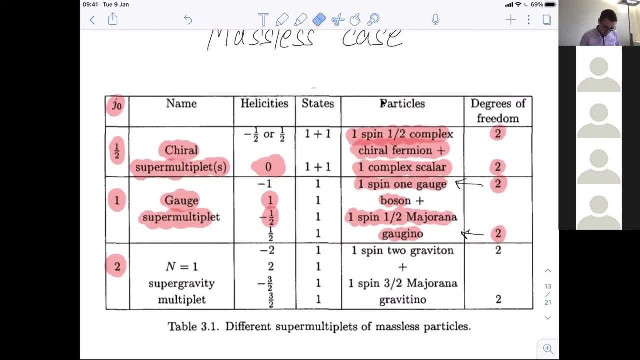 So can it be in total 12 massless particles, or does one have to choose one of these possibilities? So these are different irreducible representations, They are different entities. So for example, for example in the MSSM, in the MSSM you put a gluon. 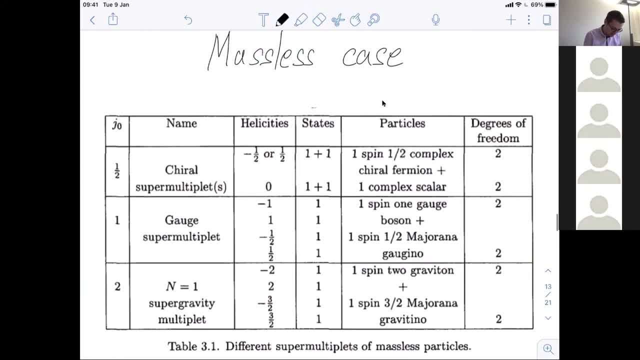 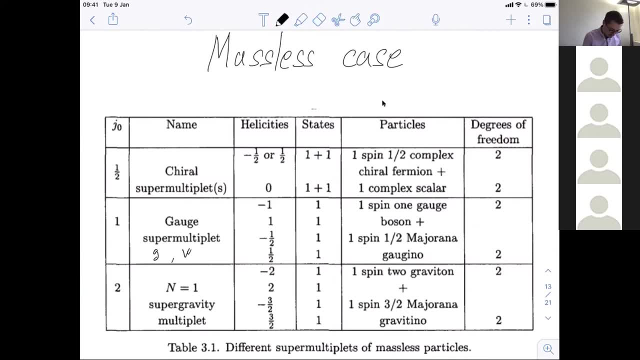 Gluon will be. gluon will be one gauge supermultiplate. The other one would be would be, let's say, WA, the, the, the, the, the, the, sorry, the gauge bosons of the SU2 and the B. 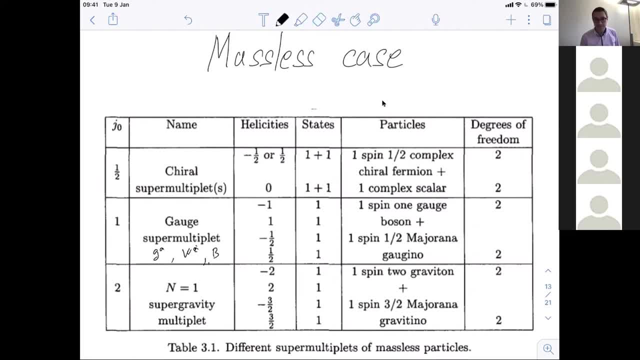 the gauge bosons of U1.. This will be three different gauge supermultiplates. Like in the standard model, you have a gluon field, you have a W field, you have a B field. So now you will have a gluon G supermulti. 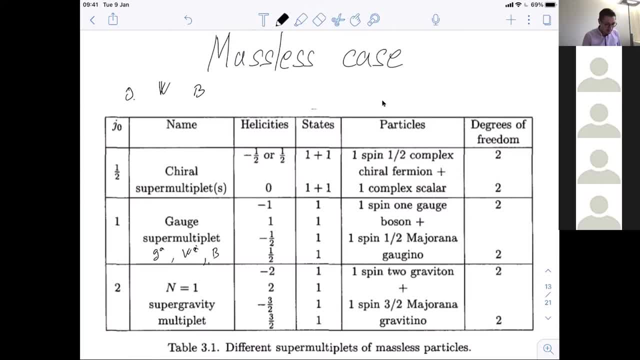 gauge: supermultiplate- W gauge, supermulti- B gauge. Regarding the, the, the chiral supermultiplates, all the fermions Q, U, D, E, L. they are different chiral supermultiplates. Furthermore, they the chiral supermultiplates. 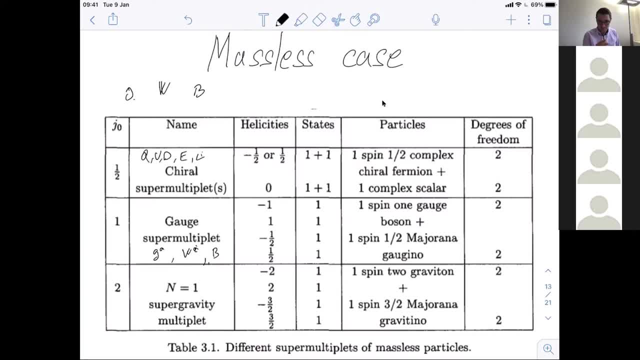 they click, they carry flavor index. I goes from one to three which are separate chiral supermultiplates. Okay, I think I understand. Okay, All right. So let's make a very short break, All right. So that was the discussion of the particle supermultiplate. 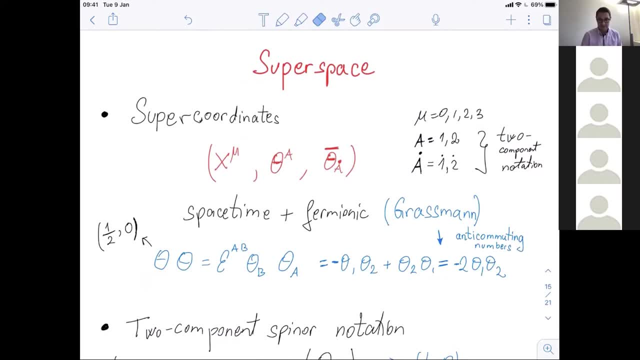 but we want to eventually do quantum field theory, So we want to talk about fields and write down Lagrangian and, yeah, formulate the theory in this way. There's the concept of super space. We enlarge the, the space sort of the Super Algebra. 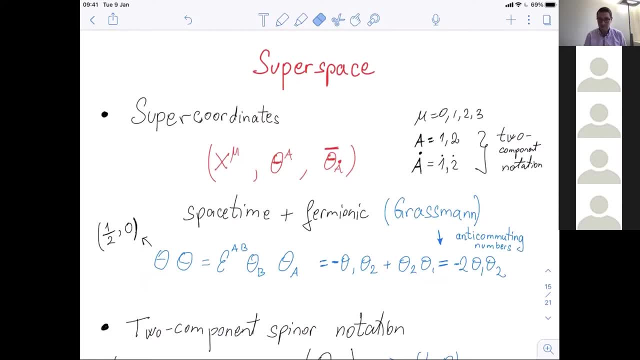 the not trivial way to combine more general space, time, space, and I mean internal symmetry, so We can introduce the concept which is called the super space. So the superspace, super space will enlarge the space-time and there will be super coordinates and the super coordinates. 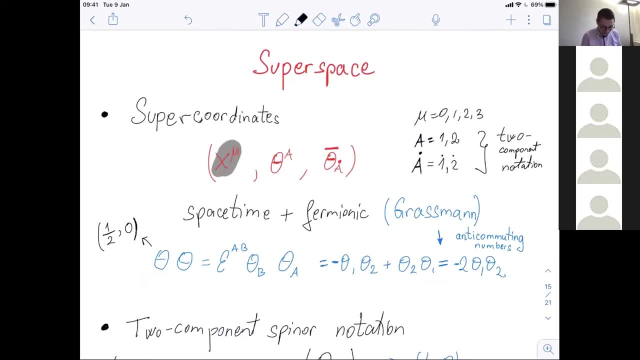 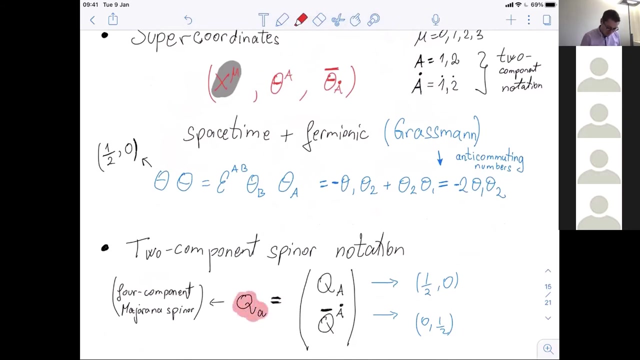 will have the usual coordinates, usual space-time coordinates, and it will have, in addition, the fermionic coordinates. these are a grassman numbers. okay, this theta a and a dot um, here i will. i will switch to the so-called two component spinner notation. remember that my super charge was a four component Majorana spinner, but in fact it is only this. 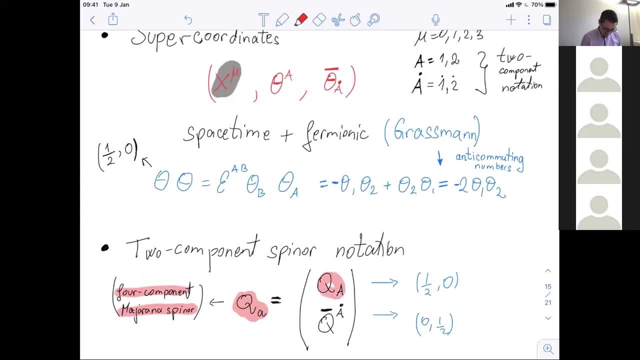 yeah, these two component wild spinners, where this dotted index a and a dotted, i use these dotted and undotted indices. so this theta, i can do products of these thetas which is Lorentz invariant, for example, this product here, theta square, uh, remember. so this theta is the? is this the? the vial representation? 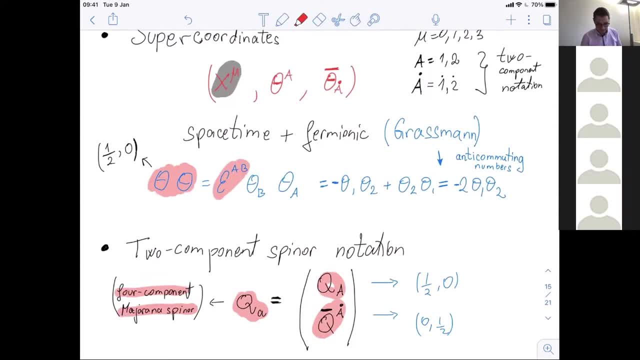 so remember that you can use Levy-Civita epsilon to, to, to, to write down Lorentz invariant quantity. so this is a. this is one of those. and, in particular, note that for ordinary numbers this would be zero. right, if these were ordinary numbers, this thing would be zero, but here it's not the case. okay, um, because these are anti-commuting. 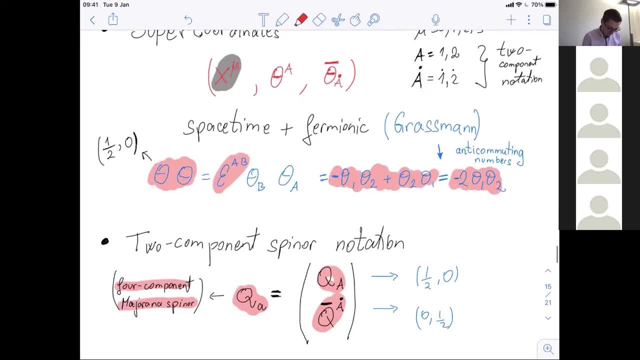 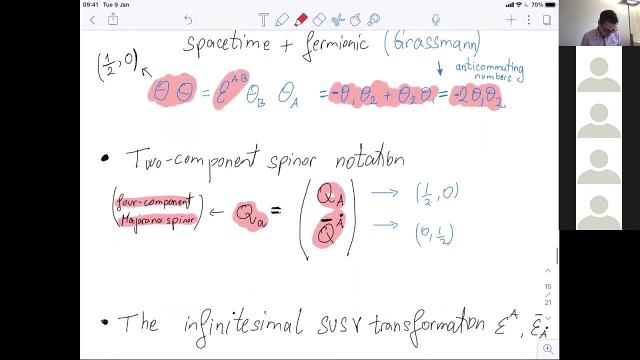 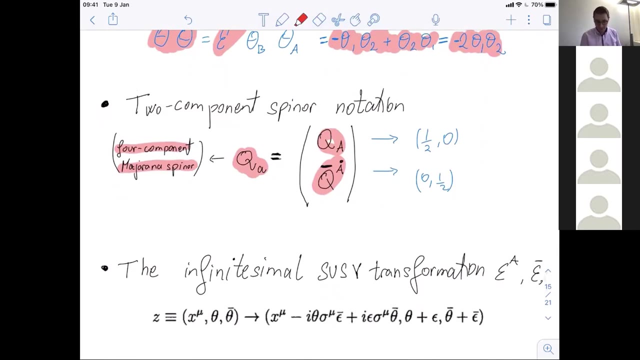 numbers. okay, okay, so these are super coordinates in super space. so we can do just like we do the, the, the, the transformation of the coordinates- space-time coordinates- under point caret symmetry. we can do the transformation of the super coordinates under supersymmetry. so this is a: these are super coordinates and you perform a supersymmetry. 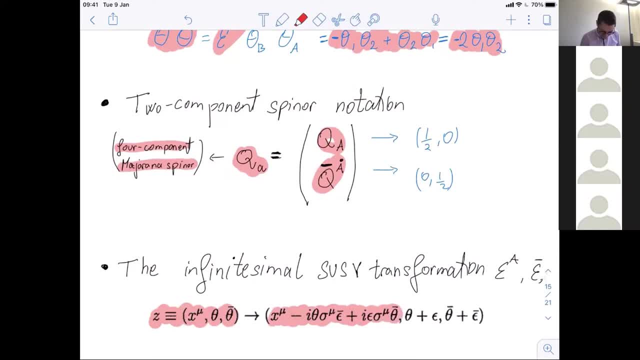 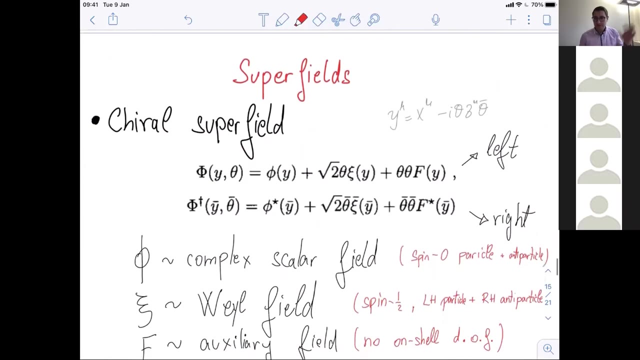 this is how the first component changes. second and third. so infinite tensimale sousie transformation, epsilon. okay, all right. so now you can. that's, your space has bosonic, the usual coordinates, and fermionic coordinates. now you can do super fields. a super field will be a function of super space coordinates. and one important thing: 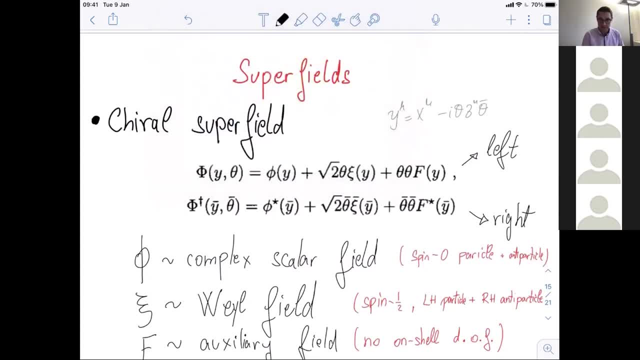 before I start discussing different types of super fields, is that so a super field? it depends on the, on the super coordinates. is that you can sort of expand the, this field, the most general super field, you can expand, you can tailor, expand in the, in this Grassmann or Fermionic coordinates. 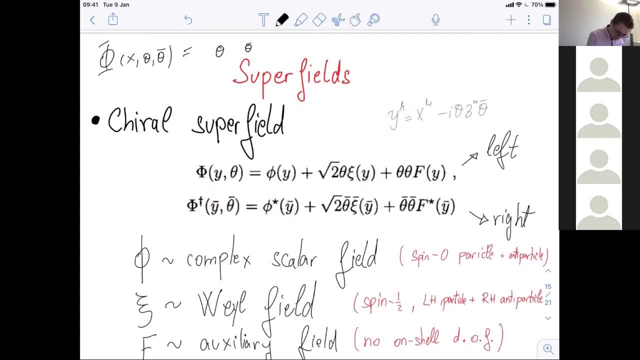 and the reason being that that expansion will be finite, you will have only a finite number of terms. so, for example, take theta 1. theta 1 square will be zero because theta. so I choose a specific component of the, of the, of the theta: theta 1. 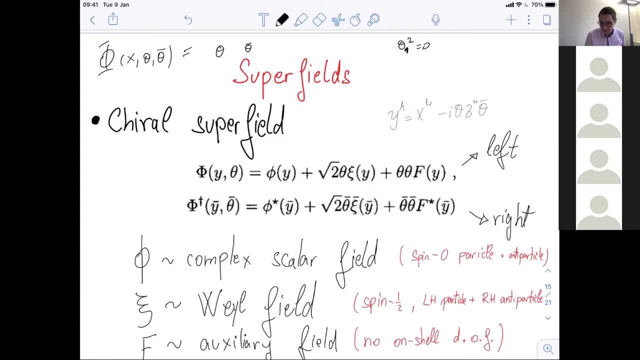 so I choose a specific component of the of the theta theta 1. so I choose a specific component of the of the of the theta theta 1. So since it's a Grassmann number, it's squared is zero because it's an anti-commuting number. 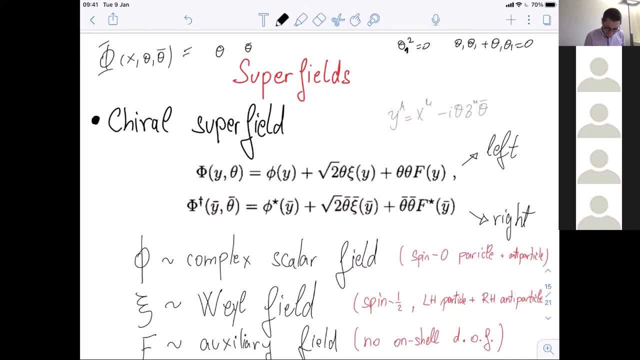 So we are going back to the definition. So when you do this expansion, there will be terms. there will be some number of terms, but it will be a finite number, not too many. We'll have this finite number of terms and those terms will be just. 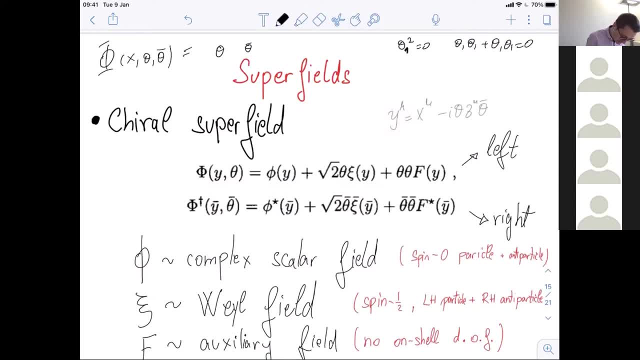 so the coefficients which multiply those terms will be just a function of space-time, which means those coefficients in the expansion in theta and teta bar will be ordinary fields, functions of ordinary coordinates, space-time coordinates. So that is about, so the most general super field. 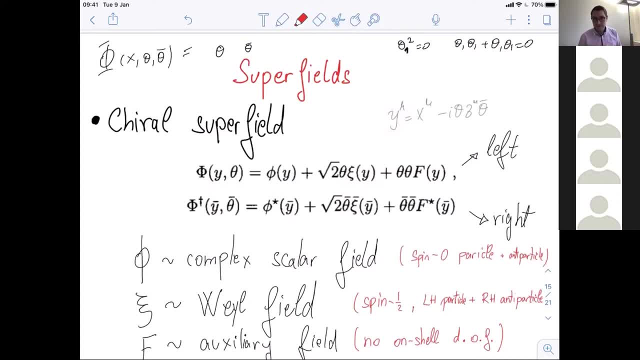 Now, if you multiply two super fields, you will get a super field again, because the super field is the one which is the general function of the super field. Because you know again, you have this expansion in the Taylor, expansion in the Grassmann coordinates. 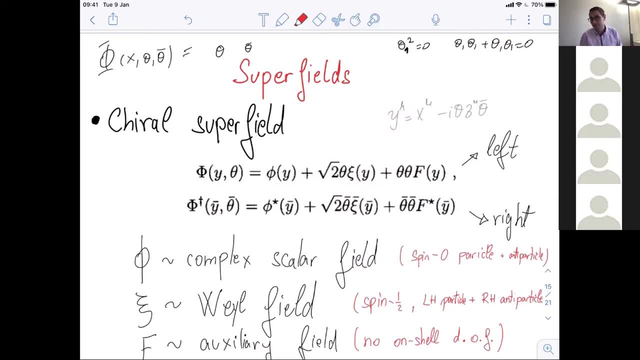 So it will. any function has to have that form. even the product of the two functions will have that form. So it's a general. the general function will cause super field. Now there are irreducible representations, meaning under supersymmetry, of course. 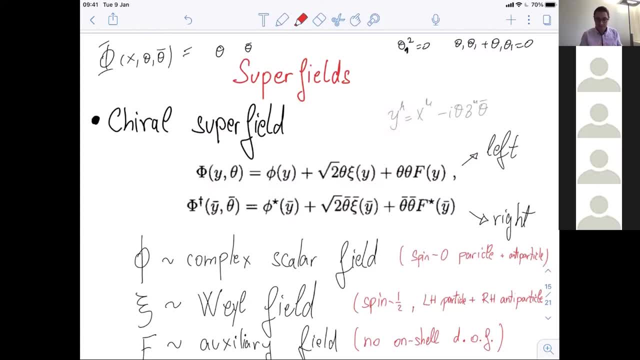 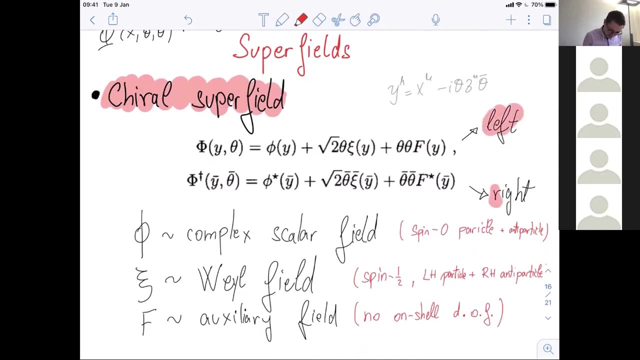 meaning a subset of these general functions of coordinates. One irreducible representation is the chiral super field. It has a very specific form, which is this one. So this is a left chiral super field and the right chiral super field. okay, 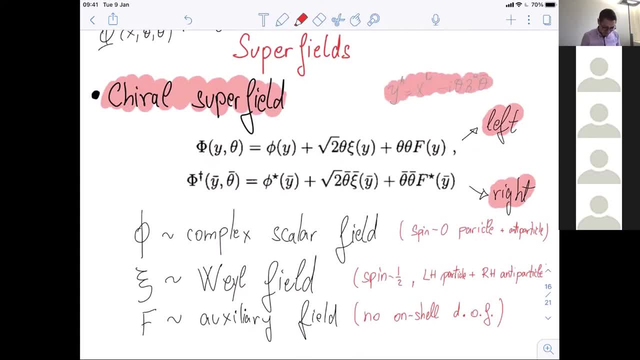 This Y is given by this formula here. So what does it have? So what does it have? So what does it have? So it is only. it only has these two terms: linear in theta and theta, square and no theta, So it only has these terms. the left chiral super field. 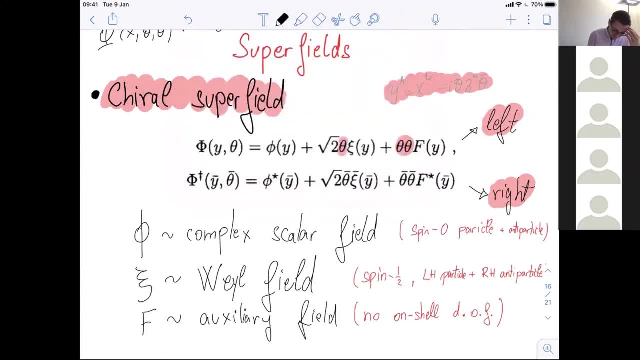 Okay, For example, it doesn't have a term which is theta, theta, theta bar, theta bar. This is a perfectly legitimate term, but it's not there in the chiral, in the chiral super field Now. so what are the coefficients of these terms? 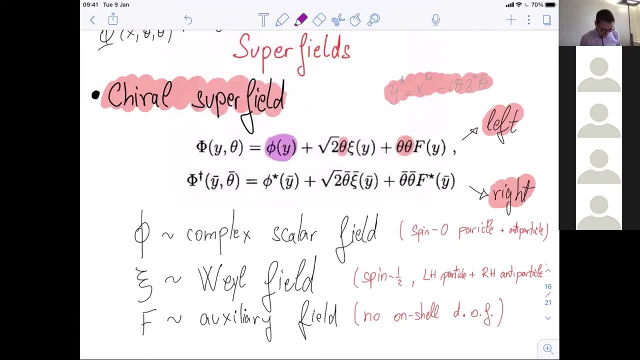 So this thing here is a complex scalar field. Phi is a complex scalar field, So it's a spin, zero, particle and antiparticle. This guy here is a fermion, Why? Because theta, theta is fermion and you need to have a Lorentz scalar. 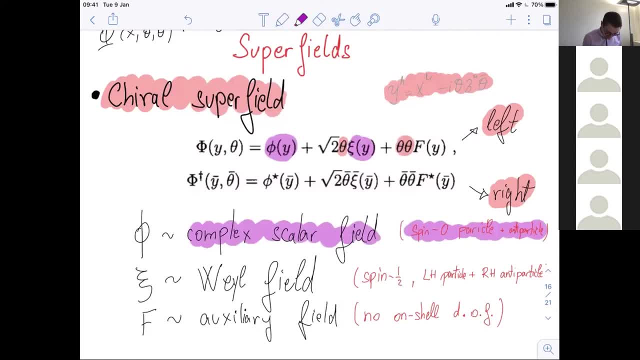 So this psi is a fermion, So it's also a field, So it's a wild field. What does it mean? So it's a spin one half, and then it has a left-handed particle and the right-handed antiparticle. 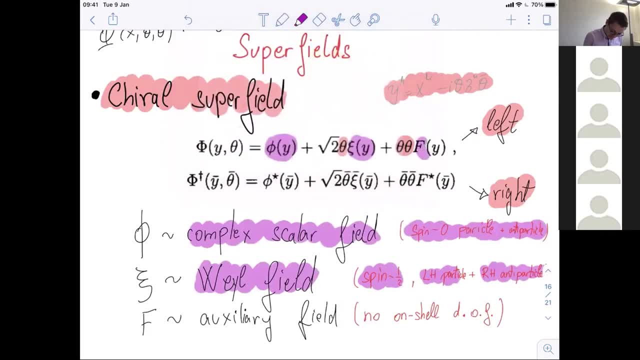 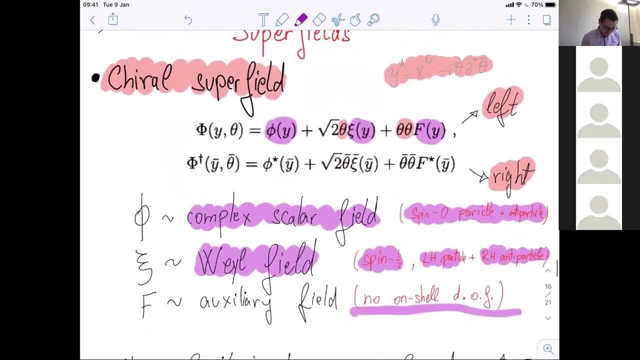 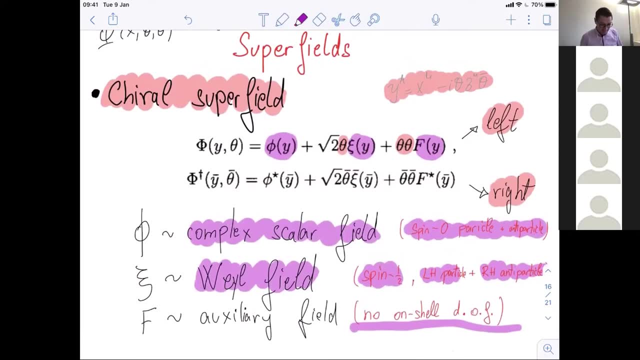 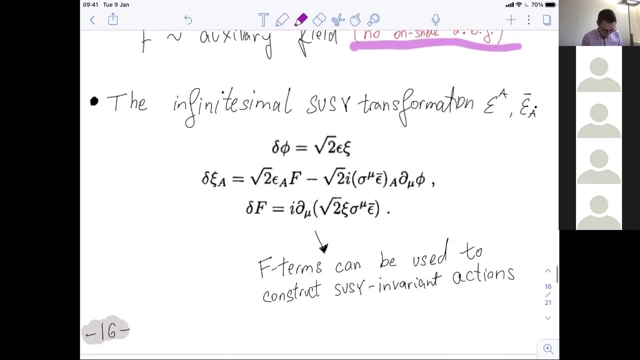 meaning it doesn't have onshore degrees of freedom. Okay, So chiral supermultiplet that we introduced before. So chiral supermultiplet that we introduced before is actually related to the chiral super field. Now you can do the Susi transformation on the chiral superfield. 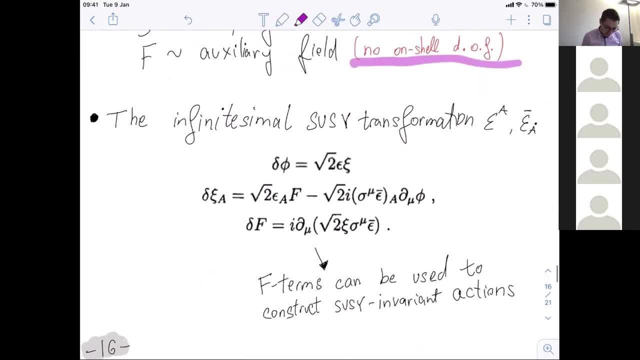 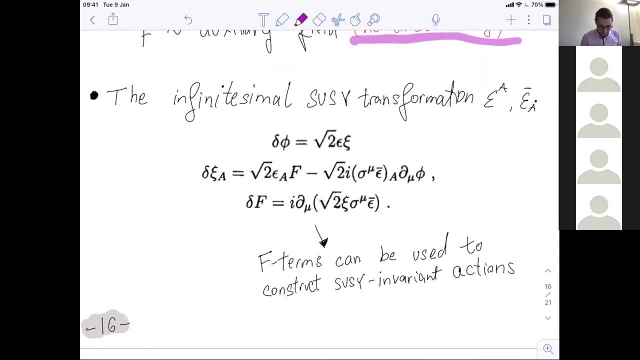 Now you can do the Susi transformation on the chiral superfield. Now you can do the Susi transformation on the chiral superfield And this is how each component individually transforms. This is a very important point here. The F-term okay. 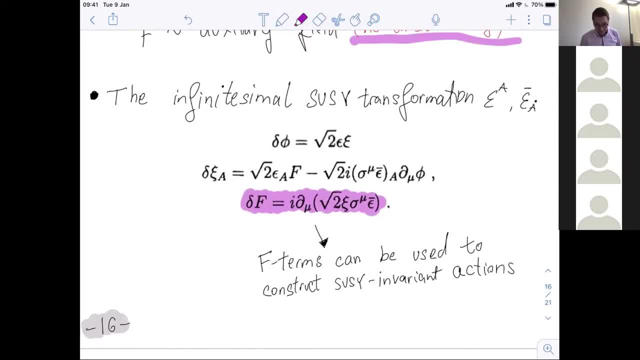 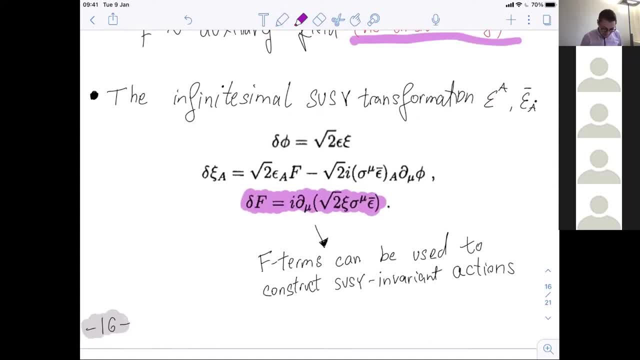 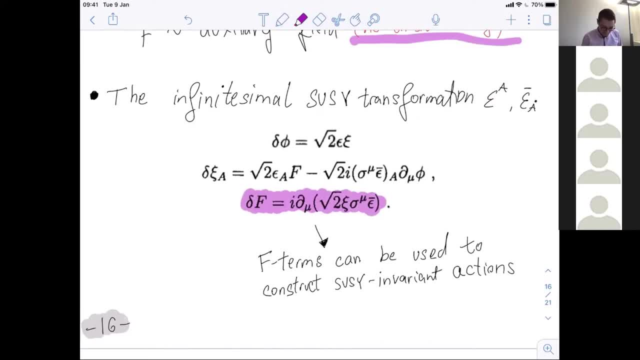 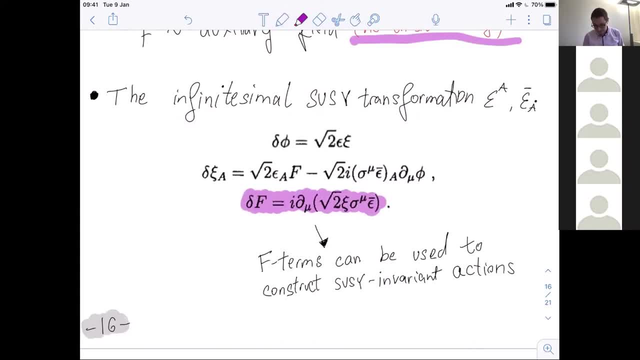 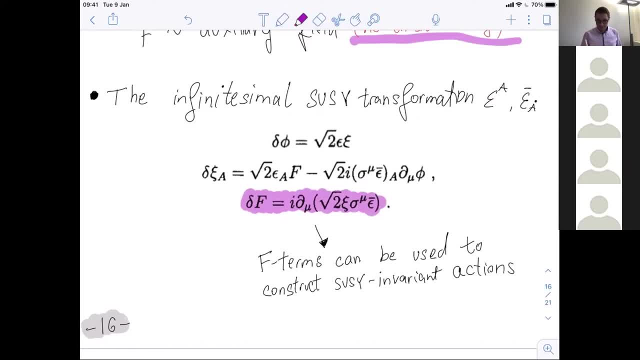 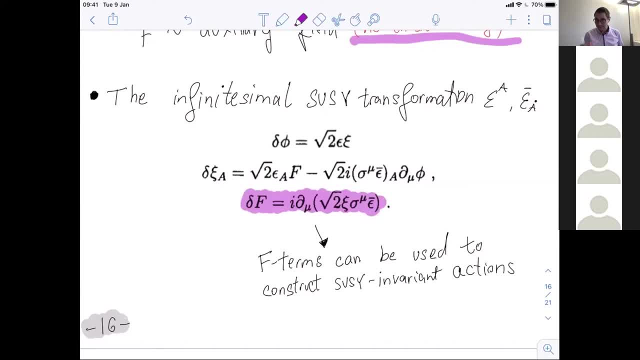 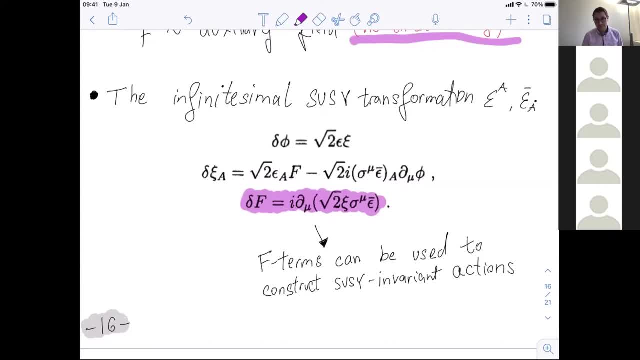 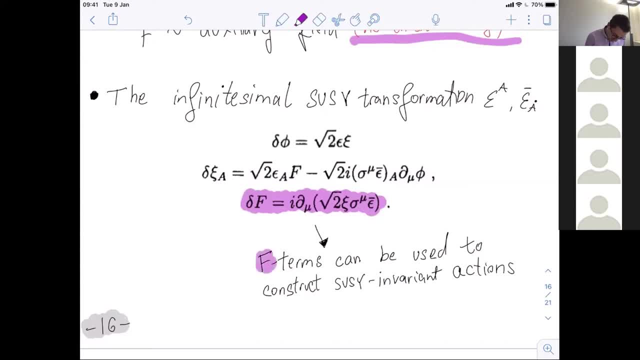 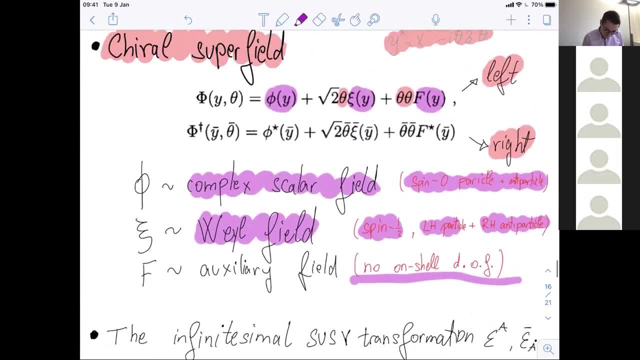 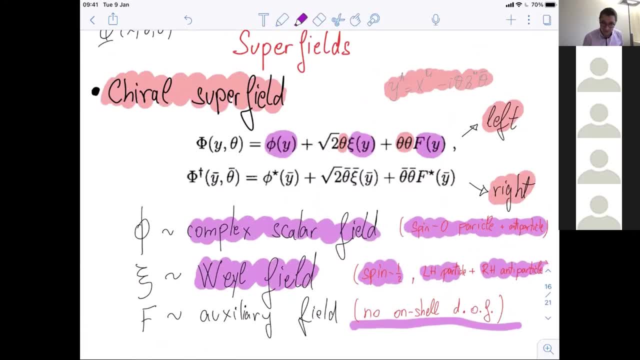 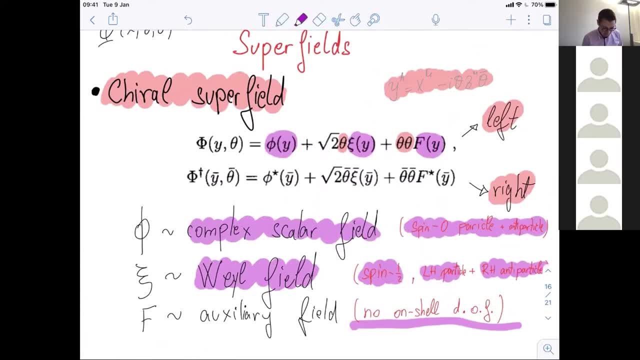 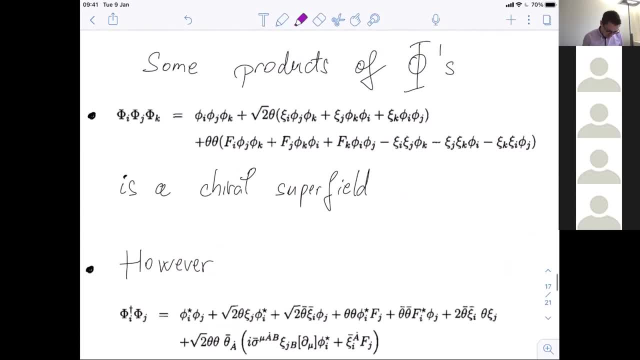 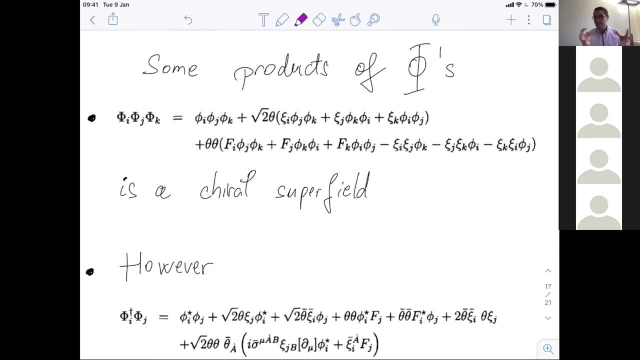 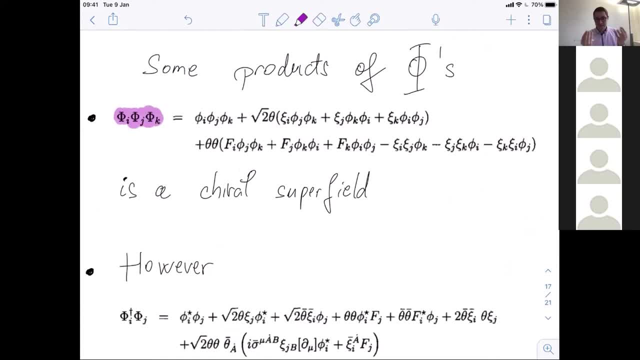 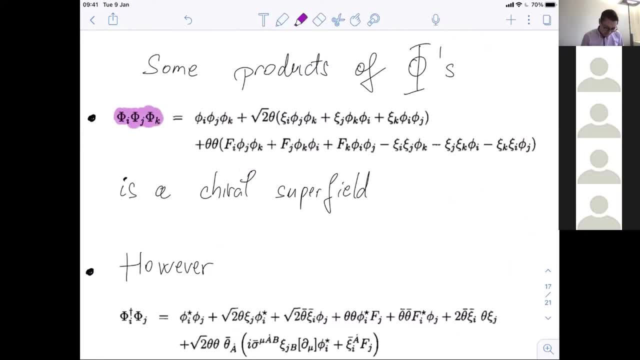 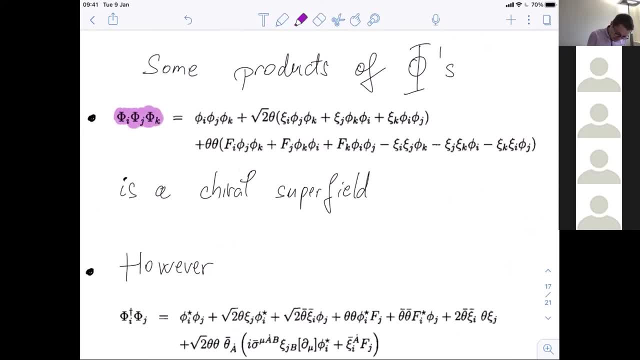 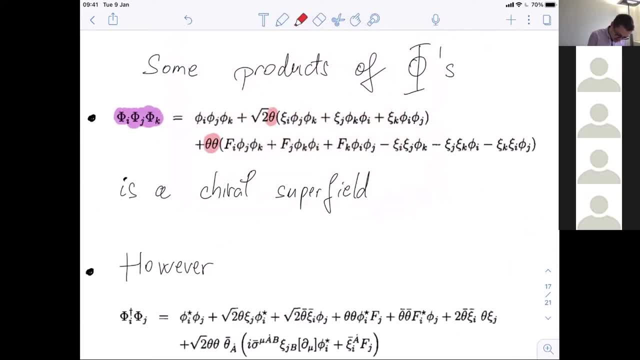 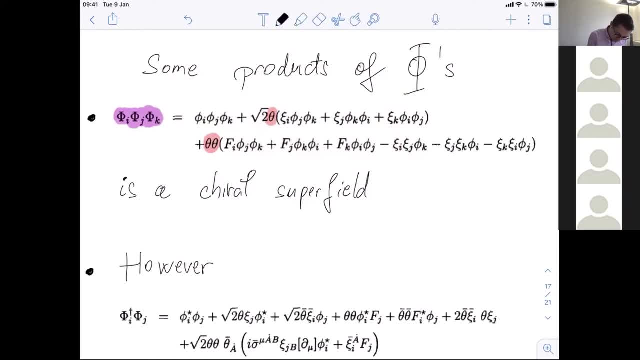 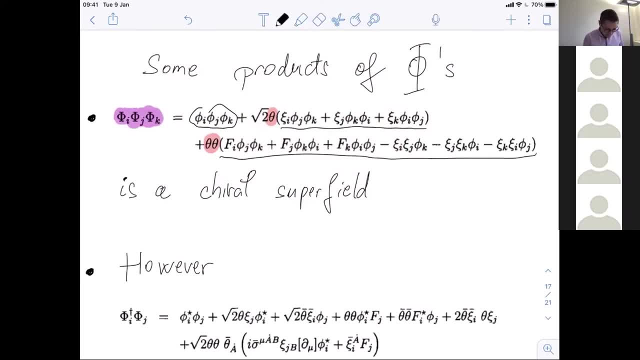 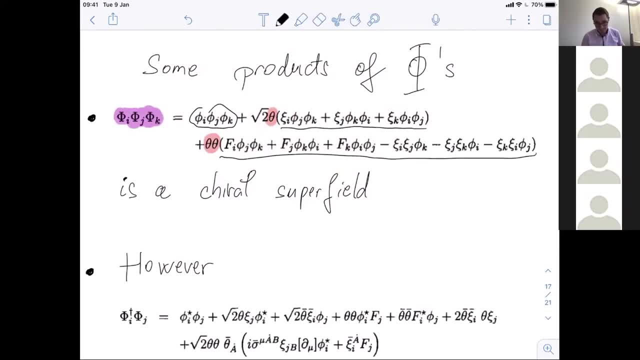 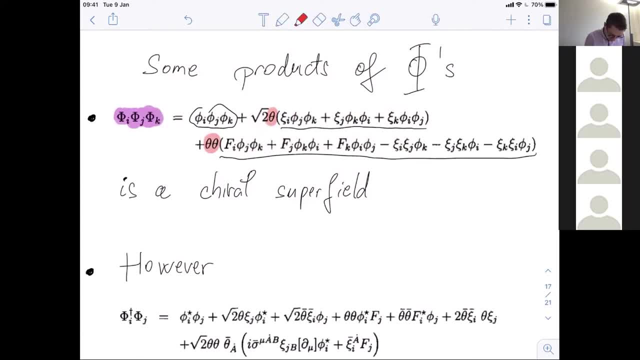 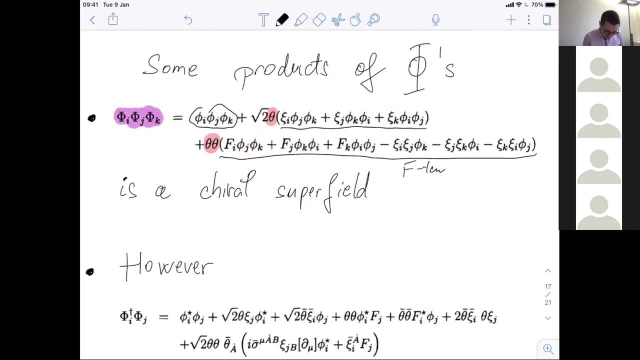 Because we know if Susi invariant action, Because we know if Susi invariant action, Because we know if Susi invariant action. for example, Yukawa interactions. These are Yukawa interactions. Remember, xi is a fermion and this xi is another fermion and this is a scalar. So we have fermion-fermion scalar, This. 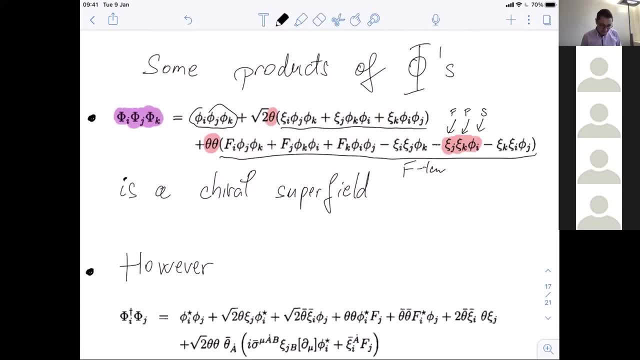 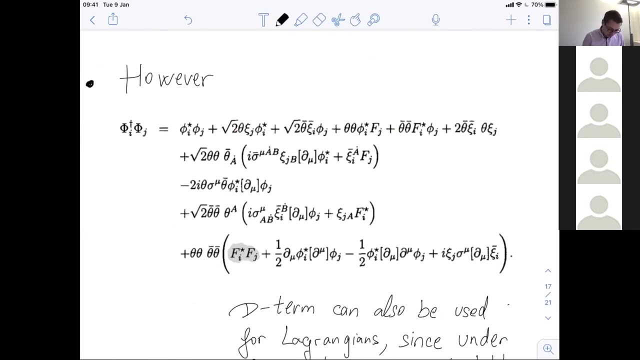 is a Yukawa interaction, for instance. So you can take the F term meaning the coefficient of this theta square piece of this triple product of chiral superfields, to be your term in Lagrangian, It's Suzy invariant. However, the product of this combination of F, dagger F or phi, dagger phi. 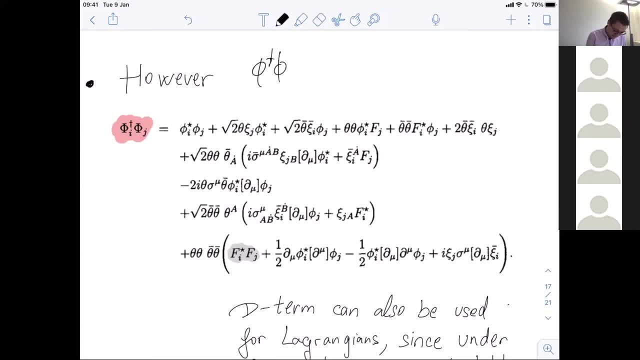 the conjugate one: phi dagger. phi Dagger is the Hermitian conjugate. This is not a chiral superfield. So look, this is Remember. chiral superfield would have this term. It would have this term. It would have- Where is the F term? It would have this term. This would be a left. 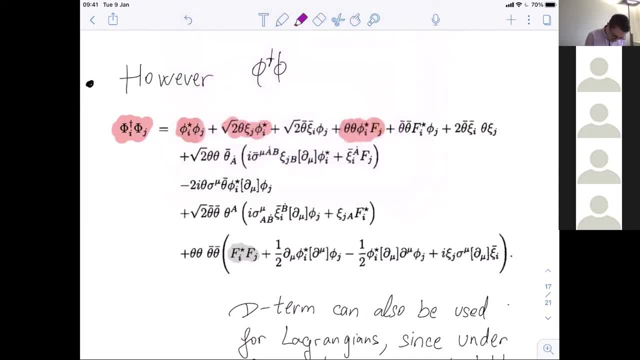 chiral superfield. okay, This term and this term would be in the right chiral superfield. But then there are. You see, there are other terms which, Yeah, there are other terms. For example, there is this term which has theta square. 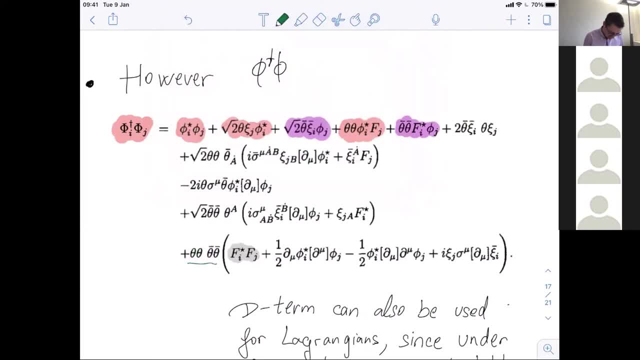 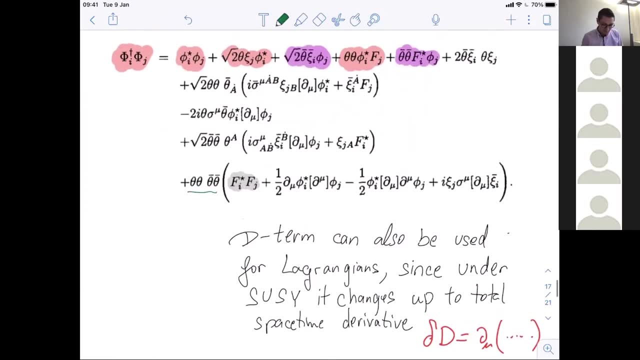 which is theta square, theta bar square. This is called the D term And in fact now you can do the Suzy transformation of the general. This, I guess, is the general superfield, the general function of the super, Of the coordinates. 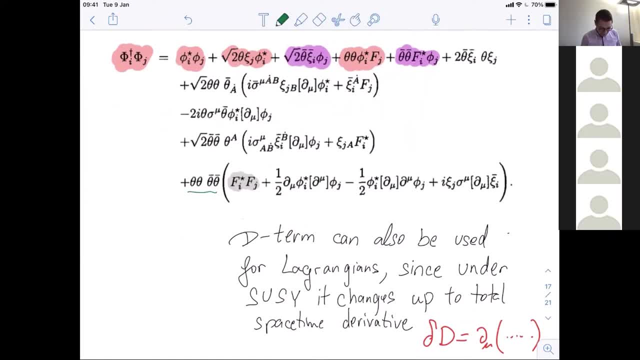 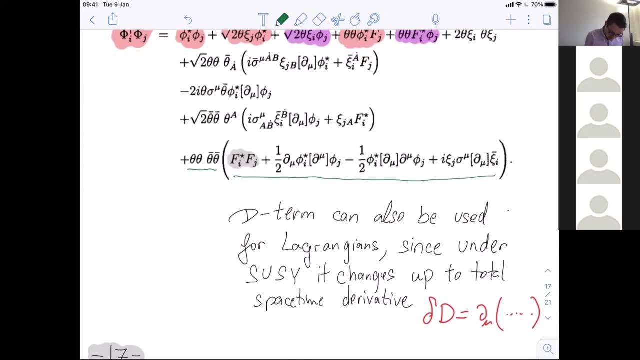 And when you do the transformation of the, The Suzy transformation, then you can show that this term, the D term, the D term, which is the coefficient in front of theta square, theta bar square, that one changes up to a total derivative. Under supersymmetry, it changes up to a total derivative. 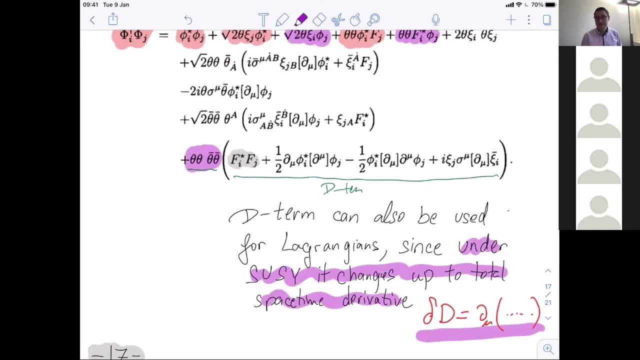 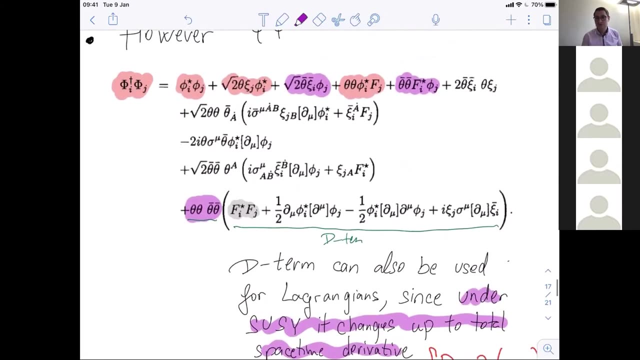 which is this formula here, Meaning that you can also use a D term. You can use a D term to construct Suzy invariant actions or Lagrangians To construct Lagrangians which lead to Suzy invariant actions. So this D term and F term is something which is used to write down the theory. 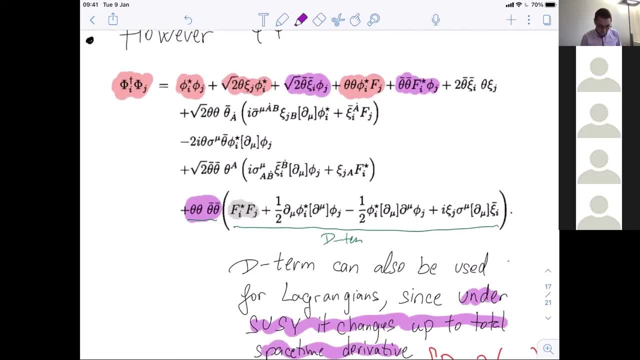 F terms are usually called the superpotential, And this D term, this one in particular, is the Kähler potential, And this D term, this one in particular, is the Kähler potential. It's just some terminology, Notice. in the D term we have the 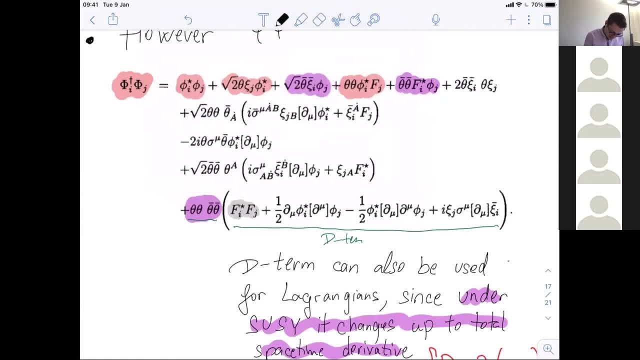 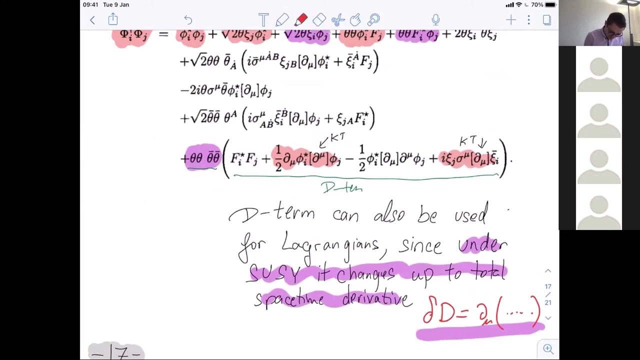 For the Kähler supermultiplet. we have the kinetic term for the scalar field and the kinetic term for the fermionic field for the Weyl fermion. So notice that in this piece we don't have a kinetic term for F. 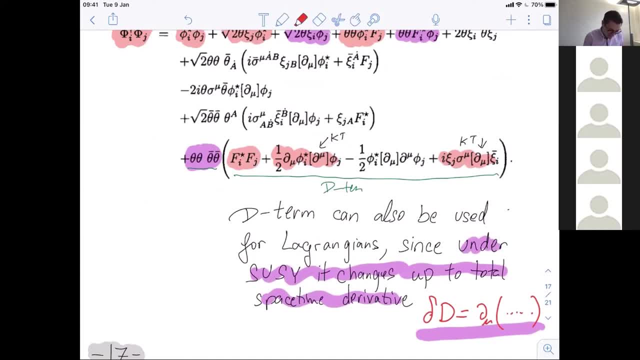 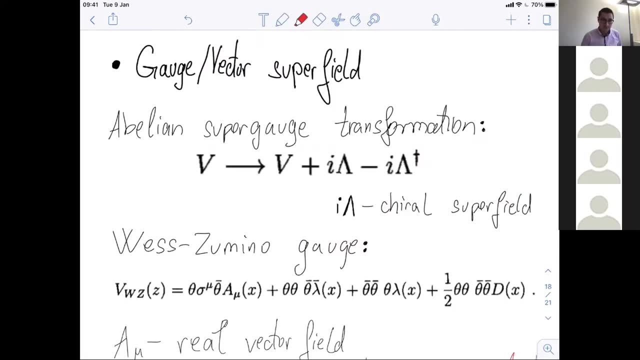 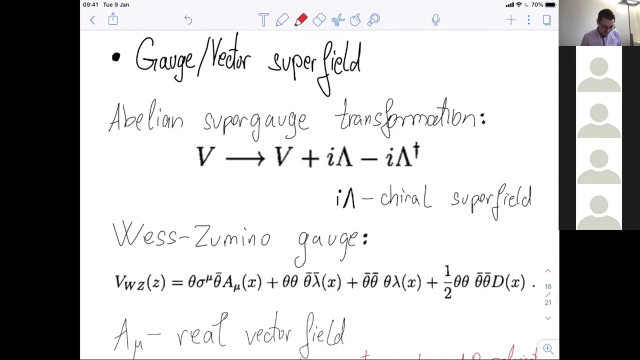 So the F, that scalar F, is the auxiliary field because it doesn't have a kinetic term, It's not propagating. Okay, If no questions, I will go through the gauge or vector superfield. So for the gauge and vector superfield we have a reality condition. 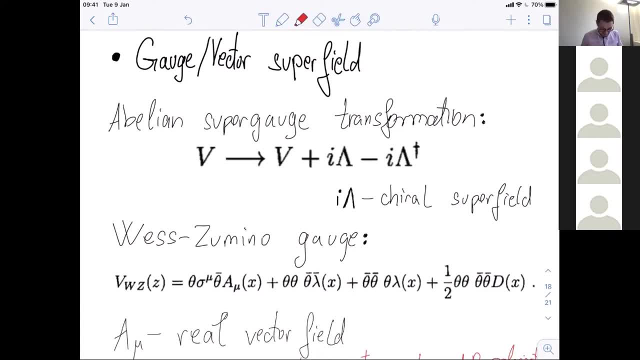 So the field is real, superfield, there is a reality condition which defines it And, in particular, there will be a super gauge transformation, a billion super gauge transformation. Remember that the gauge transformation, for the ordinary gauge transformation, you would take a vector field and you would transform it by gauge. 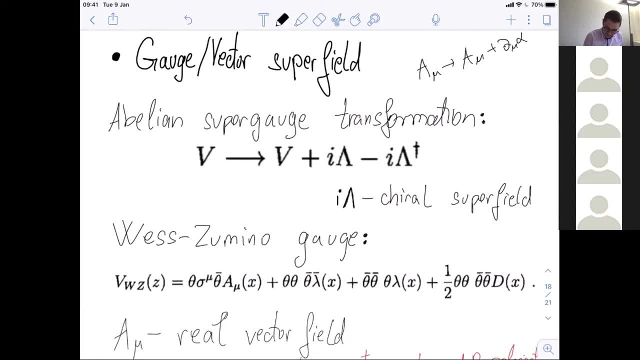 The derivative of some. Okay, So there was a scalar function. So this parameter, alpha, depended on space-time. This means local transformation, So it's a scalar field. So a billion super gauge transformation would be changing the super field by the real part of the chiral superfield. 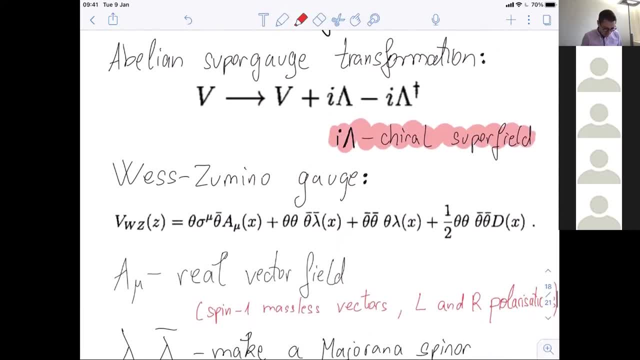 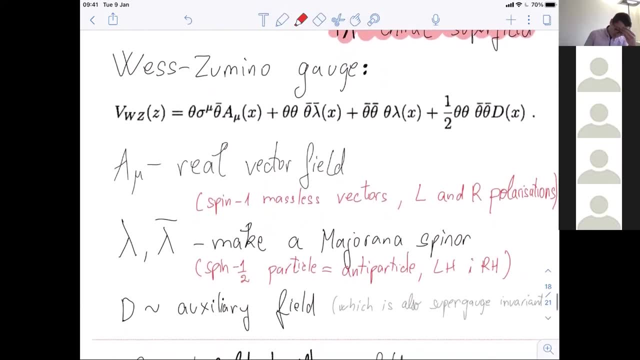 This is a chiral superfield, Okay, So now you can do this gauge transformation and fix and go to a very specific gauge And this is called the Vesumino gauge, for example, And it will have these terms. So again, the components will be: 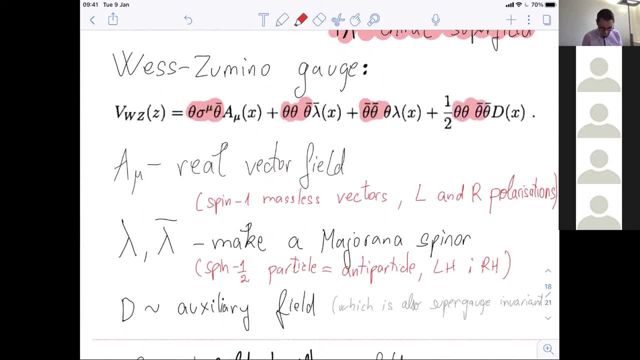 So these are the, So these are the expansion in theta and theta bar And the components will be just ordinary fields. So, for example, this guy here is the real vector field, For example photon. So it's a spin, one massless vector. 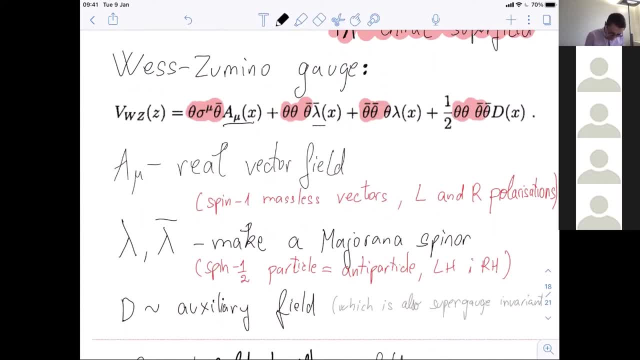 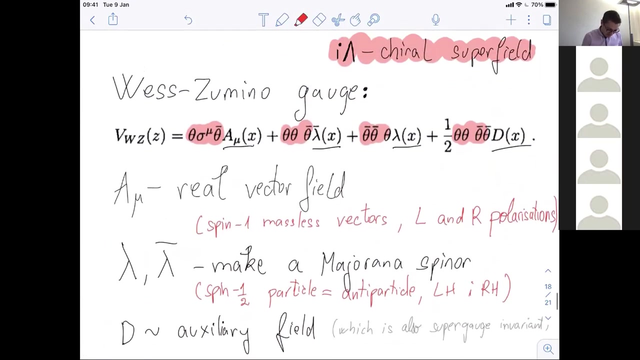 With left and right polarization, And this guy and that guy, they are a Majorana spinner. You have to make a scalar Lorentz, scalar right, And this guy here is some auxiliary field. This D is the auxiliary field, So in the vector supermultiplet, 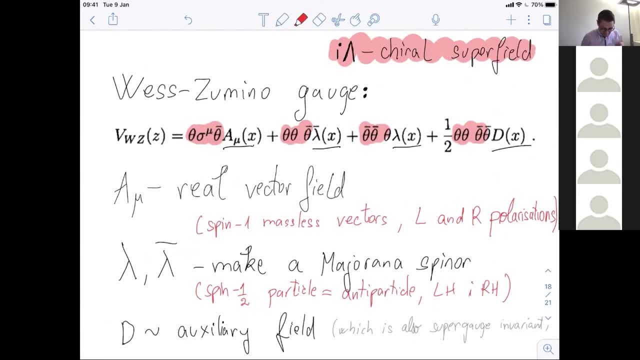 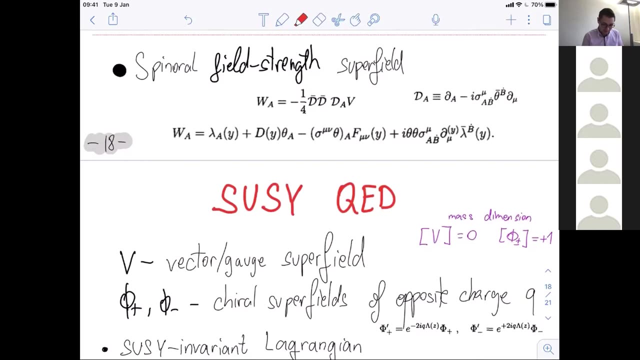 So we have a real vector field and a Majorana field and the auxiliary D field And the vector supermultiplet is related to the. The vector superfield is what gives the vector supermultiplet, Gives rise to vector supermultiplets. One can construct from a vector superfield. 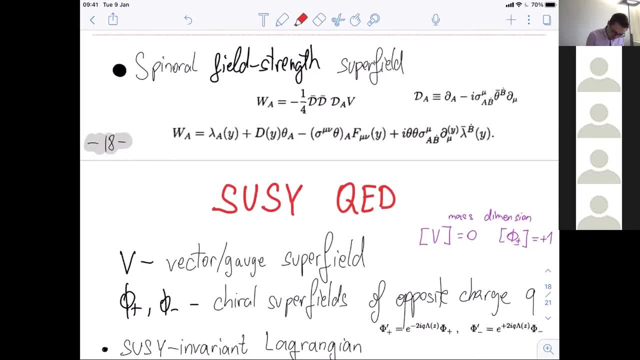 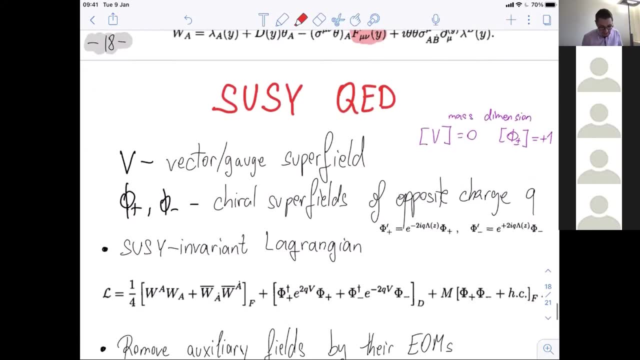 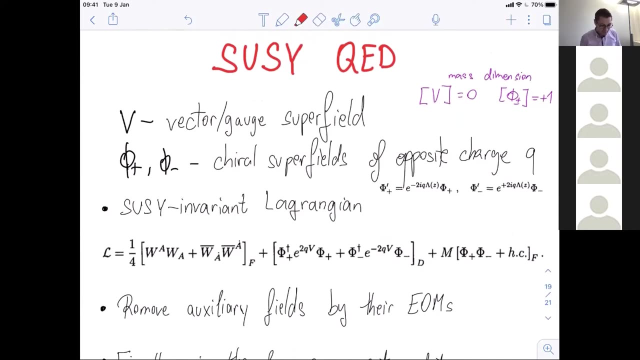 One can construct a field strength superfield which will have the gauge invariant field strength F-Munu. Okay, And with these ingredients we can formulate a supersymmetric version of quantum electrodynamics. So let's see, how would the ASUSI version of QED look like? 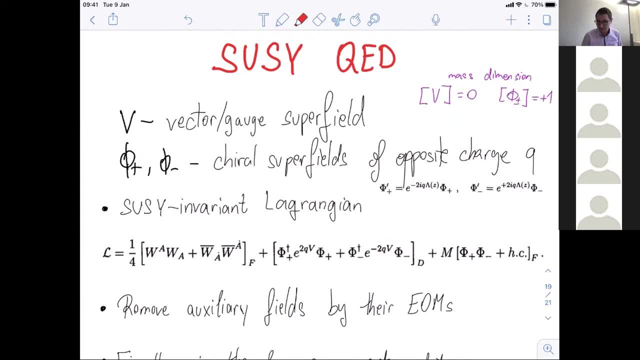 So, to explain the electron field, we know that, first of all, QED is vector-like theory, So we have a left-handed electron and the right-handed electron. Therefore, we need two chiral superfields, This guy and that guy, Which would have both chirality. 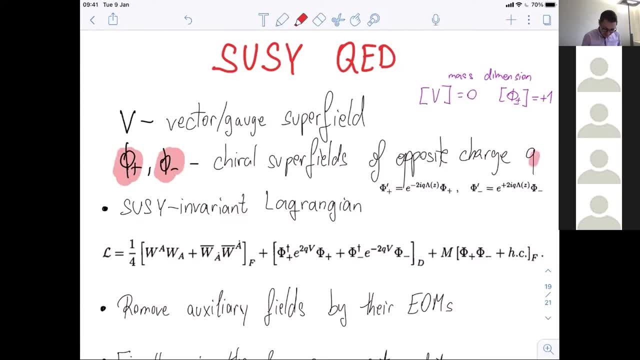 And they would have all the Opposite electric charges. Q- We want to have the gauge anomaly theory. vector-like theory. QED is a vector-like theory, So if you require U1 gauge invariance, you will have to introduce a vector superfield. 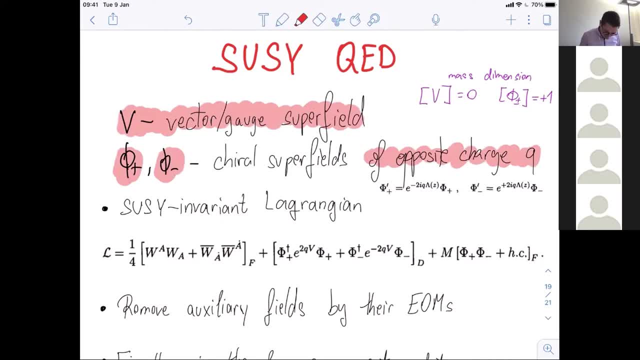 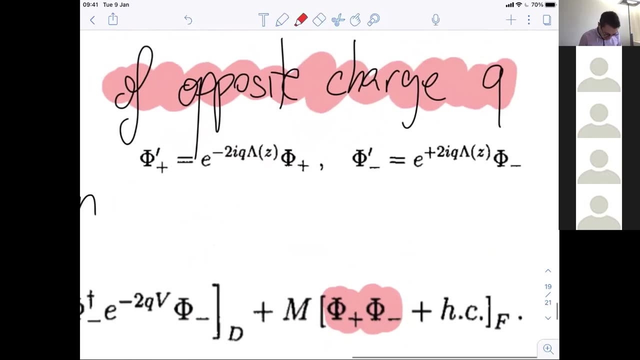 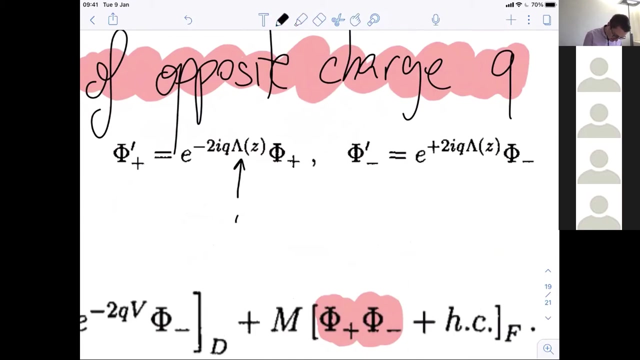 This is the SUSY invariant Lagrangian. Okay, The first term is the mass. for the electron, for instance, This is just phi plus, phi minus And this is the gauge transformation. So, remember, we are doing gauge transformation by this parameter lambda. 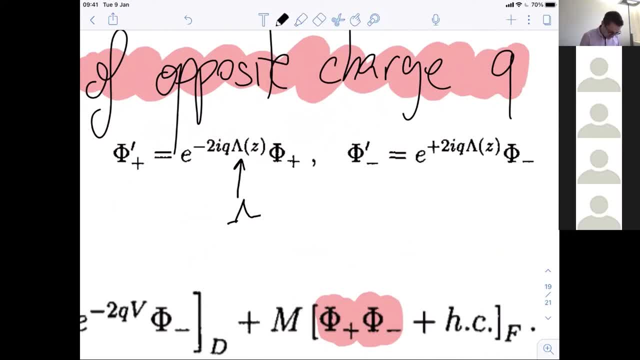 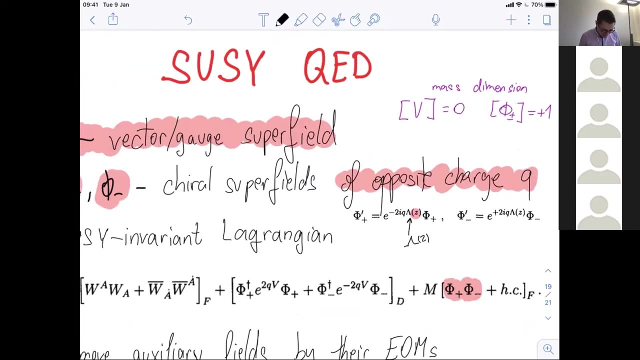 This super It's also, It depends on It's a local transformation. It depends on the, On the, On the super coordinate. Okay, Lambda depends on superco. So this term is invariant And we want to take So in our Lagrangian, we want to pick the. 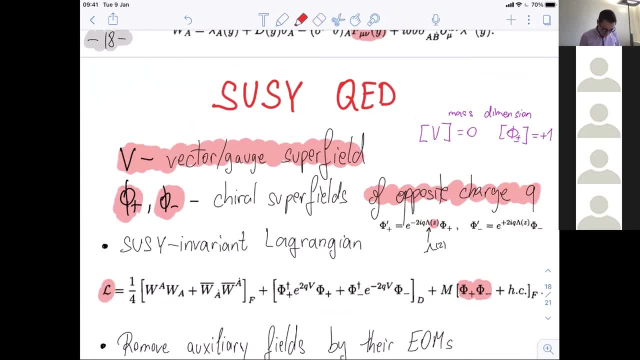 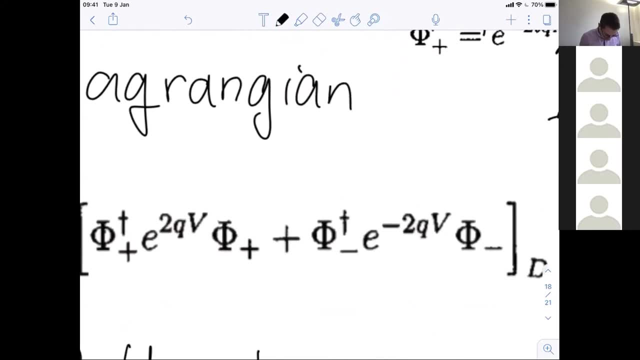 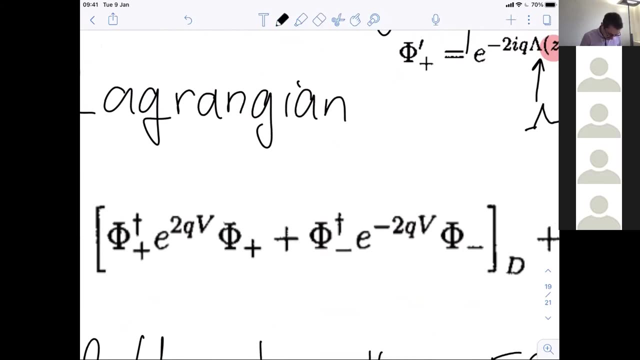 We take the F term of this. Okay, We want to have SUSY and gauge invariant, Lagrangian This term here. In order to make phi dagger, phi gauge invariant, we need to put the connection this. We have to put the vector field. 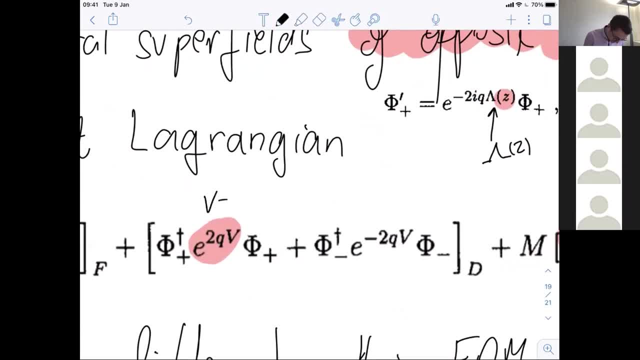 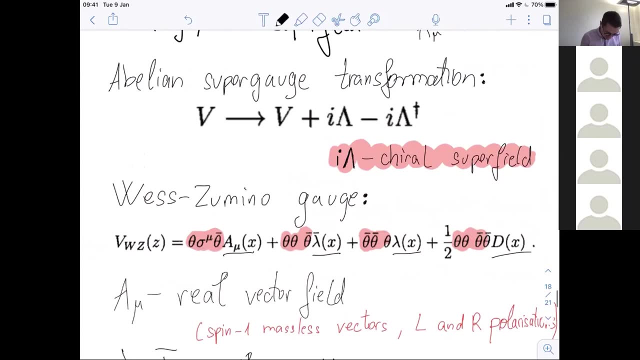 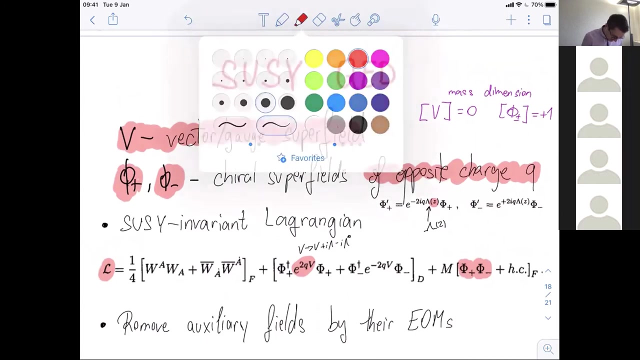 Remember, the vector field transforms in the exponent. It transforms as: V plus I, lambda, minus I lambda star. Okay, From here it's. So. that's how the vector field transforms. So it has to go in the exponent: Okay. And then, finally, this piece is just the supersymmetric analog of the. 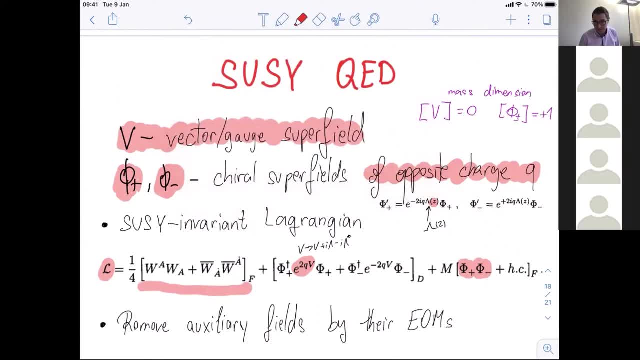 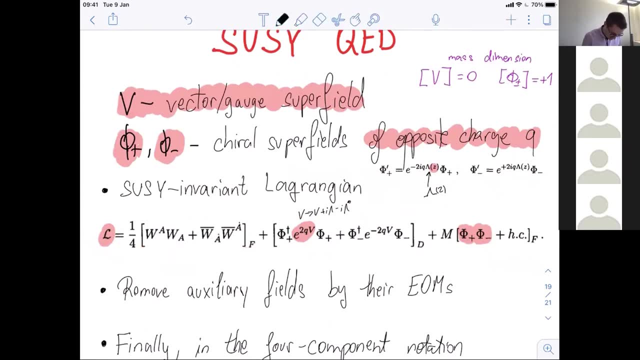 Of the gauge, Of the kinetic term for the gauge field. Sorry, let me ask just one question. Yes, please go ahead. So in this second term, in the middle, where you have phi dagger plus Yes, And then you: 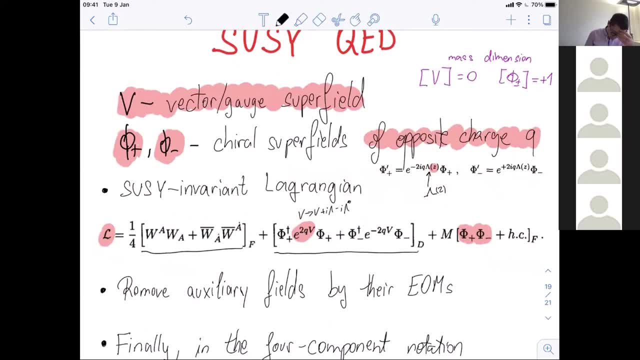 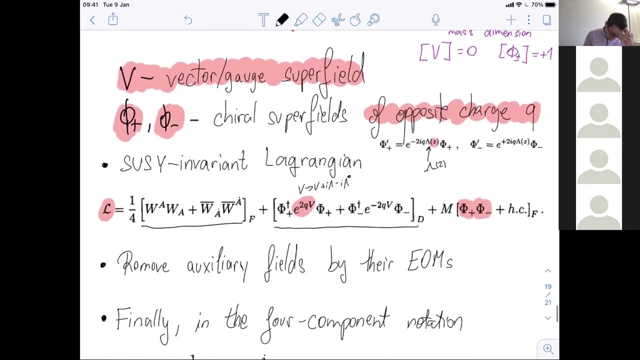 So the vector field is in the exponent. but how would we practically calculate anything? Would we have to- I don't know- take this into a series expansion and then get I don't know a lot of interaction terms, or So the point is that you have these Grassmann variables. 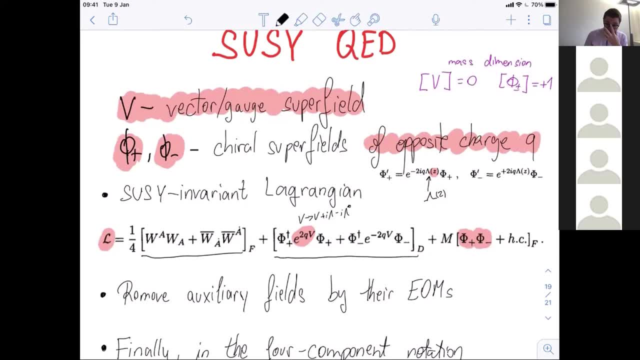 and the expansion would stop. Ah yeah, exactly, exactly. And in fact you will have only, You will have only renormalizable terms up to dimension four. Yeah, yeah, So the mass dimension of this vector super field is actually zero. 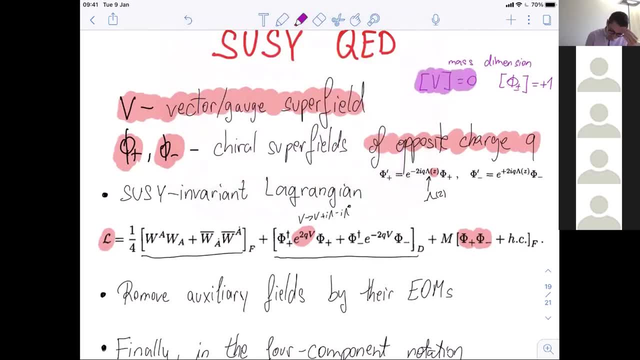 This is why it can be exponentiated. You know the canonical dimension, you can look into the details, but the canonical dimension of the vector super field is zero, Right? so you can say: are there any non-renormalizable interactions? 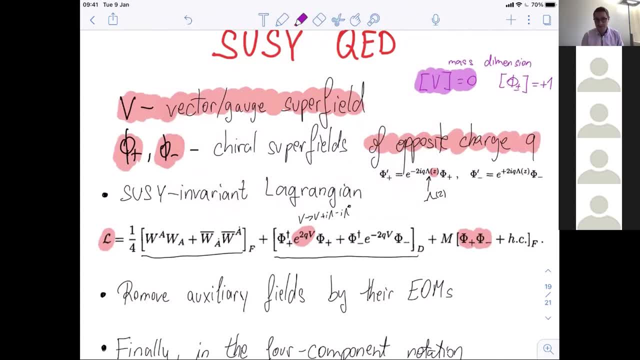 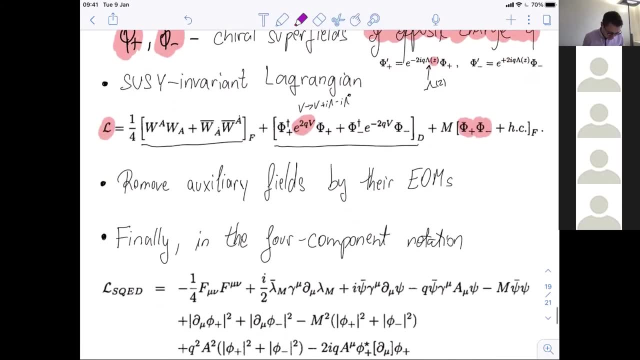 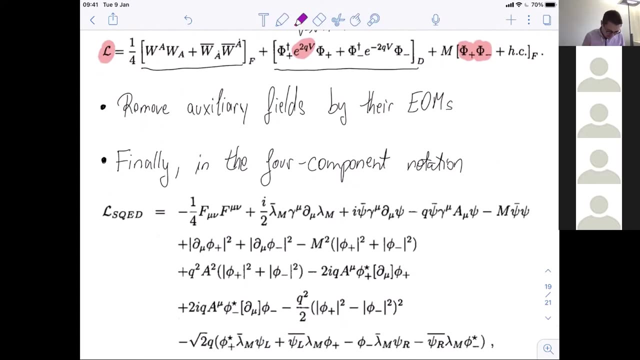 When I do component-wise, will I generate dimension five, dimension six terms? You can convince yourself that the answer is no. Yeah, exactly, Okay, okay, thank you. So you can remove the auxiliary fields by the equations of motion. So first we will remove those F and D guys and then you can expand that Lagrangian. 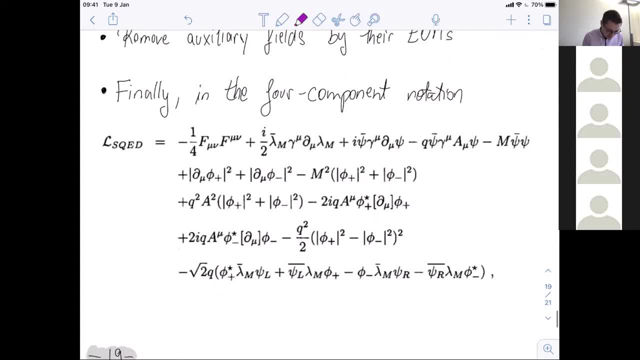 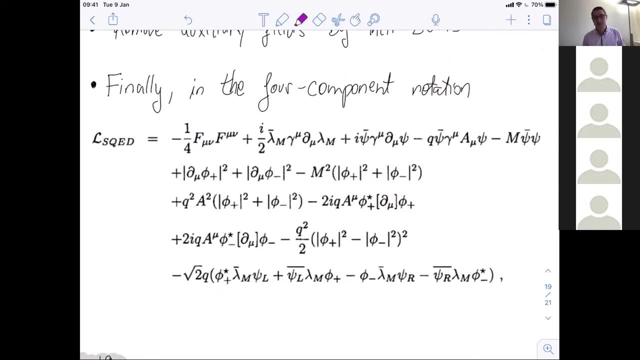 So this is Susie and Gage invariant Lagrangian, and this is what you get. This is the Lagrangian of the, The scale of the supersymmetric quantum electrodynamics, And so let's say that, if you did not pay attention to this mathematics so far, 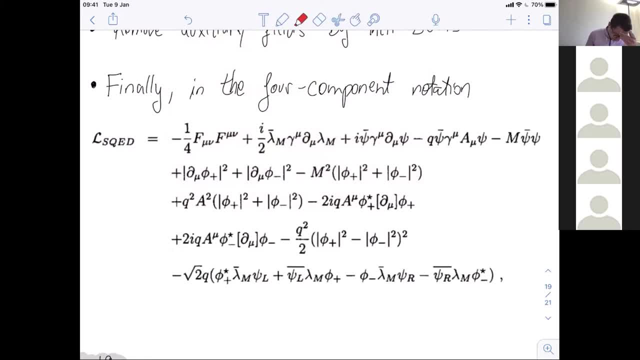 maybe at this point you should start paying attention, Because at this point I will just talk ordinary non-Susie language. So let's see what we have in this Lagrangian. I will go term by term. This thing is the kinetic term for the gauge field. 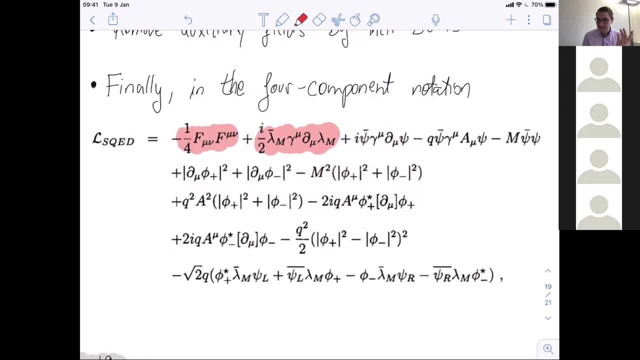 is the kinetic term for the superpartner of the gauge field, which we've called gauge genome. It's a Majorana fermion. This is the usual fermion. This is electron. This is the interaction of the electron with the photon. the usual one form QED. This is the mass of. 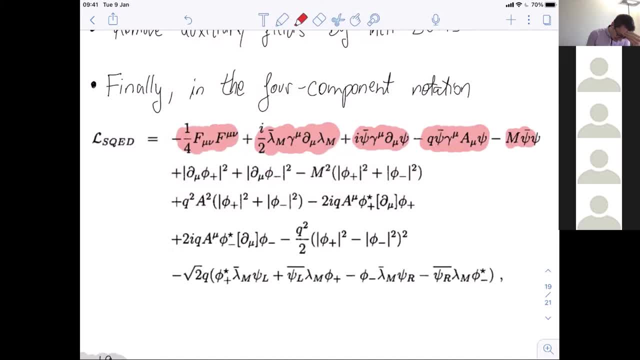 the electron. This is the kinetic term for the electron partner, selectron, supersymmetric partner. the scalar guys. We have two of them because we have two chiral fields. There are two complex scalars. Notice their mass term. They have the same mass as the electron. 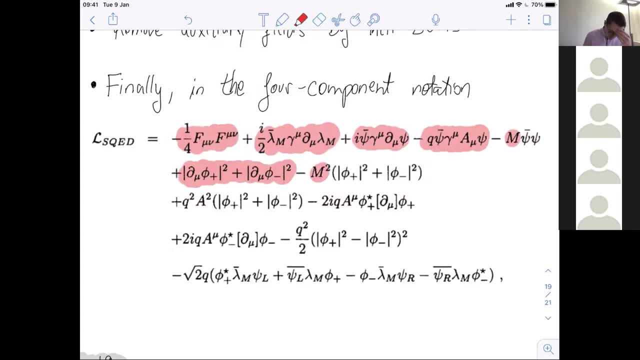 Remember they are in the same multiplet. Notice that there is no mass term for the photon and fotino Gauge. genome is in this case fotino, So they are both massless. Photon and fotino are massless, while electron and selectrons are massive and have the same mass m. 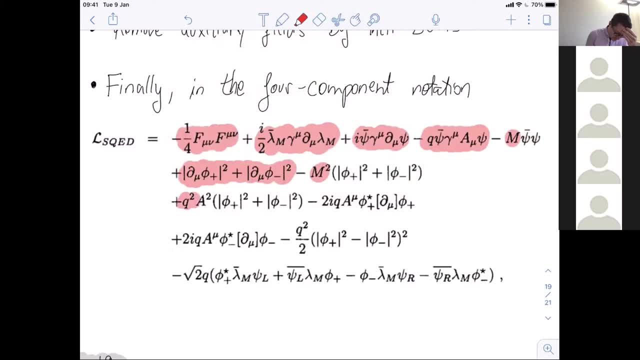 Okay, then let's move on. Now we go through the scalar QED. Remember, the scalar is the scalar Interacting with the photon. Remember, scalar QED has quartic and triple interaction with the derivative. So these three are scalar QED. Now we have the, we have, we come to the scalar. 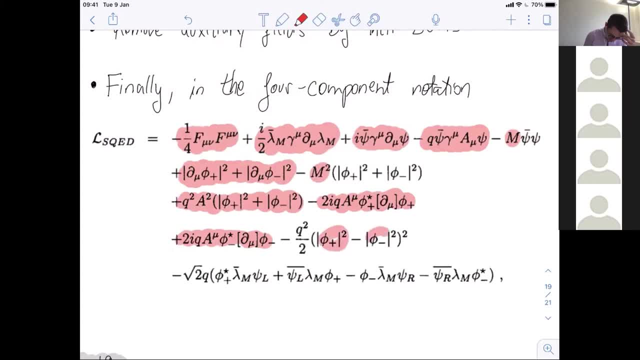 quartics. This is, this is: this is scalar quartics. These are things of this type. no, What is really funny here is that the quartic coupling is related to the gauge coupling. This is what supersymmetry does. So these are quartic couplings between, between scalars And the final. 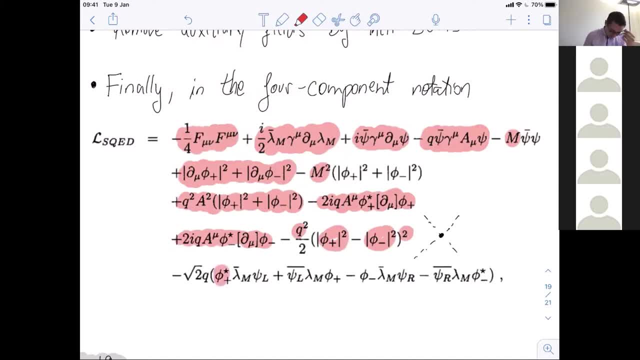 row is the interaction between the scalar selectron with the, with the, with the, with electron and gauge genome. Okay, So this is. this is selectron-fotino-electron coupling. This is peculiar to, to, to supersymmetry. 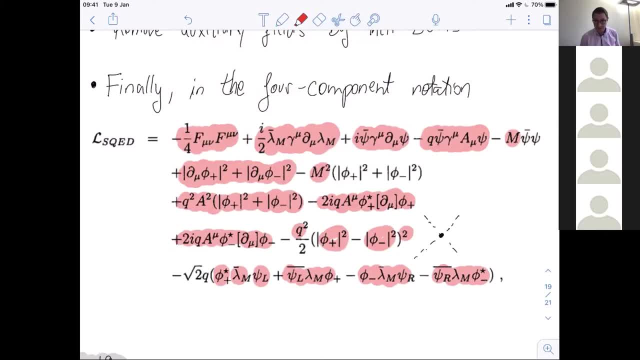 which supersymmetry gives you this Fotino-electron-selectron coupling And this in ordinary, in ordinary theory, this kind of interactions you would call Yukawa interactions. So this is a scalar And this is a fermion, and this is also a fermion. So this is, this is just Yukawa interactions. 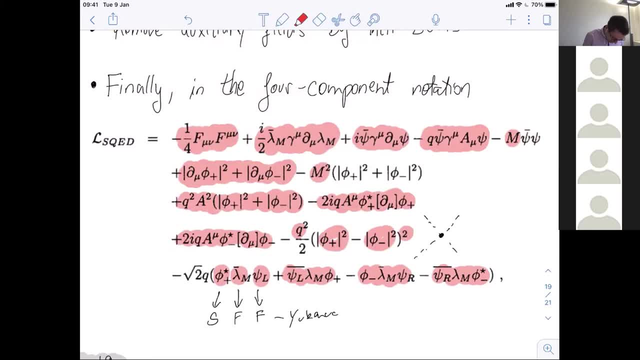 And notice. another thing is that Yukawa interactions are also given by the charge Q. Let me clear all of this. And if I were to ask you the following, Okay, Okay, I will give you the fermionic field, I will give you scalar fields and I will tell you. please write down the. there is a U1 gauge symmetry. there is a charge Q. the charge is the same for this two complex scalar and for the Dirac fermion. 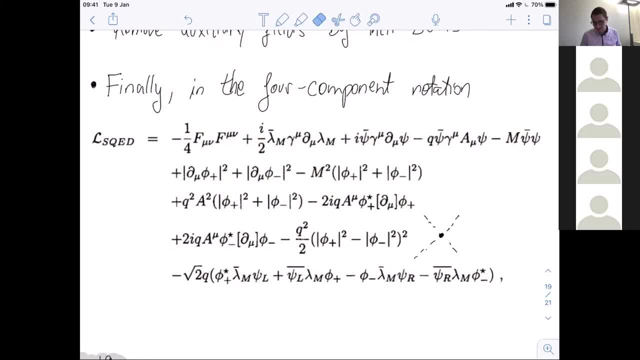 and could you please write down all the interactions which are renormalizable, consistent with the Poincare and the gauge symmetry. You would write down many terms. for example, you would write down these quartic interactions and this quartic coupling will be completely independent of the charge. 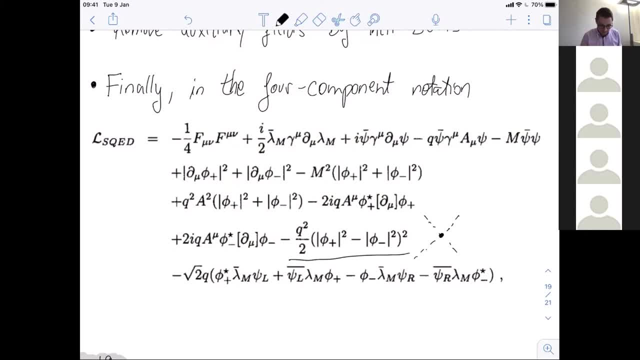 It will be just some new input parameter in your theory, like the quartic in the standard model is just okay. Also, Yukawa interactions: the Yukawa interactions and the quartics would be some input parameters, and also it will be. it will be different, like 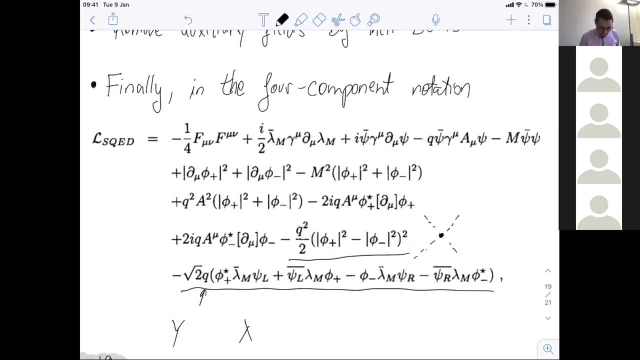 you know, each Yukawa would be independent, each quartic would be independent input parameter. Supersymmetry is a very powerful symmetry. It tells you- you see this example of supersymmetric QED. it connects the gauge coupling. it connects the Yukawa and the quartics to the gauge coupling. tells you, it dictates: you know the. it's very powerful symmetry which gives you additional relations between the couplings. 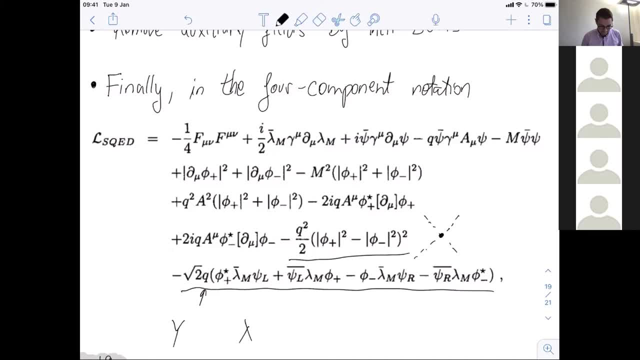 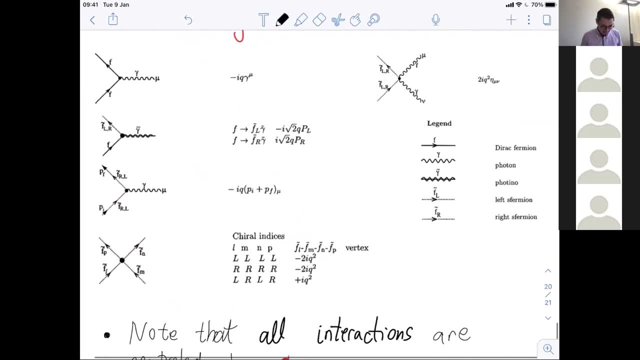 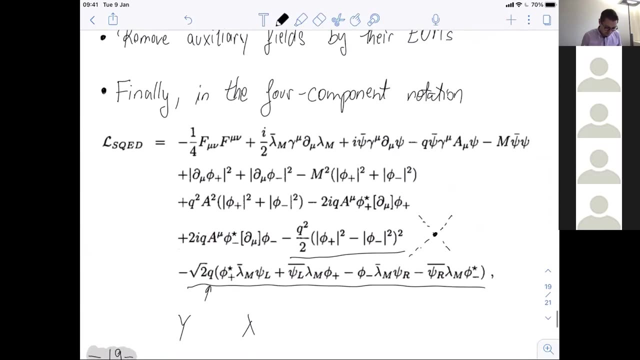 I hope that this point is clear. This is actually what will be crucial to the higher problem. All right, and then you can have a look at the different super QED Feynman rules. Do you have any questions about this point? I think this point is crucial. 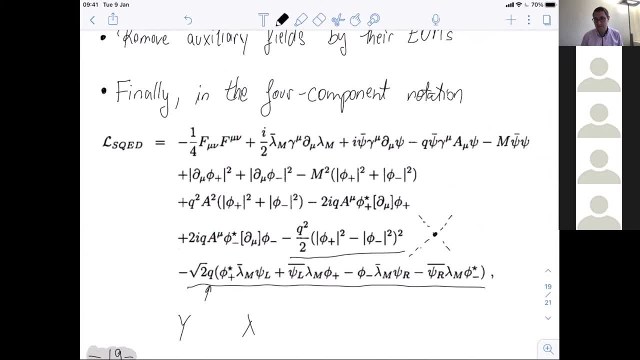 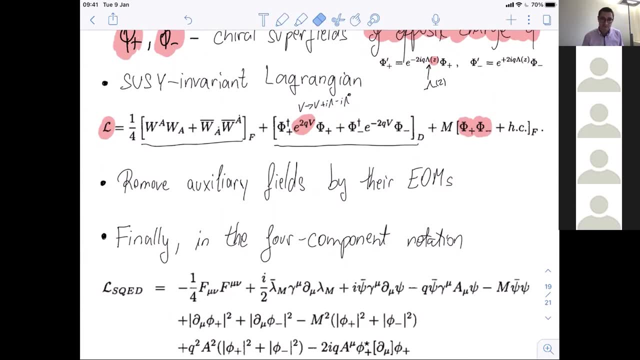 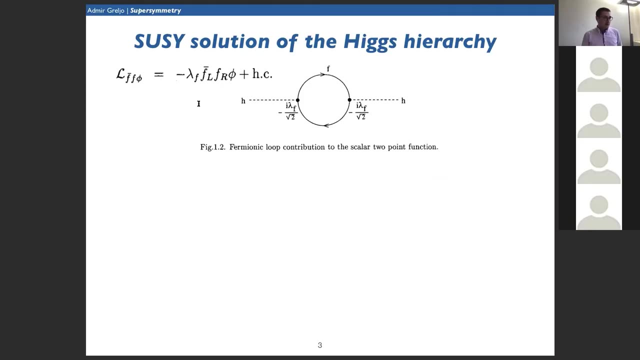 How supersymmetry connects different terms in the Lagrangian. Okay, I will stop sharing this one and go to the other one. Okay, so remember the Higgs hierarchy problem. For example, the correction to the Higgs self-energy for coming from the top quark were quadratically sensitive, quadratically to the new physics scale, okay, and we had this interaction between the Higgs and then the quark. there is this lambda F which is the Yukawa coupling. 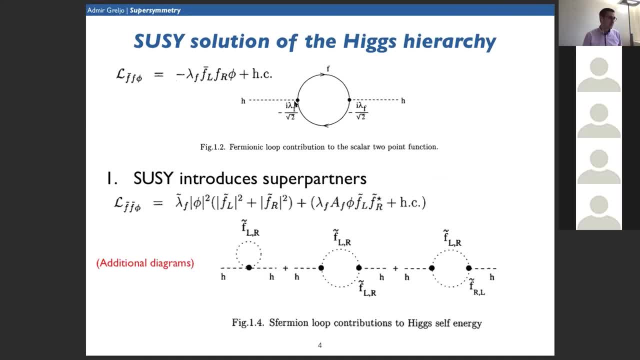 So how does supersymmetry solve this problem? So, first of all, supersymmetry introduces super partners. So in addition to the Fermion F- okay, that couples to the Higgs- there will be Sfermion, its super partner, which is spin zero. okay. 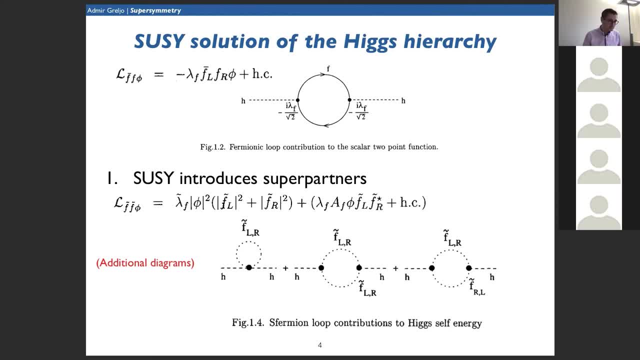 the chiral super multiplet, which will also talk to the Higgs with some coupling. So this is the this lambda F tilde. I will come to the relation between lambda F and lambda F tilde. And we know that supersymmetry is broken. 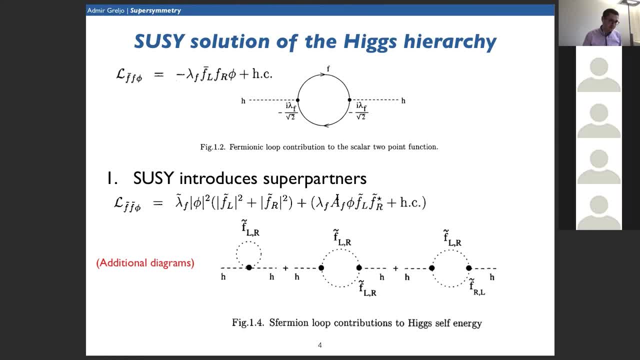 So there will be this piece here. can you see me pointing the second term? This A F, Okay, This A F. this actually breaks supersymmetr. the first term, president is comes from the supersymmetry presenting the second one is breaking. 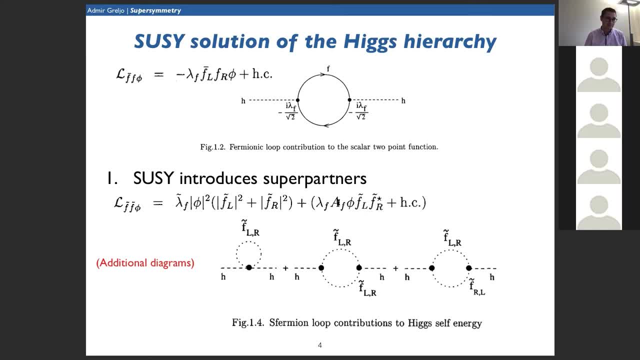 And this one will give a mass to the, to the super partner. This is called the soft breaking because it goes with the relevant operator. Relevant meaning is meaning that dimension less than four. So in fact this is dimension three, because this is scalar, scalar, scalar. 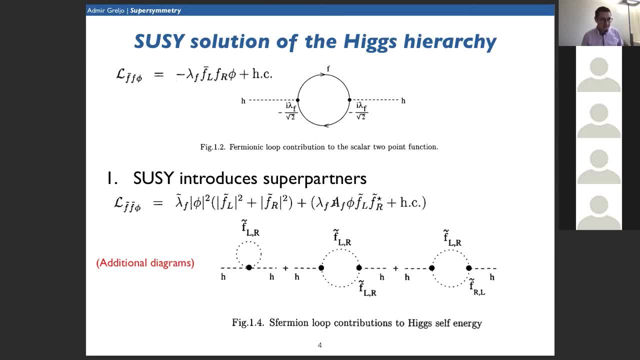 This is the A has mass dimension one. okay, So the point is that at very high energies these operators will not be so important, but at very low energies they are relevant. okay, This is called soft breaking. In any ways, what do we do? 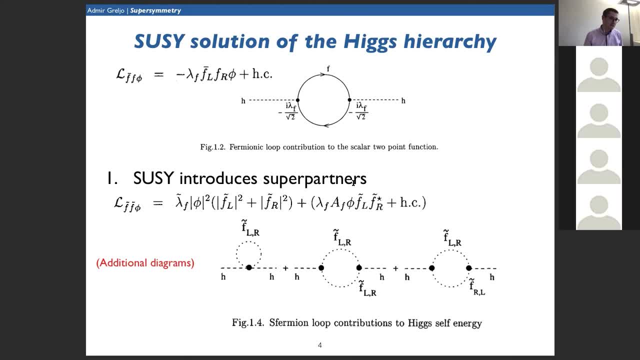 So we have to call it. we have additional diagrams because supersymmetry introduced additional particles. These are the additional contributions to the Higgs self-energy. Now you take, you have to include them, all of these contributions to the self-energy of the Higgs. 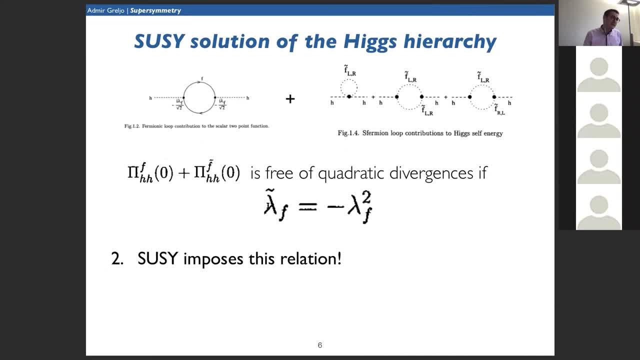 And notice what happens is that if Lambda F- tilde coupling to fermions- is minus Lambda F squared, then the sum is free of quadratic divergences And supersymmetry imposes this relation, exactly this relation. Remember the QED, Susie QED example where quartic 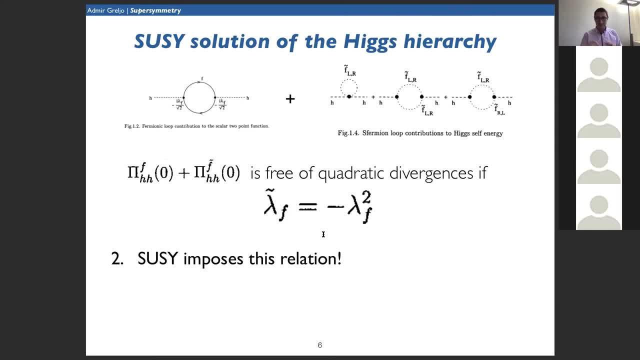 and the Yukawa was connected to the gauge coupling, So all the couplings were connected with the same parameter. The supersymmetry imposes the connection, so that this might seem like a miracle, but if in fact it is not, you are putting in the same multiplet, super multiplet. 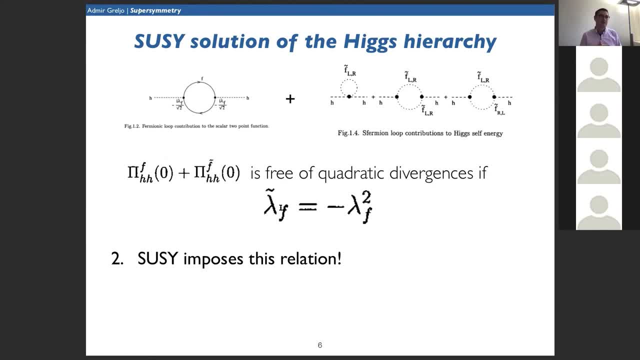 you are putting a boson and the fermion, And we know that fermionic mass is protected in the top sense from the, from these quadratic divergences And even more. if you are more interested in this, even more deeper is. the explanation goes under the name of: 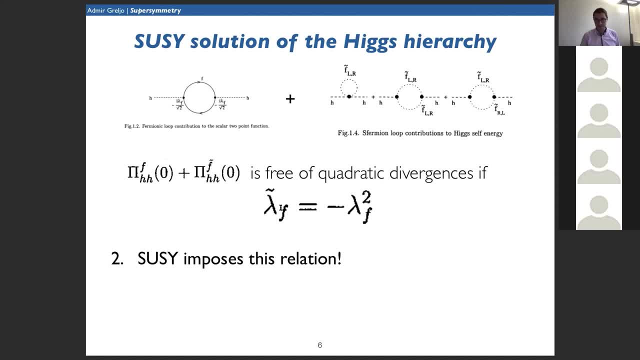 the Newtonian equation And it will be used to calculate the non-renormalization theorem in supersymmetry. It's a very nice subject that one can. one should have a look, But this is in simple terms. this is how the Susie solves the problem. 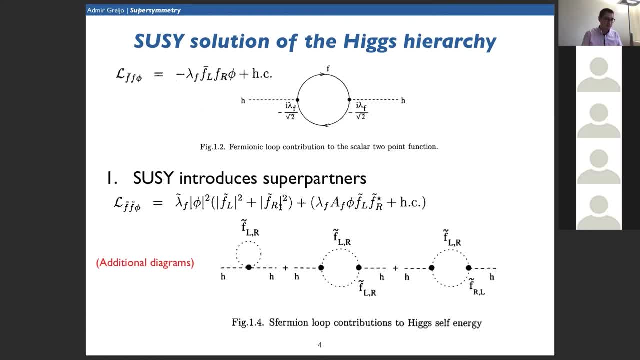 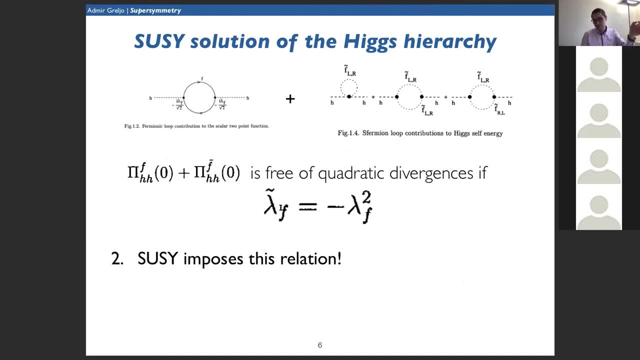 First, it introduces new partners. So there are new, new diagrams. And not only that: it relates the couplings between Higgs with the top and Higgs with stop in precisely such a way to cancel the top, the quadratic divergence in the loop. okay, that's how it works. another tiny detail is that the, the 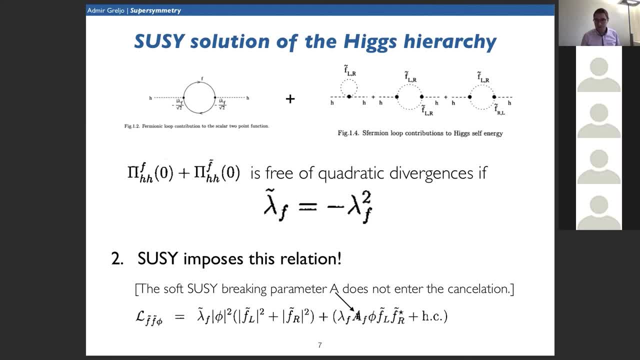 soft SUSY breaking. parameter a, which was there to give the mass to the Spermion, does not enter the cancellation, so that the cancellation of quadratic divergence doesn't depend on that, on that that parameter. so this means that. so you, you are solving the hierarchy problem above the 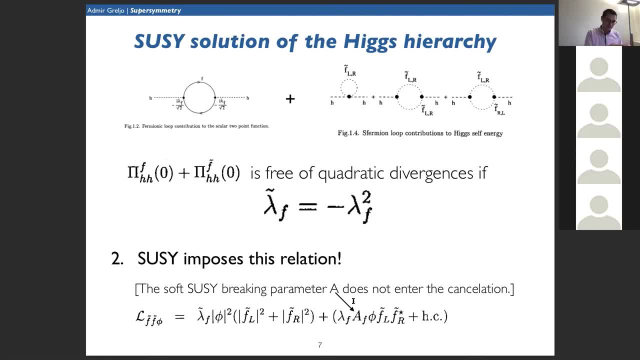 mass of this guy, so above its mass of this super Spermion. the loops between particles, anti-particles, would cancel out the quadratic divergence. so from that scale on, your theory is is safe. you don't have a hierarchy problem. the only hierarchy that you have to think about is: 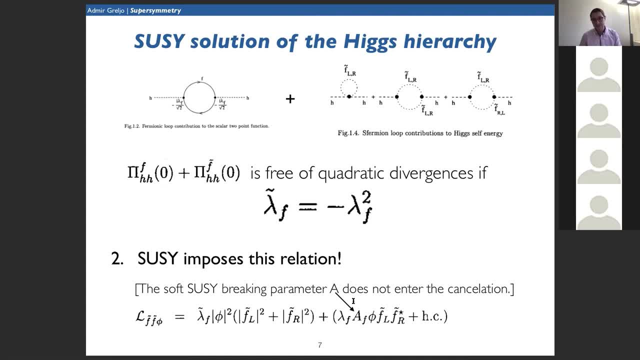 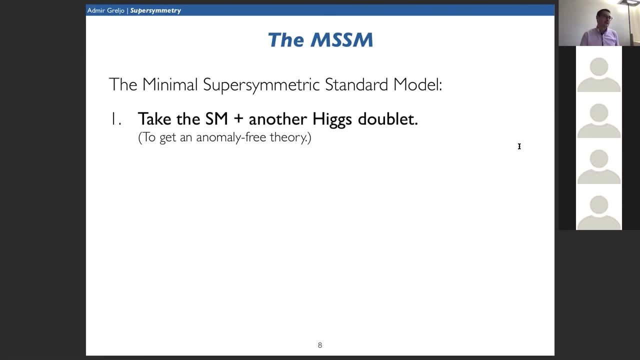 the little hierarchy between the Higgs and supersymmetric partner, the mass of this Spermion. okay, so what is the MSSM, the minimal supersymmetric standard model? so what do you do? you take the standard model. you have to add another Higgs doublet. the reason is that when you promote the, the fields to super fields, 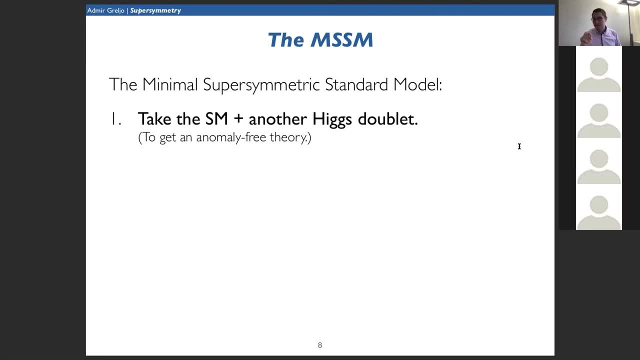 when you supersymmetrize your theory. the Higgs is a scalar, it will. it's in the, it will be part of the chiral super multiplet. so it will, it will have. there will be additional chiral Spermion, Higgs, Sino, okay, and you will have gauge anomaly because you start from the anomaly free theory. you will. 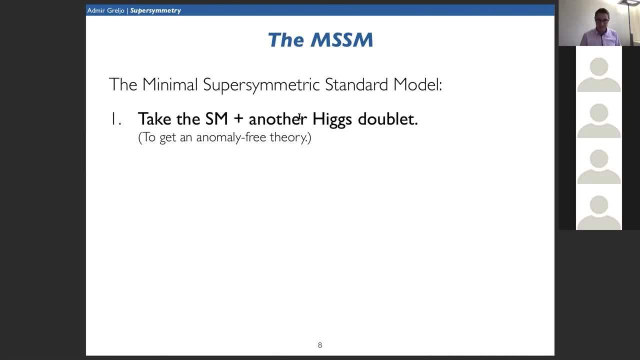 get. so you have to introduce another Higgs doublet with opposite gauge charge in order to have a anomaly free theory. so in fact, you start with the two Higgs doublet, you have to introduce the two Higgs doublet model, standard model, plus another Higgs, then you supersymmetrize. 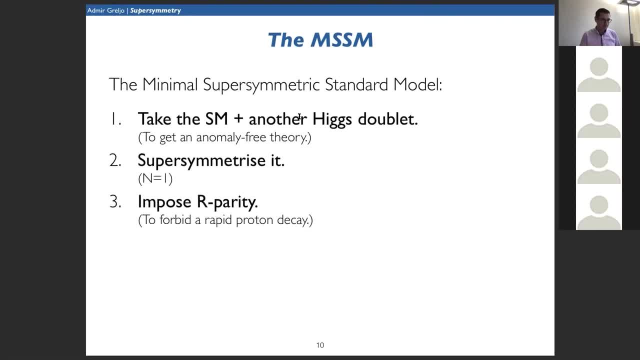 it in a minimal way and equal one supersymmetry. then you impose the R parity, this discrete Z2 parity, otherwise you would have problems with proton decays. and then you need to break supersymmetry. from phenomenological reasons we haven't observed it. then you 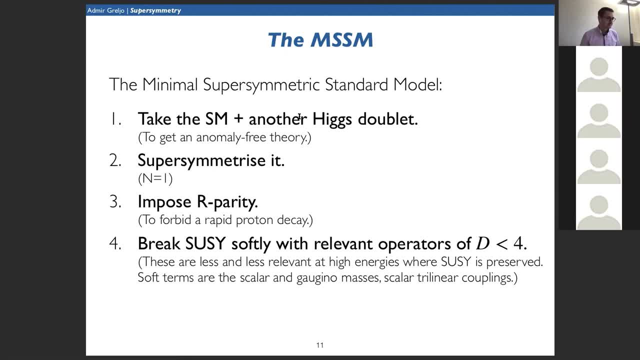 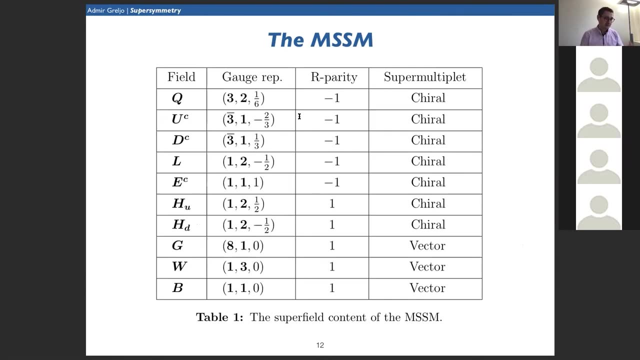 break the supersymmetry with in a soft way, meaning you only put scalar masses or gaugino masses or the scalar trilinear couplings, and this is MSSM. the MSSM has this is the chiral, the superfield content. so in the chiral 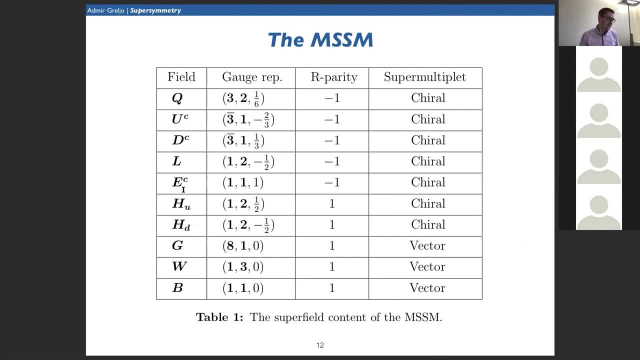 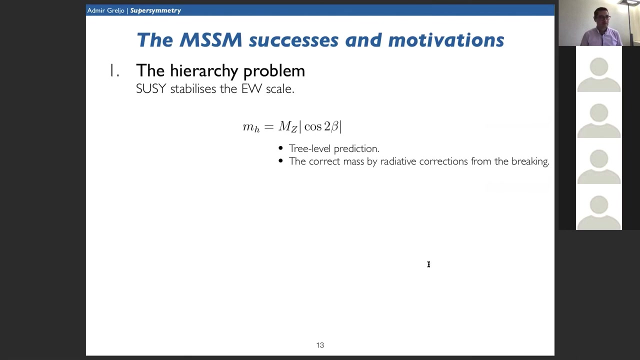 superfields are the usual QUDLE: the fermionic guys and the two Higgs's. note that they, the two Higgs's, have a different U and charge and the gauge fields are put in a vector, in a vector supermultiplet. okay, so the MSSM is really the benchmark for. 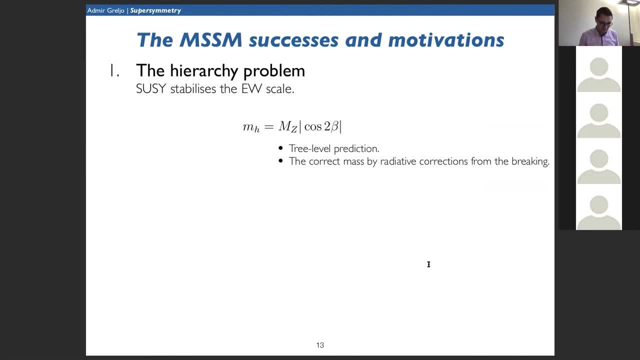 beyond the standard model physics for many, many years. you know people consider this, as you know, the most important benchmark theory beyond the standard model and has some really fantastic features. for example, it solves the hierarchy problem. this r parity, which was needed to protect proton decay. it gives you automatically a candidate. 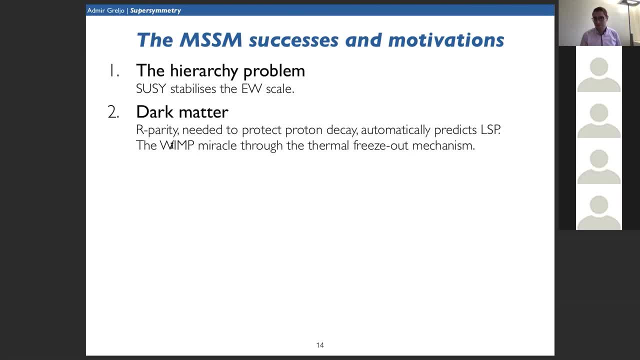 for dark matter and in fact you can realize the WIMP miracle: weakly interacting massive particle through thermal freeze out mechanism. it is the vanilla, you know, dark matter that we can think of. then you can sort of fairly generically get electroweak symmetry breaking that we. 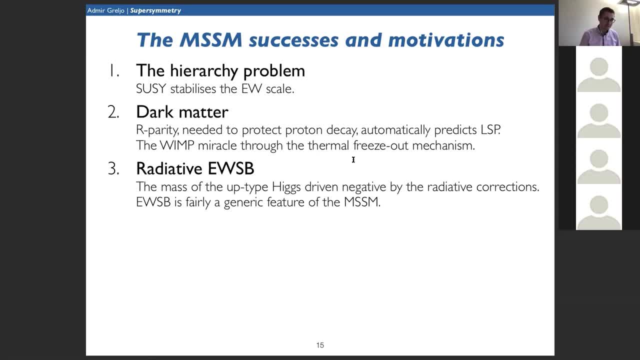 observe by radiating corrections which drive the mass of the up type Higgs to the negative value. so you could even have a rationale for the electroweak symmetry breaking. then you can do baryogenesis. you can explain the the matter. anti-matter asymmetry, MSSM can. 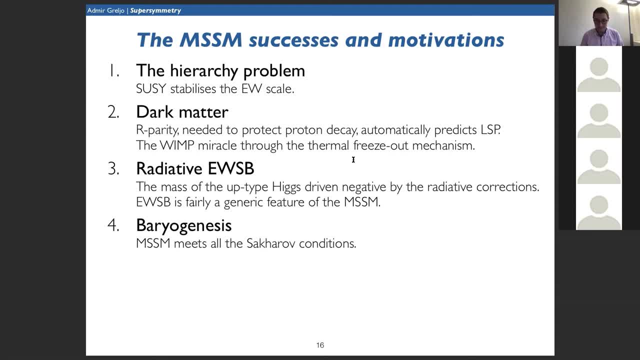 meet the Sakharov conditions, unlike the standard model. uh, unfortunately you can see that the energy is very low. so you cannot do any much about the flavor puzzle. but you don't. you typically don't have the new physics flavor problem, for example, if you have a. 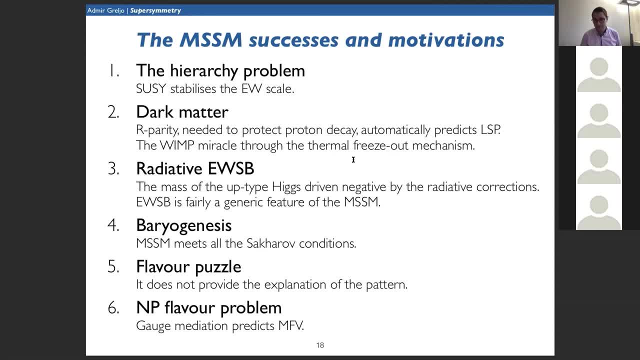 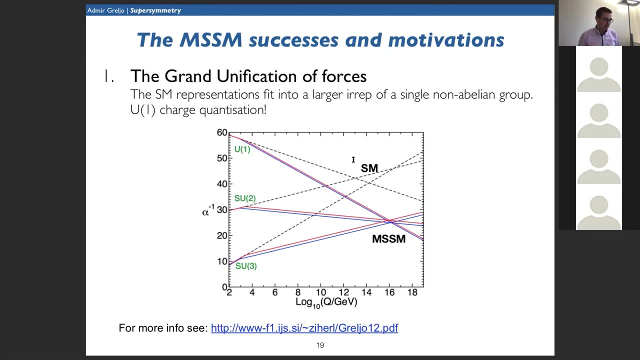 specific type of SUSY breaking, called gauge mediation, you. it predicts minimal flavor violation for energies, meaning that you can have states close to the tv scale and not induce large flavor changing neutral currents. finally, what i really like about supersymmetry is the following: it is the, the, the grand unification of 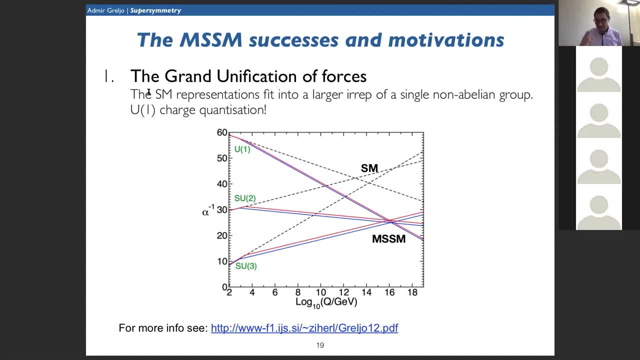 forces. so in the standard model we have this u1 charge, which is just a phase, and um. we see from from from experiments that these are some rational numbers. for example, proton has the same as an opposite charge as the electron, and this to many people, this, this uh. 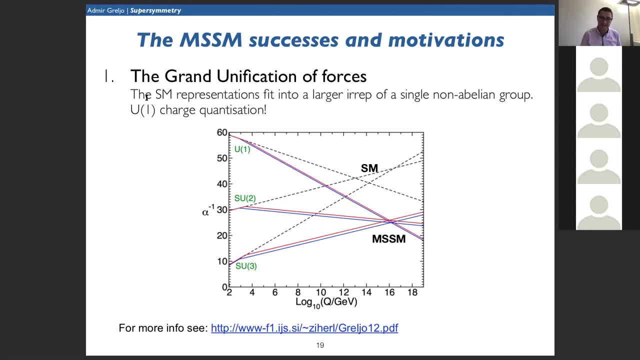 consistency of gauge anomaly cancellation is actually a hint that we can put the, the, the, the particles, the, the, the standard model representations into a larger irreducible representation of a single non-nobelian gauge group. so there would not be a three groups like su3, su2, u1. 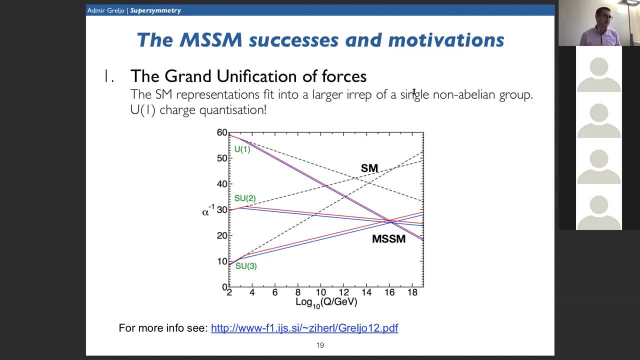 but one big, grand unified uh group. so the gauge couplings, if you go to very high energies, if you run up, they would eventually eventually merge into a single coupling, su5, for example, um and in the standard model, if you do the running with the standard model. 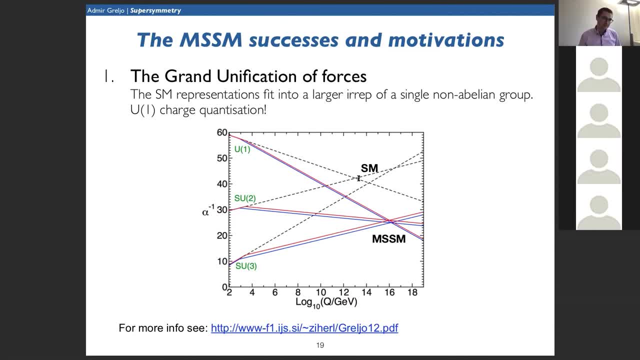 field content. you would miss that. they don't. uh, okay, but in the mssm they just mssm, they miracle low scale mssm around the tv they um, unify to the gauge, couplings unify. there is a hint for unification from the uh. 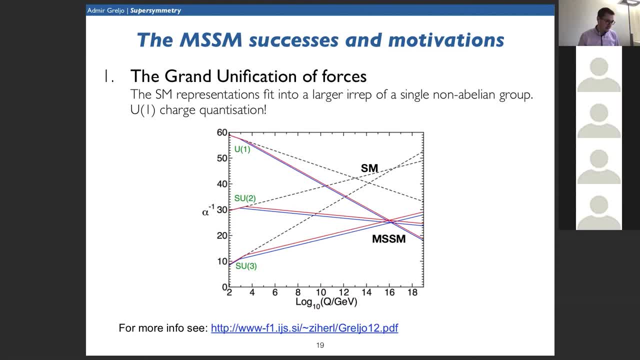 from from the mssn and uh. i was really fascinated about this subject during my phd and this is a link to to my uh homework from 2012 on the subject of grand unification. so mssm really has many nice features. other motivations for supersymmetry: 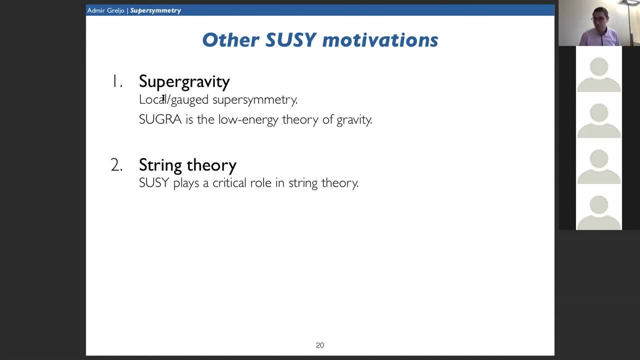 would be super gravity. if you, supersymmetry is a global transformation. remember that epsilon did not depend on the, not depend on x, but if you, you can gauge it. if you gauge it, you get something which is called sugra and it's a low energy theory of. 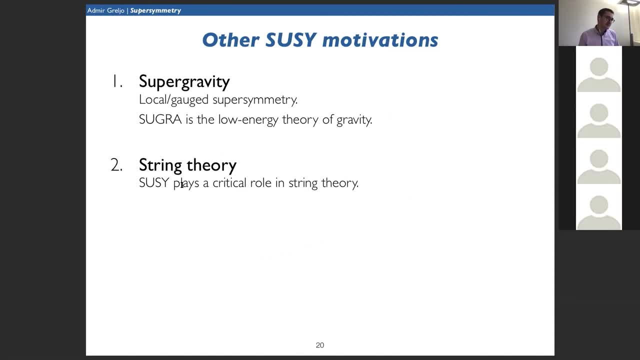 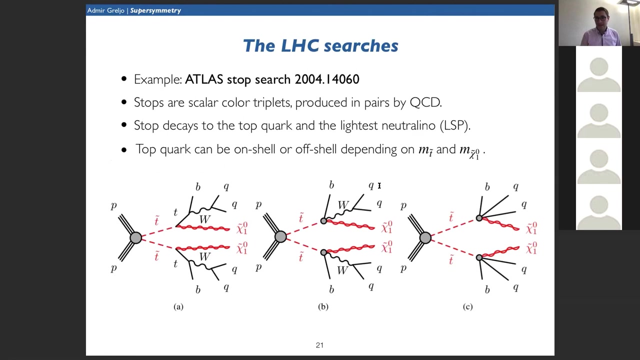 gravity and also supersymmetry plays a critical role in string theory. it's in basis of uh and string theory is one of the most celebrated framework to to go to the quantized gravity. so supersymmetry is all over the the place and clearly it was the prime target for.